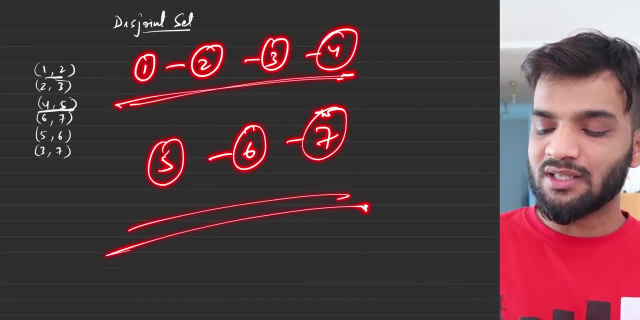 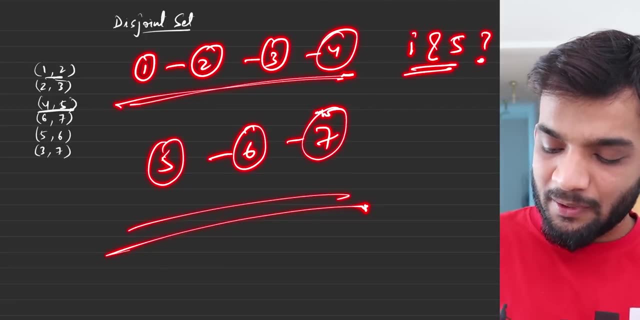 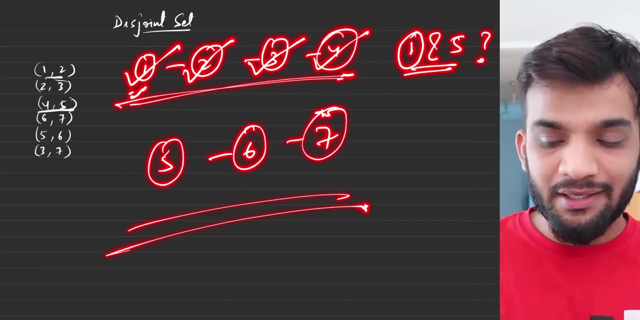 this Second one is this. Now, suddenly, someone will come up and say: hey, does 1 and 5, belong to the same component or not? How will you determine? You'll pick up 1 and you'll start a DFS traversal: 1,, 2,, 3,, 4.. And the traversal is complete. You could not find 5.. Since you could, 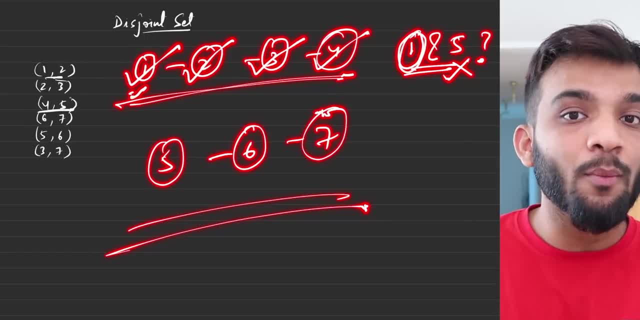 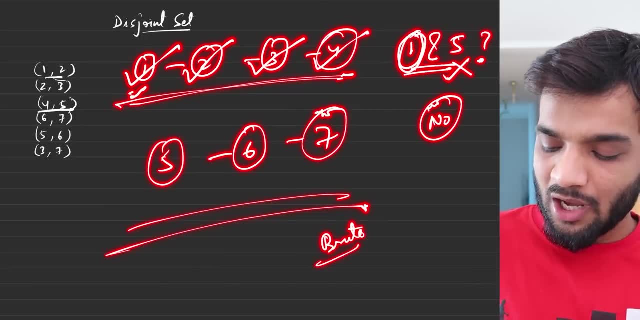 not find 5 in the DFS traversal of 1 in that component, you'll be like they do not belong to the same component. You did a DFS traversal and that's the brute force. How much time will the DFS traversal take? N plus E, That's the complexity of the DFS or the BFS And you'll 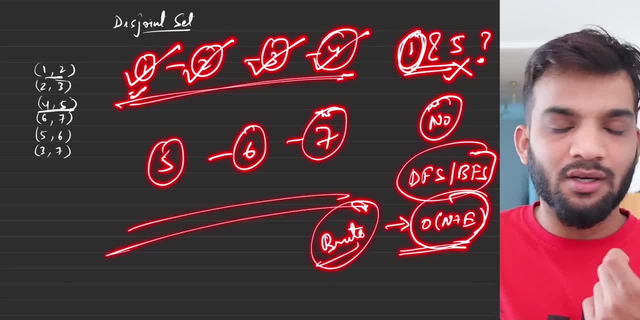 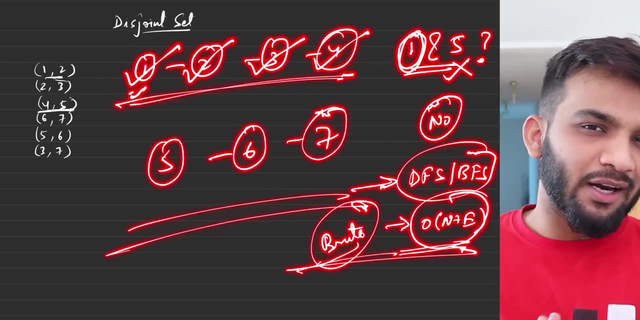 be like: how much time will this take? Already discussed this in the previous section of the graph series. If you do not know DFS or BFS, go back and watch it. So the brute force is going to take a kind of linear time complexity. So this is where something like disjoint set comes in and 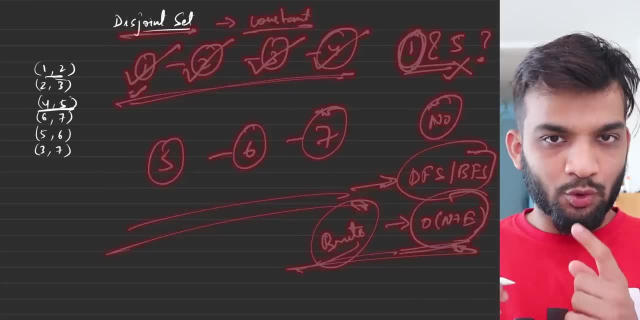 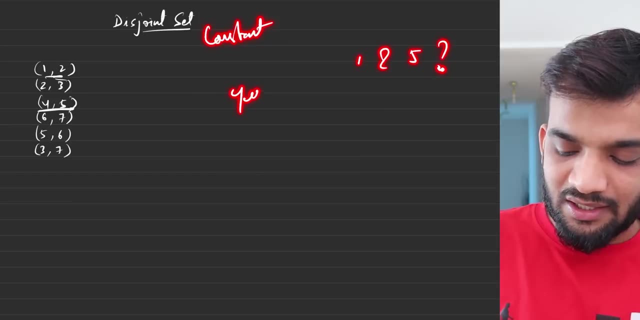 says: hey, I'm going to do the same thing in constant time. You ask me: does 1 and 5 belong to the same component? I'm going to tell you in constant time either a yes or a no. That's the. 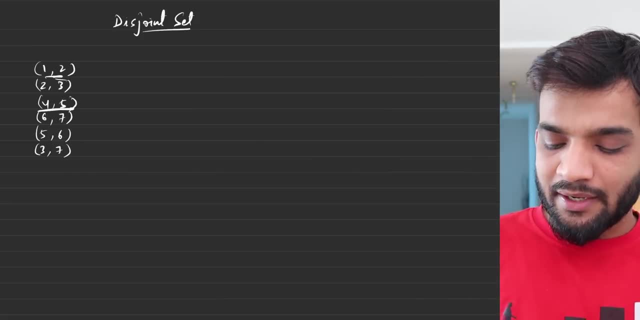 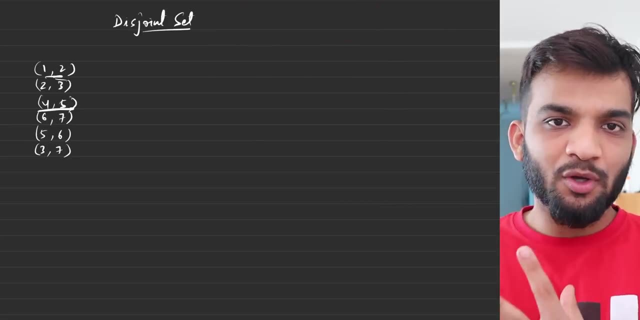 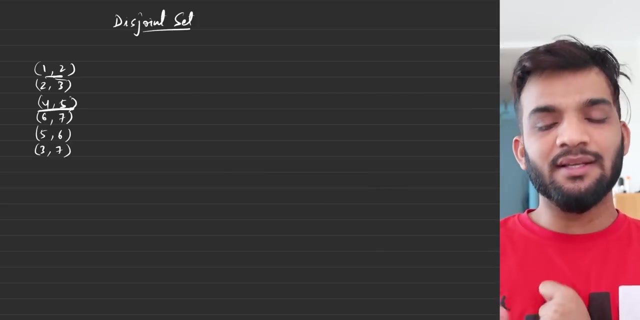 idea of disjoint set data structure. And one more thing: it is usually used in dynamic graphs, graphs which keep on changing, graphs which keep on changing their configuration at every moment. What do you mean by exactly changing configuration? I'll explain you that in the later part. 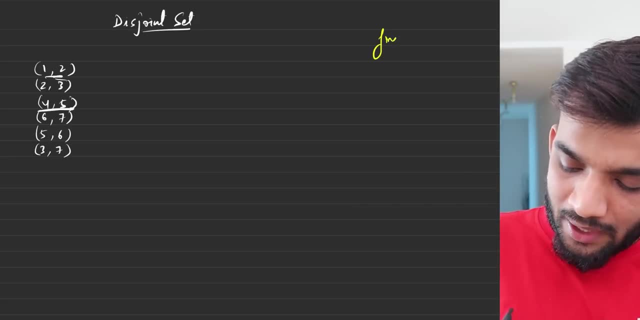 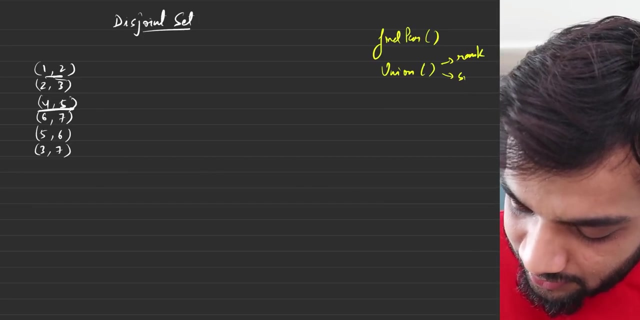 So disjoint set gives us two options. One is finding the parent, That's one of its main functionality, And the other main functionality is union. Now, union can be done with two methods. One is rank, Other one is size. I'll be discussing both of. 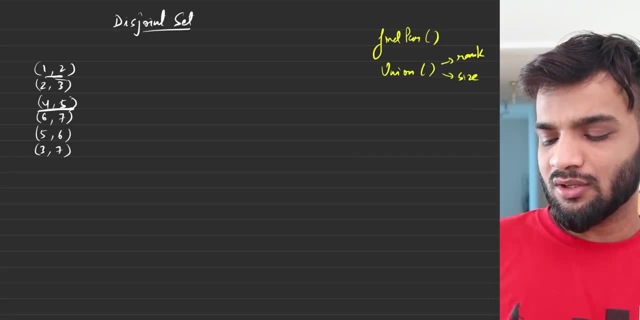 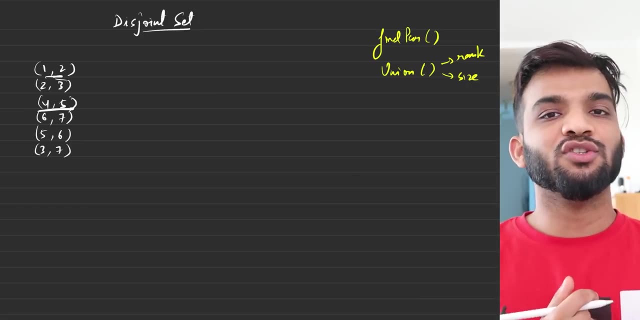 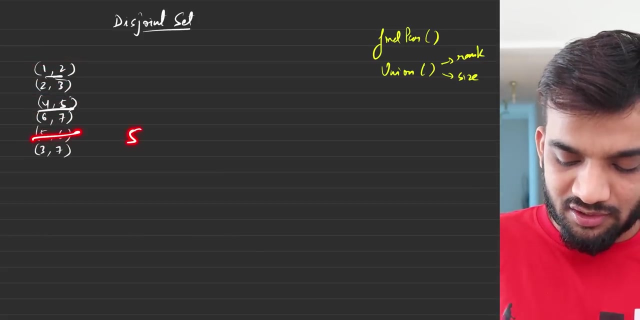 them. But so, primarily, it gives you two functions: find parent and union. Now I did talk about dynamic graphs, graphs changing configurations, So let's understand this. Now, what do you mean by these things? These are all edges. There's an edge between 5 and 6.. So, initially, what we assume. 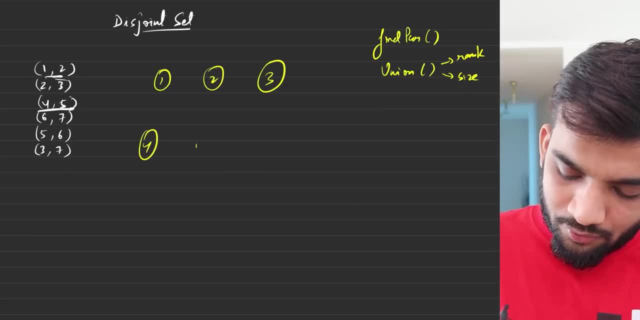 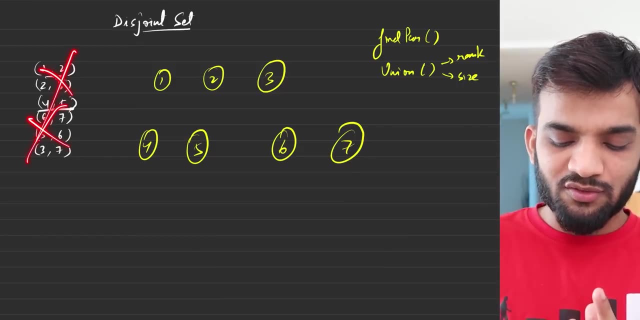 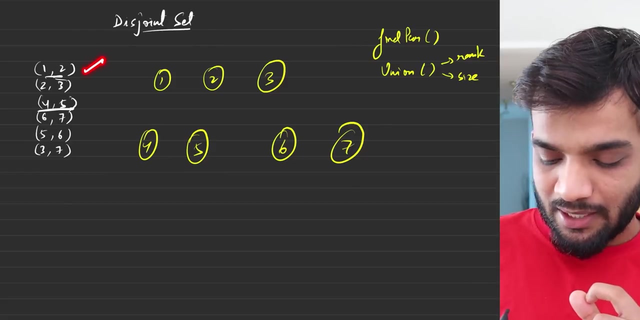 is 1,, 2,, 3,, 4,, 5,, 6, 7.. Everyone is alone. So initially, before all these edges formation, every node is single, single right. So you have 1, 2.. What it means is I'm asking you to connect. 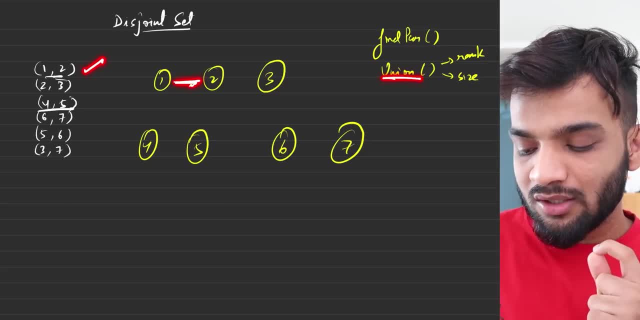 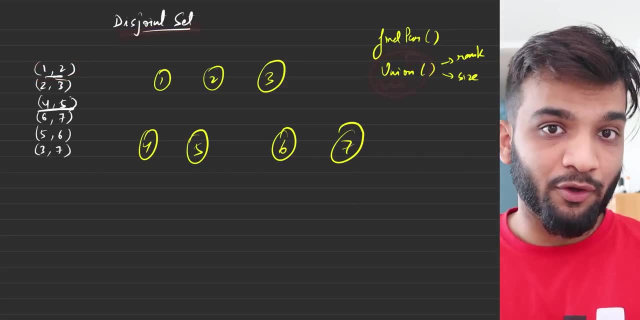 1, 2.. So that is what union does for you. Remember this: Whenever I say connect 1, 2, union in disjoint set will do it for you. We'll talk about that in a little bit. So let's get started. So let's get. 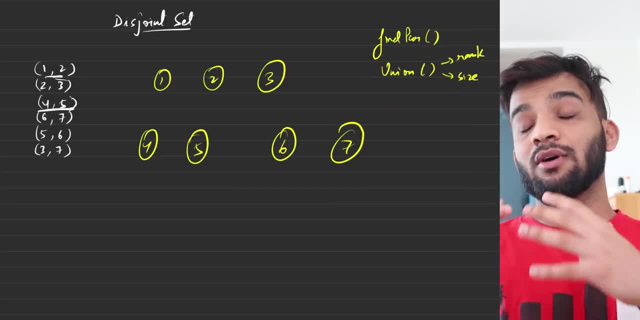 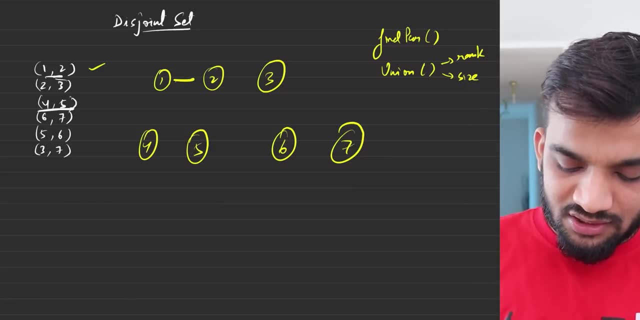 started. Let's talk about union in details. But as of now know the higher level of union Union will go and connect. So what I'll do is I'll go and connect. Okay, done. Next: 2 and 3. Connect 2. 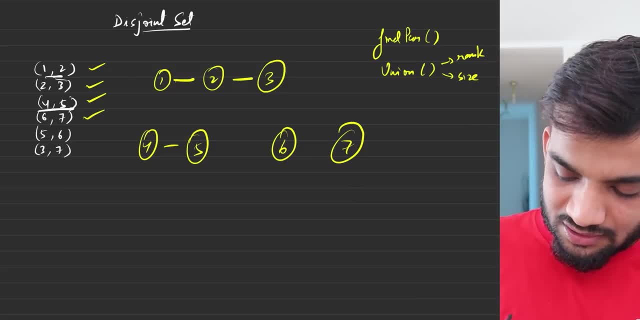 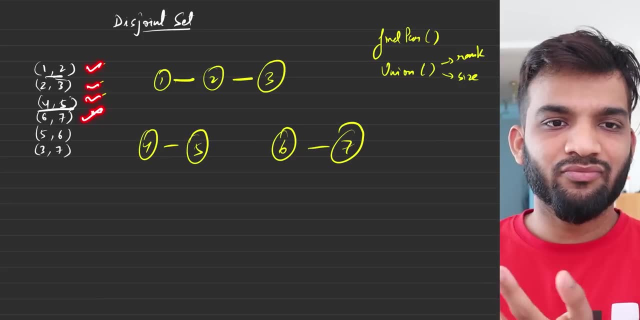 and 3.. Next 4 and 5.. Connect 4 and 5.. Next 6 and 7.. Connect 6 and 7.. So you see, the graph is changing at every instant. But you'll be like: but Shriver, wait, this is how graph is formed. 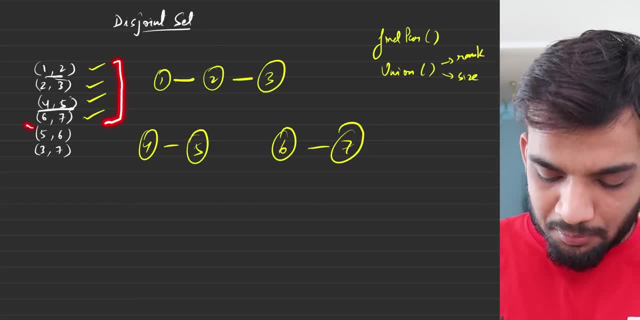 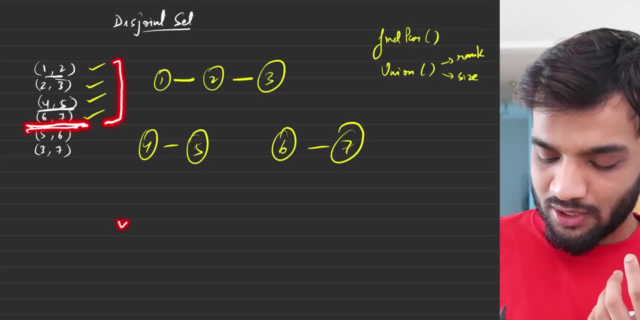 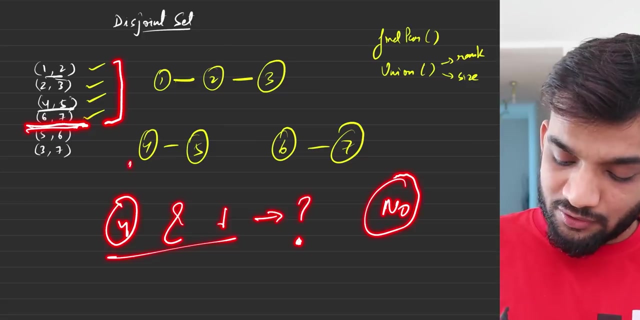 But what happens here is, if I stop the formation over here and I give you a question where, after this formation, I suddenly ask you: hey, does 4 and 1 belong to the same component or not? You will say no, Why? Because 4, as of now, is here. 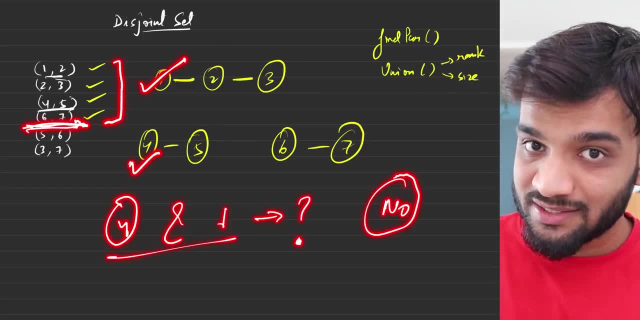 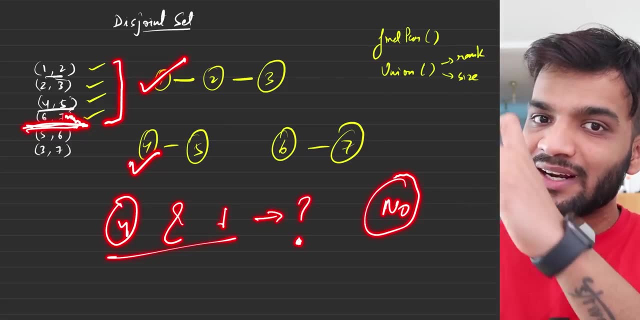 1 as of now is here. Till this point they're not in the same component, So the answer will be no. So in any stage someone might come up and ask you, because the graph is changing at every step. But I can ask you a question at any step And you should be able to. 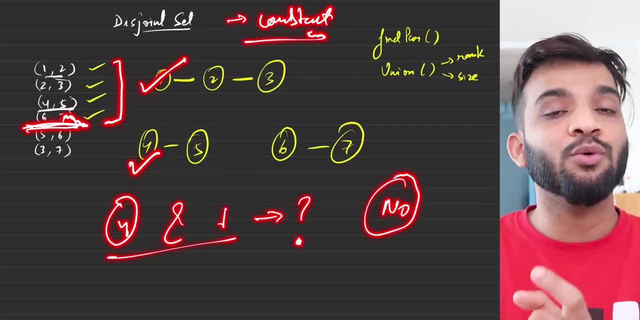 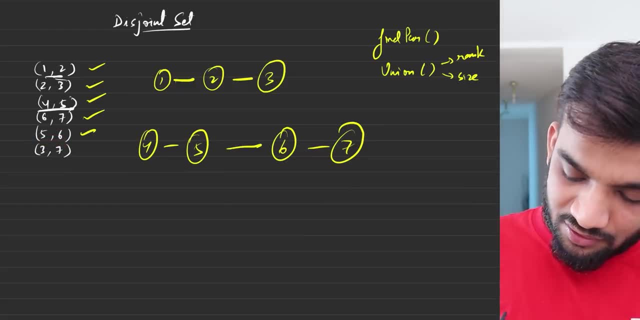 answer that in constant time. That is what this joint set will do, And I'll explain you how it does. Next, 5 and 6.. Let's connect 5 and 6.. Next, 3 and 7.. Let's connect 3 and 7.. Now, if I ask you, 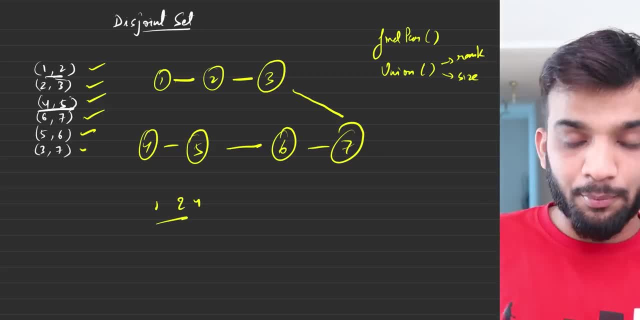 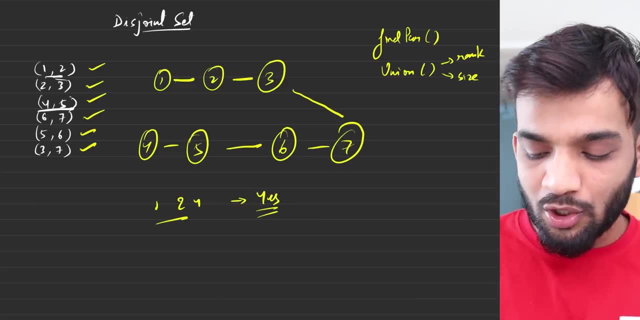 the same question: does 1 and 4 belong to like after performing all the operation? does 1 and 4 belong to the same component? Your answer to that will be yes, they do belong to the same component. Understood So you saw till here. the graph was something different. 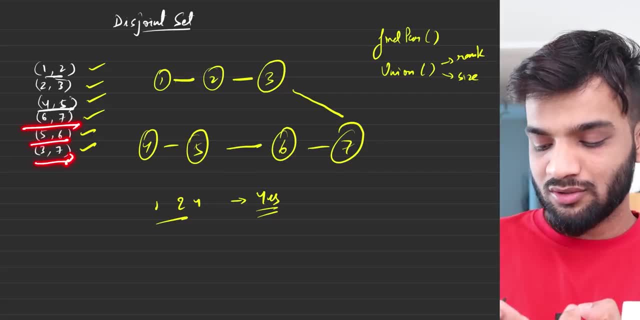 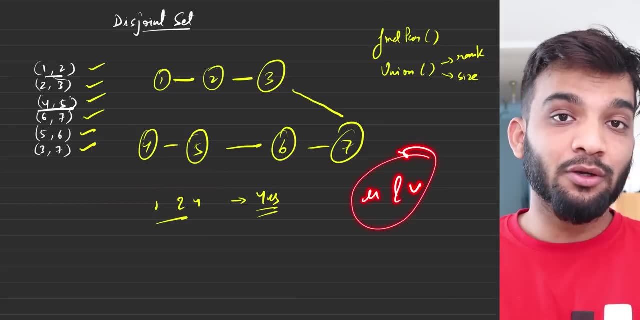 The moment you performed the next two operations, the graph was a combined one, So I can ask you this particular question, or any: u and v belong to the same component at any particular time. So this is the use case of disjoint set data structure. Now let's quickly check out what is find parent and. 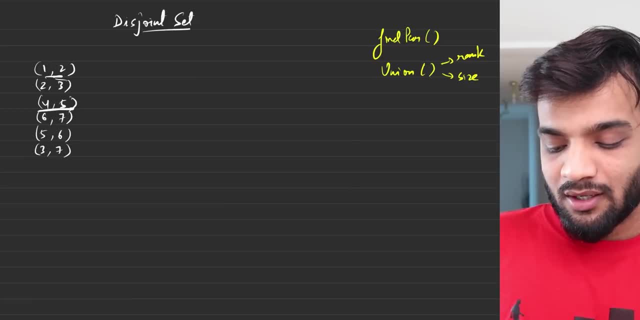 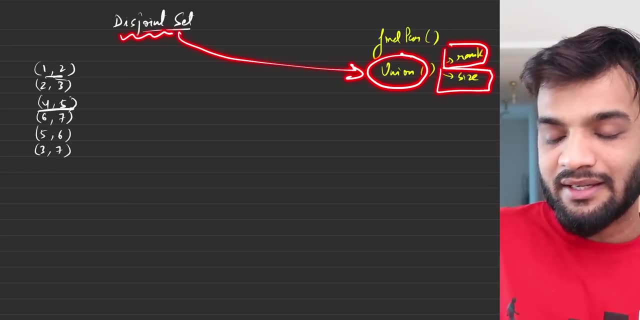 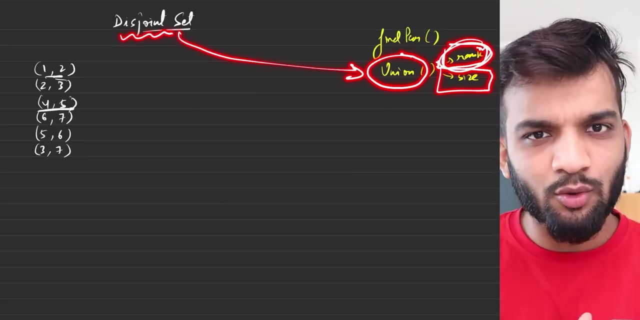 what is union exactly? So, in order to implement a disjoint set data structure, we can implement union in two ways. One is the rank, The other one is the size. So I can follow in two ways of doing it. Okay, But initially I'll be teaching you the rank, I'll be coding you up. 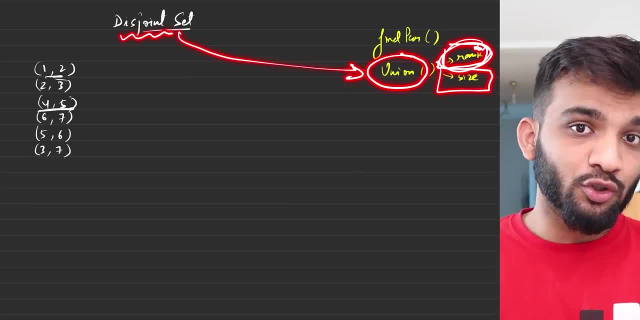 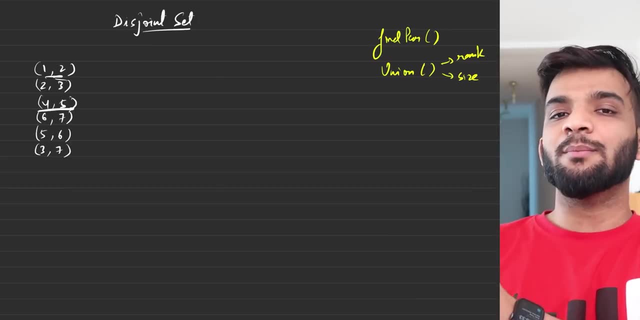 showing you how to write a clean code so that it can be used in almost all the problems, And then I'll be teaching you the size one. So the video will be the first: union by rank, then union by size. Okay, So let's understand rank. So in order to implement union by rank, we will be requiring: 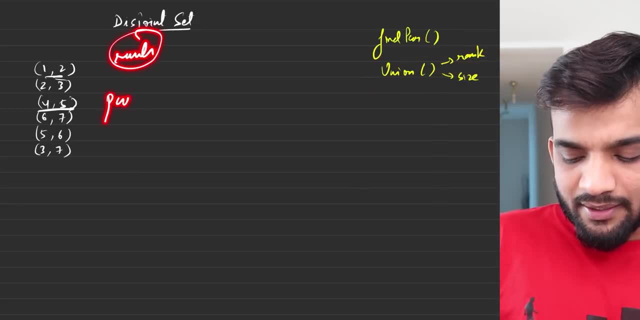 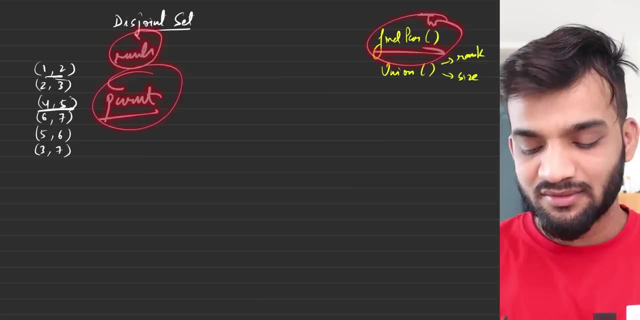 a couple of arrays. One is the rank array, while the other one is the parent array, which will serve for finding parent. I'll explain you, So let's quickly assign rank and the parent arrays. okay, so the initial configuration is very, very simple. what we do is: 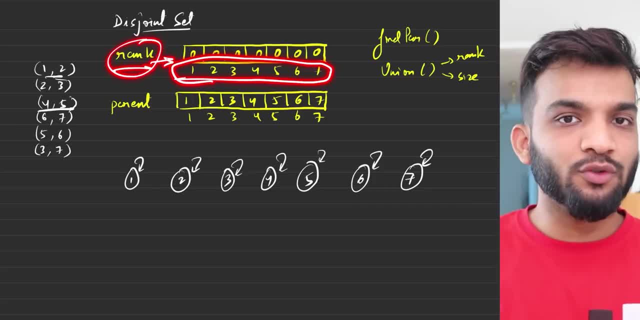 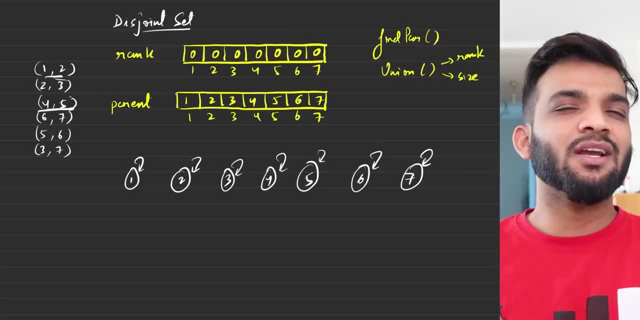 we assign a rank array with the same size of the number of nodes. since the graph is one based indexing, i start the array from one, so everyone is assigned to zero. okay, so what does rank zero mean? so if you see this particular node, there is no one beneath it, so it means there is no one beneath it. 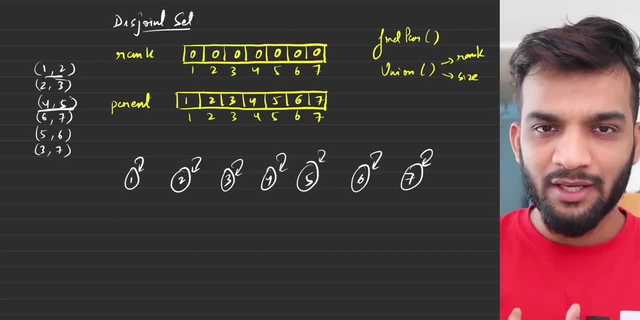 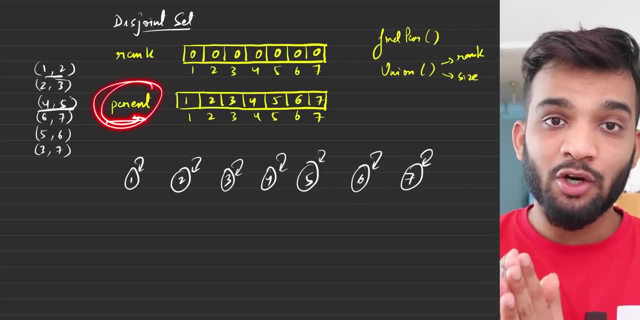 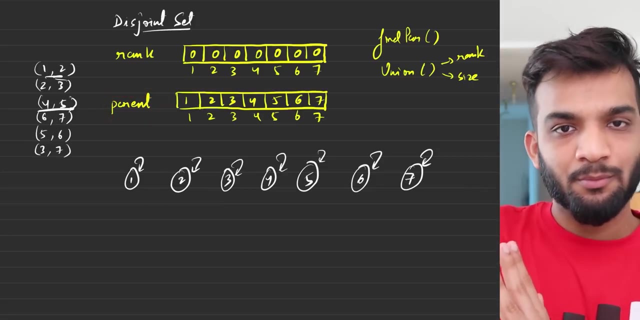 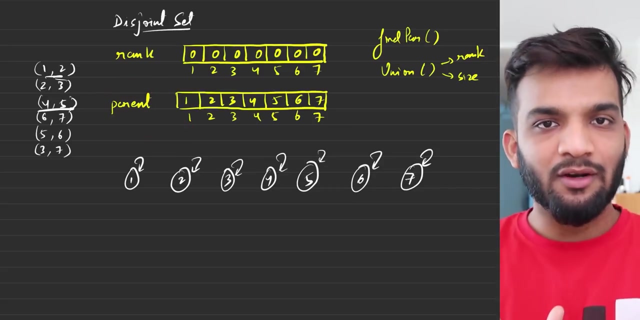 zero nodes beneath it, but eventually, with the optimizations that we will do, the meaning will change. so i'll explain you throughout the course. so now we have a parent array. now, remember, initially everyone is the parent of himself. now, what does parent mean? parent parent, okay, right above guy. that is what is the definition of the parent, which is stored here again over. 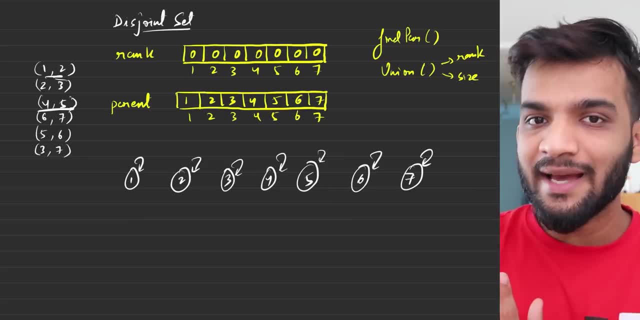 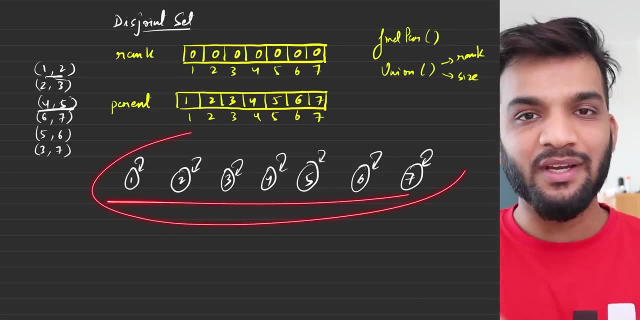 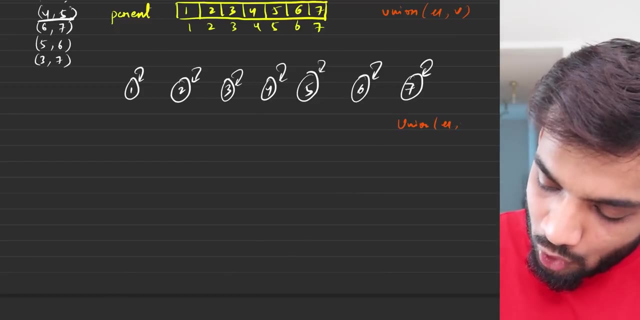 the course of this lecture, the definition of parent will change as we do multiple optimizations in order to obtain a constant time complexity. so this is what we currently have. let's quickly start the operations. so let's quickly write the pseudo code for the union of u comma v. so remember, the step one is very, very simple. the step one says: 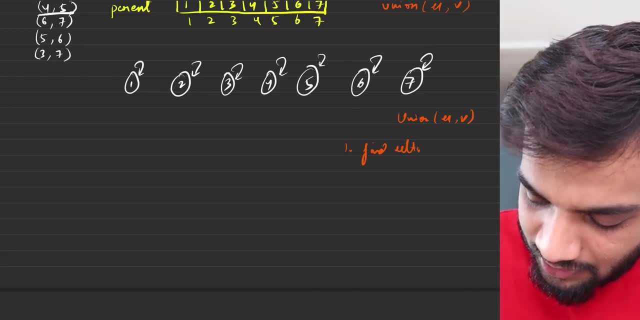 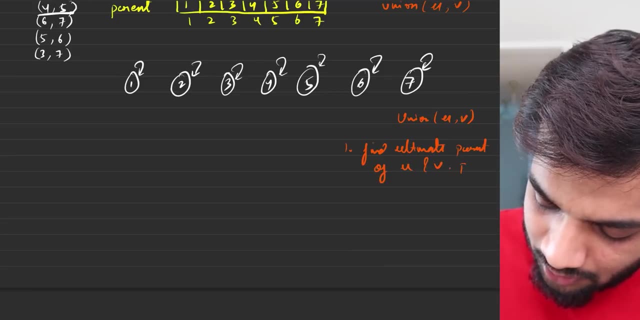 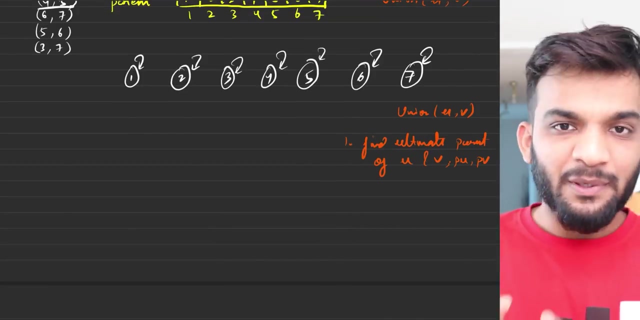 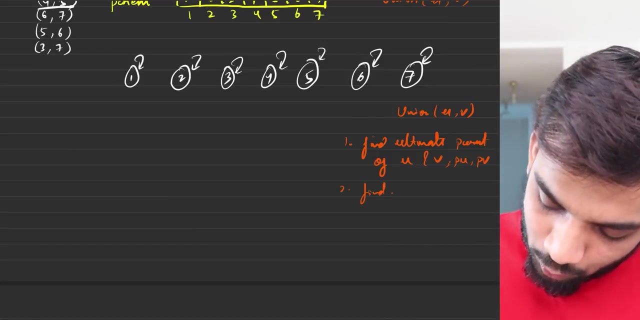 find ultimate parent. yes, find ultimate parent of u and v. what is the meaning of ultimate parent? i'll explain you. and we can term this as uh- ultimate parent, like ultimate parent of u and v. let's term this as p? u and p? v. p? u means ultimate parent of u, p? v means ultimate parent of p? v. now, find rank of those ultimate. 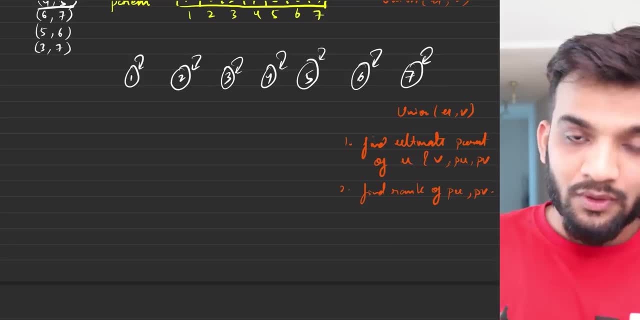 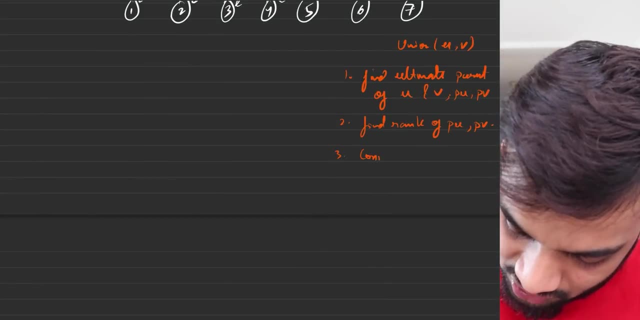 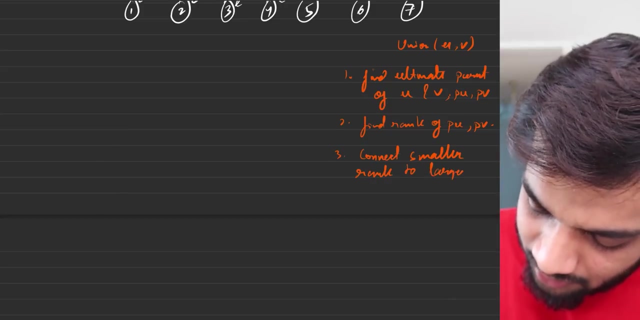 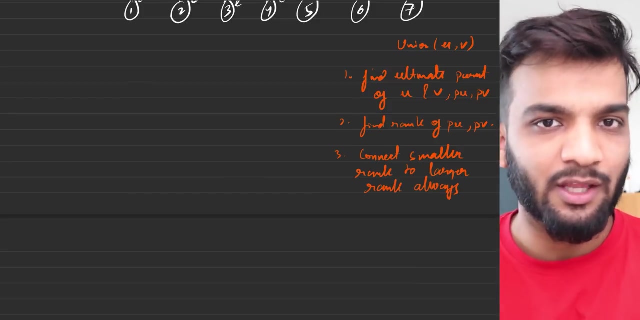 parents. find rank of p, u, p, v. find rank of ultimate parents, not u and v ultimate parents. okay now connect smaller rank to larger rank. connect smaller rank to larger rank. always in case of duality, you can connect anyone to anyone. we will explain that as we move. okay, cool, we have. 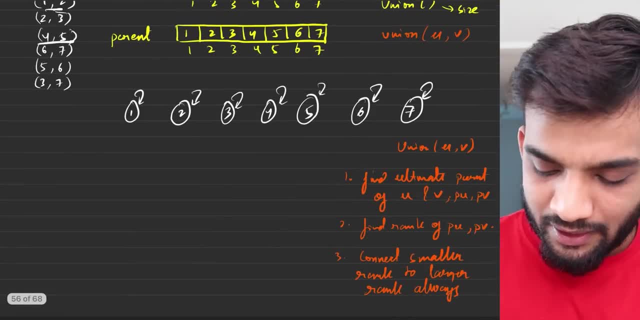 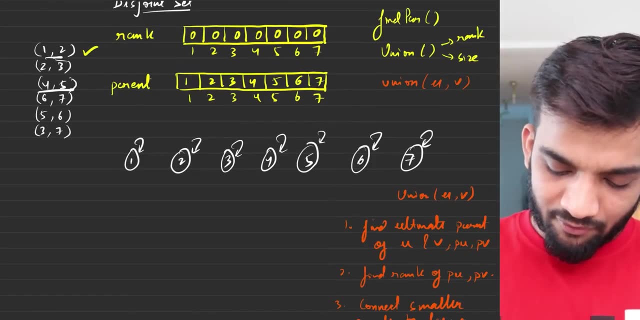 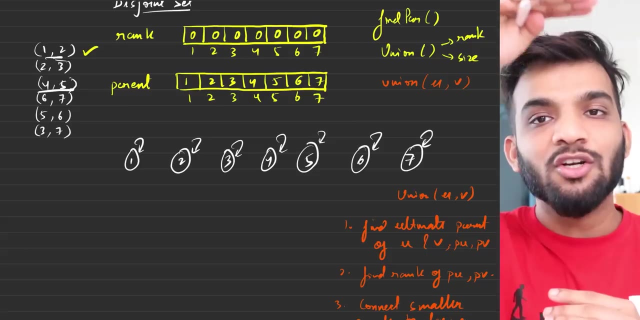 understood, or i've written the pseudo code. okay, let's now quickly, uh, check out the first operation that has been asked for us. it says union of one- two. so what i do is i have one, so i go and look at the parent of one. what is the ultimate parent? you have a bunch of nodes. the guy at the top is 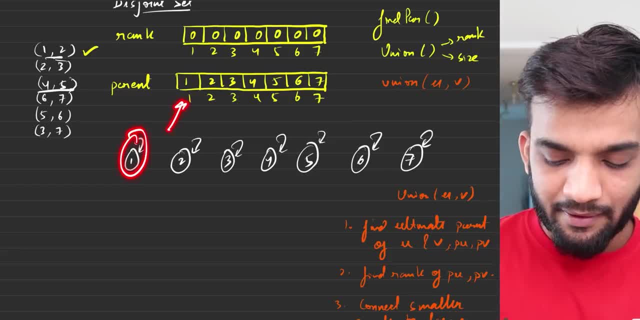 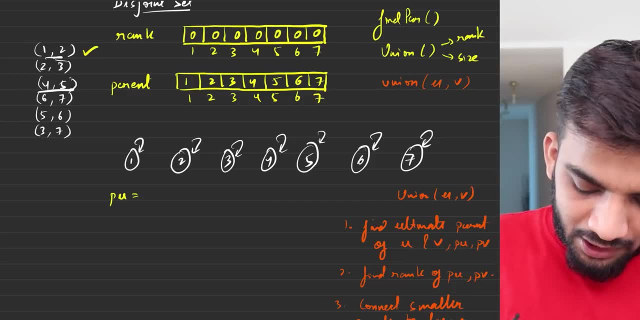 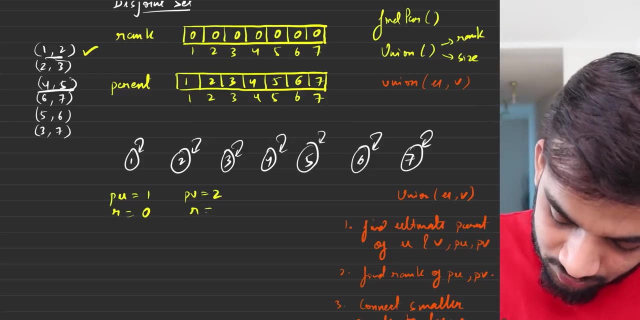 known as the ultimate parent. okay, so for one, who is the ultimate parent? one itself for two is the ultimate parent. so i can see, as of now, the ultimate parent of one is one and the ultimate parent of two is two. what is the rank of both? can i say the rank of both is, as of now, zero, if you. 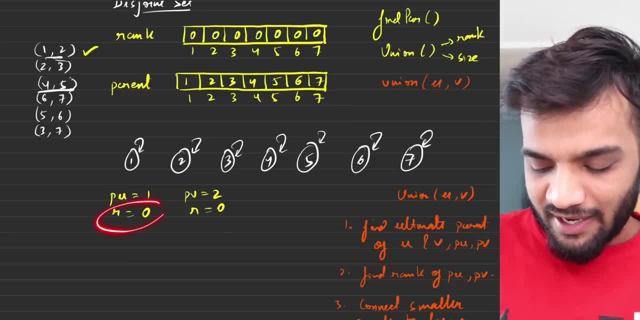 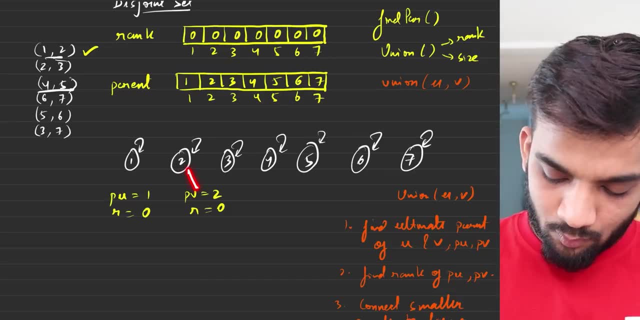 carefully see. both the ranks are zero, so if they are equal rank, you can actually connect anyone to anyone very, very important. you can go ahead and connect. either you can connect like one here, or either you can connect two, which is completely your choice. so what you do is you will go ahead. 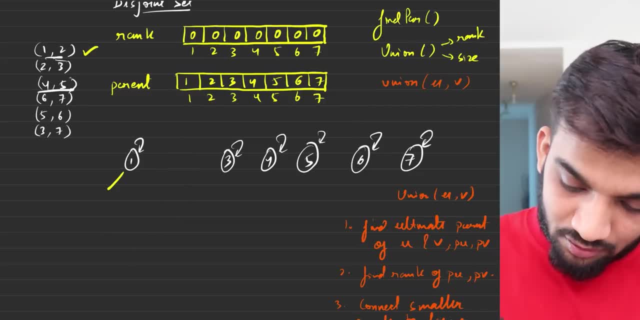 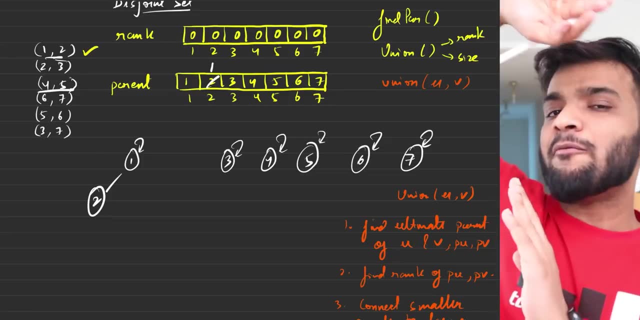 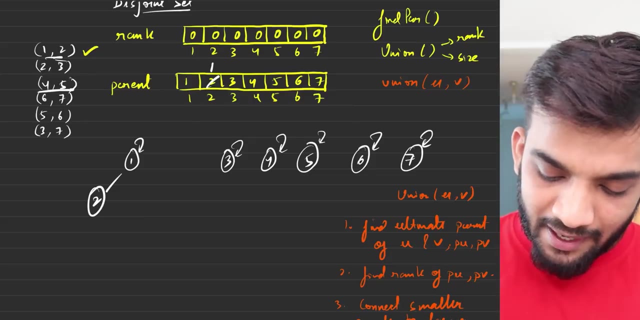 and take this two, say: can you please connect with or? i can change the color, can you please collect, connect with two? and you'll go to that. now your above parent is one. now, remember you connected two to one right. both of them had same level, both of them were equal height. you took it and connected, so the 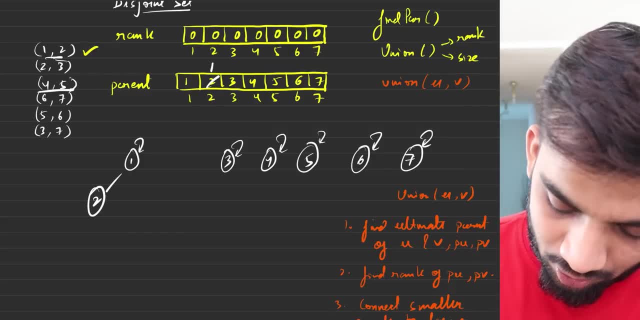 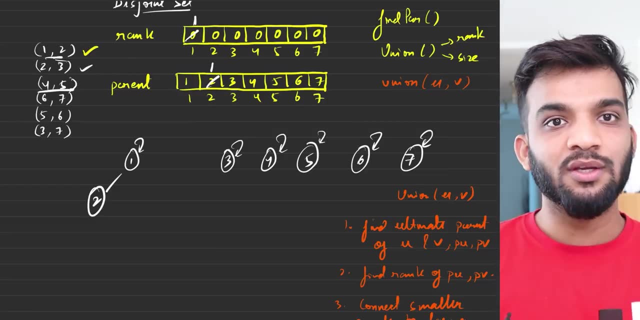 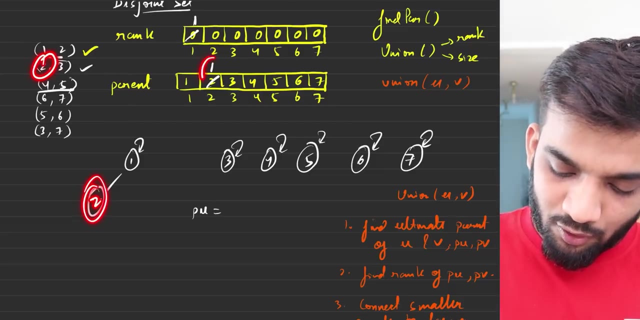 height increased, and if the height increased, the rank will also increase by one. the rank will also increase by one. done perfect, next two, three. and this is where, again, the next thing comes: who is the ultimate parent of two? let's use the ultimate parent of two. it's one over here and is the one. 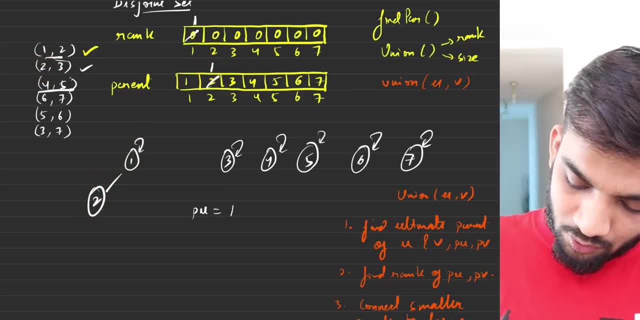 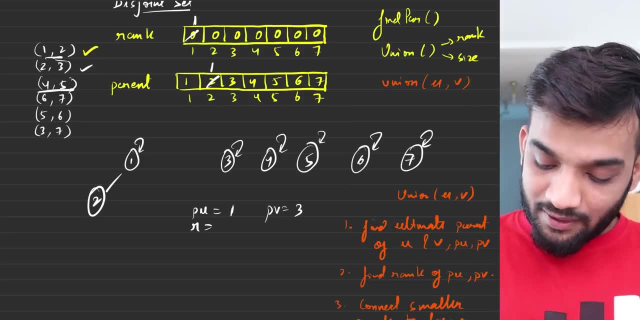 the top guy. it is so. the ultimate parent of two is one. who is the ultimate parent of three? be itself. what's the rank? rank of this particular one is one. rank of this particular three is three. if you, one is one, three is zero. sorry, it will be zero. 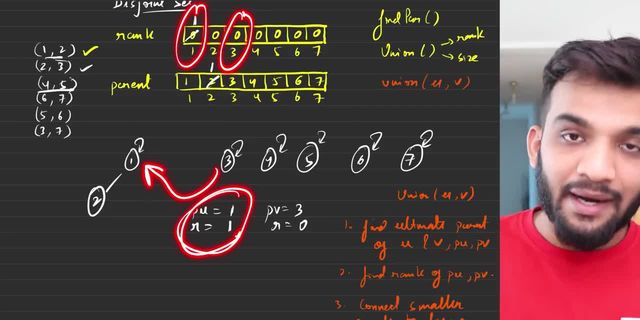 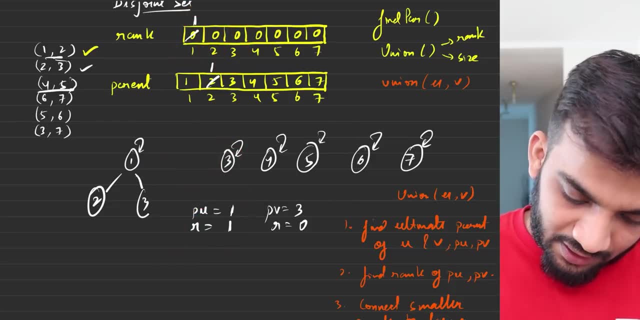 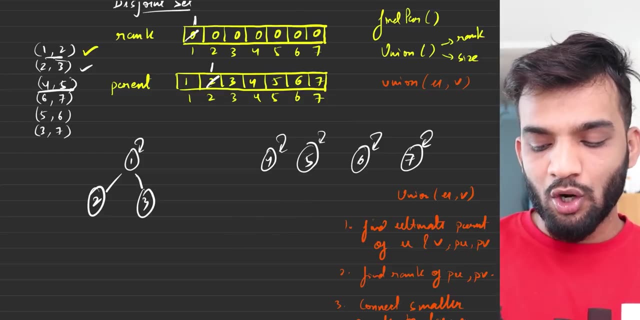 who is the greater guy? this one, so three will come up and get connected to the smaller guy. comes up and gets connected to the larger one, so three is connected to this. now i'll go and erase this connected. do i do anything to the ranks? no, you will not do anything to the ranks. 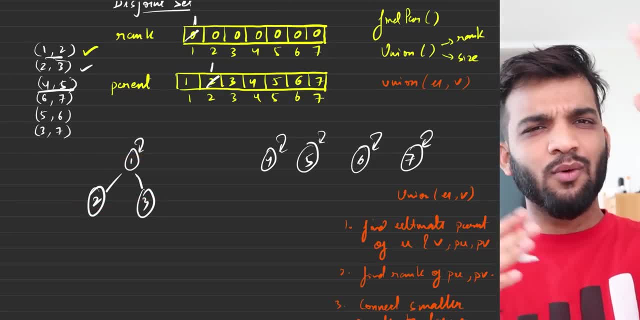 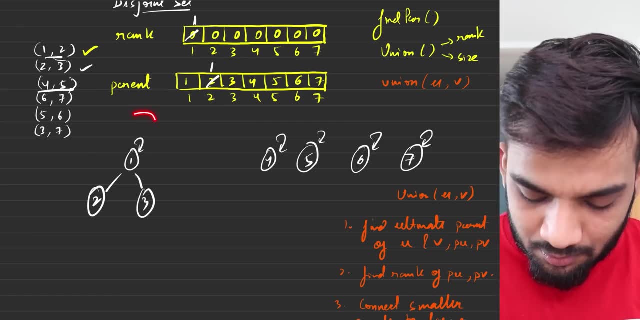 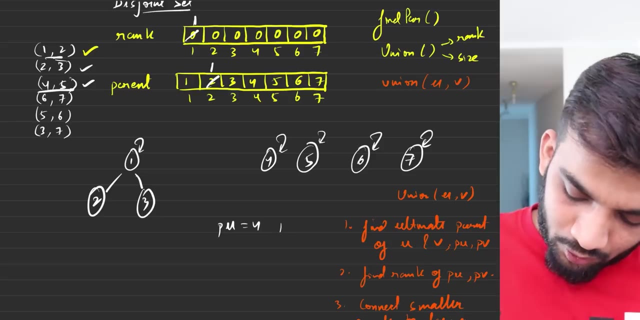 why? because it still has a height of one. because you connected a smaller to the larger, so the larger is not going to increase, it's not going to increase, so thereby we keep the same height, perfect. next, connect four and five. who is the ultimate parent of four? four is the ultimate. 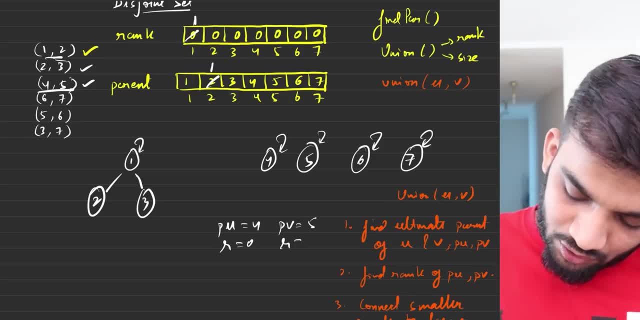 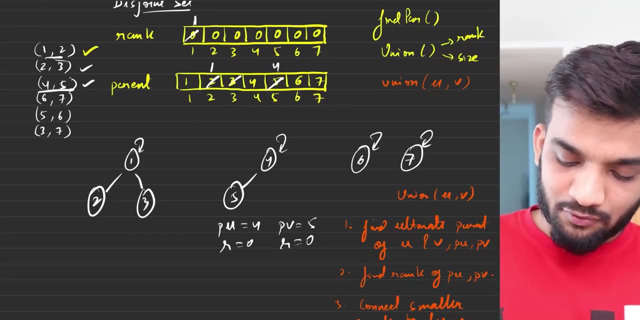 parent of five. five. what's the rank? zero, zero. connect any one to any one. so what i'll do is i'll go ahead and connect five to four and i'll erase this. i'll increase, i'll update the parent of five to four and the other thing that, uh, by the way, i forgot to update the parent of three. 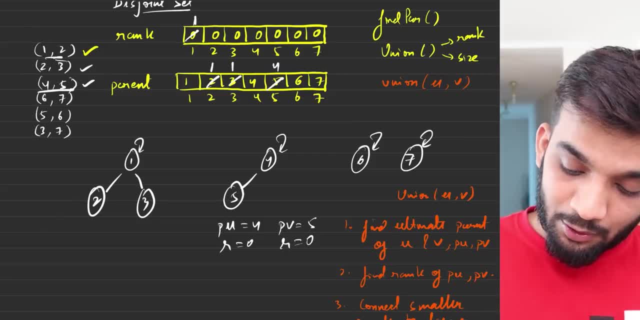 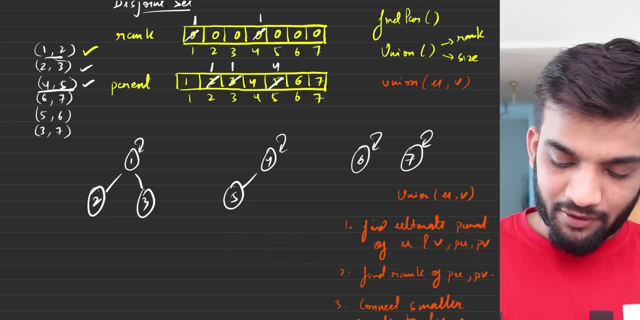 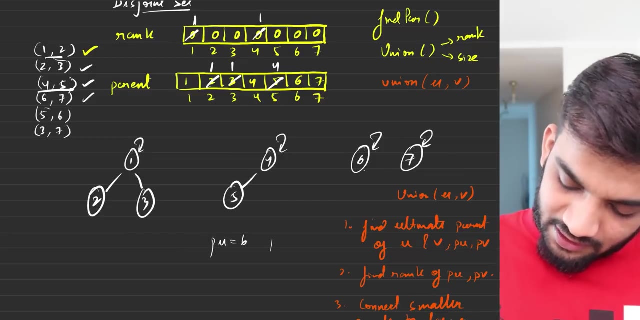 it will be one. so what the other thing i'll do is i'll increase the rank by one, because two same guys connected. height increases. so done perfect. next, connect. so what is the next thing? connect six and seven. so ultimate parent of six is six, ultimate parent of seven is seven. 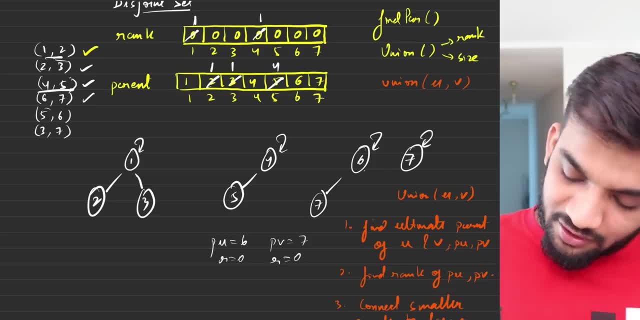 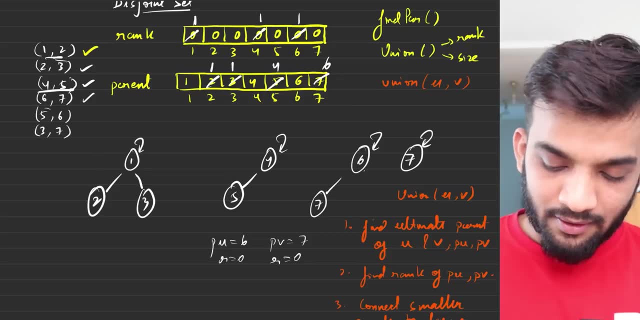 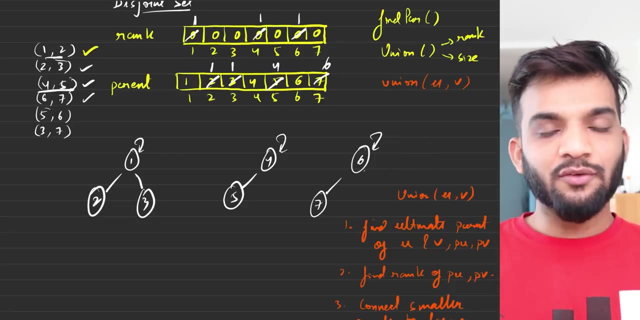 the ranks are zero. so what you'll do is you'll connect seven to six. you'll update seven's parent to six. you'll update the rank of six to one. this is how you can easily connect the perfect. done so, apparently, i can just remove this as well. so, as of now, this is where we stand. what's the next thing? it says: connect five and. 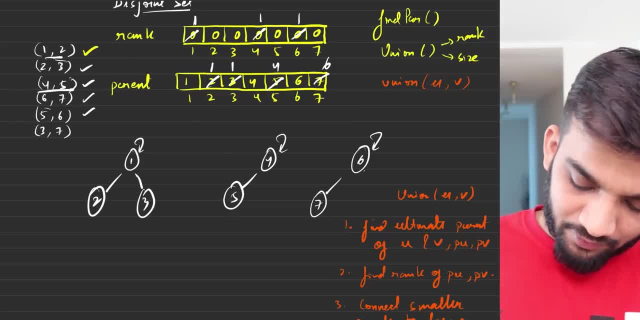 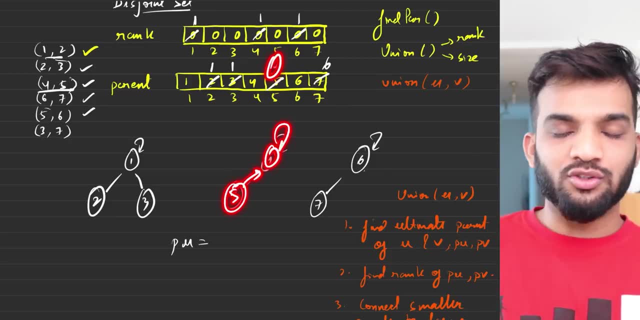 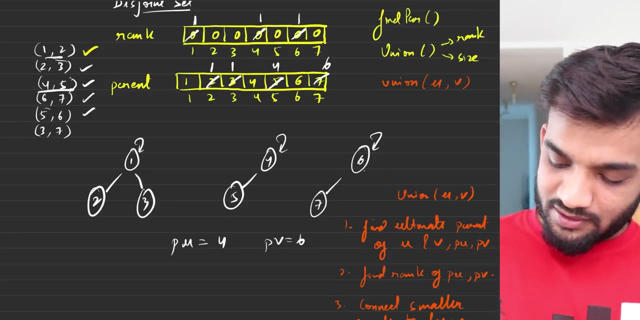 six, so perfect. so who is the ultimate parent of five? let's see. ultimate parent of five. five is here, so five's parent is four. who is actually the top boss? who's actually the top boss? so he's the ultimate parent. now i've been asked to connect six, so six parent is six. six's parent is six. 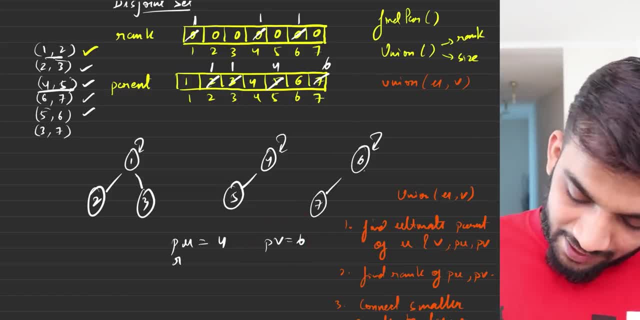 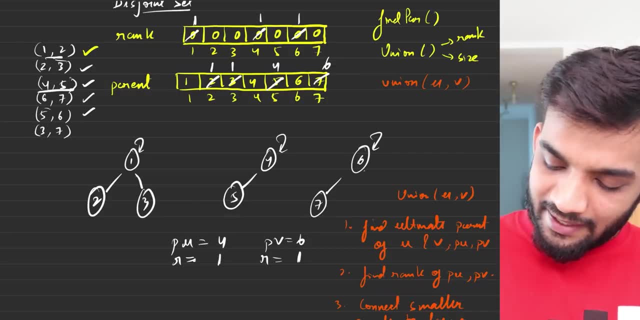 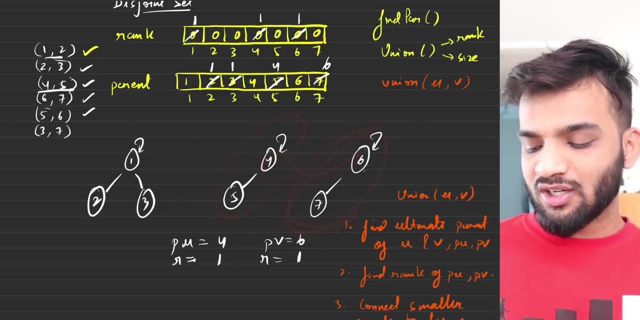 himself. so ultimate parent is six. let's write the rank: rank of four, if you see is one, rank of six, if you see is one. do you agree? you do agree. so apparently i can say that, okay, fine, we have someone of the same ranks. so either this can go and get attached here, either this can go and 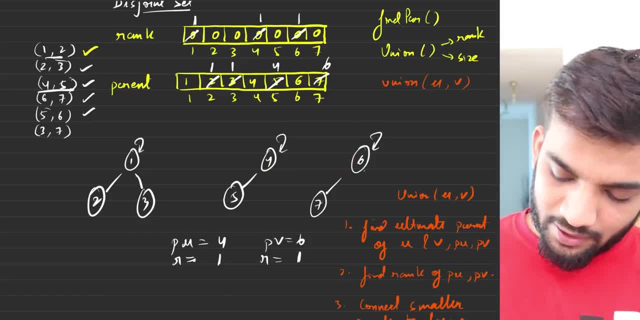 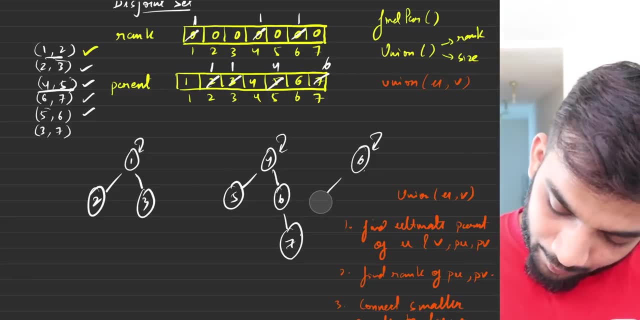 attach it so you can do as you wish. so what i'll do is i will just go ahead and take the six and make it attached to seven. i'm sorry to four done and now i'll omit this. you can do as you wish. so what i'll do is i will just go ahead and take the six and make it. 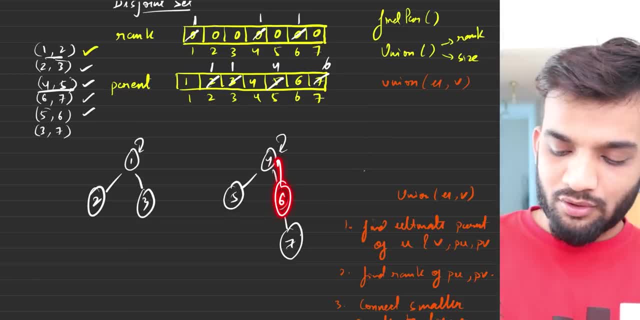 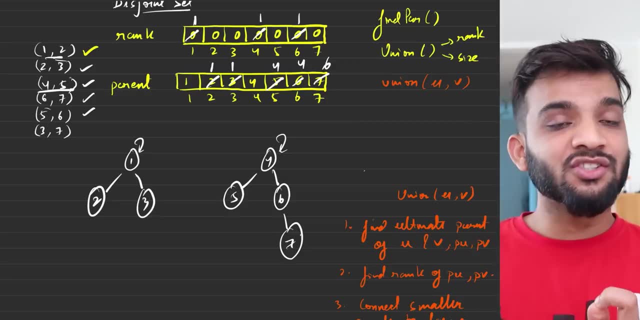 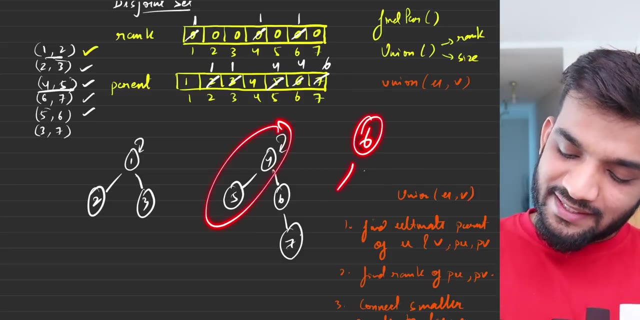 remember one thing: you attached six to four, so the parent of six will be four, the parent of six will be four. remember this very, very well, okay, next, what is the other thing that you will do? you will have to increase the rank, why? because you had four, five, you had six, seven, both of the. 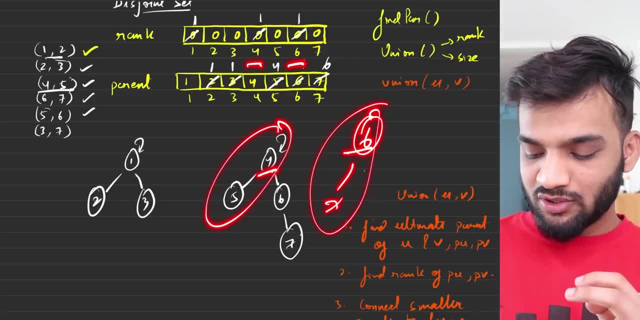 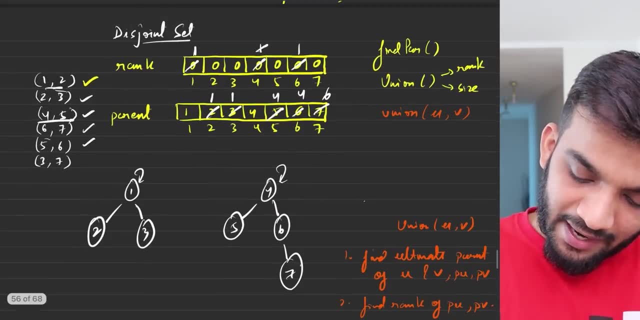 ranks. if you carefully see four and six at a rank one. so since you attached same guys height will, if you see the height increased. so apparently you go ahead and say the rank to increase by one more, so the rank will be two. so this is where we stand till we have not performed the 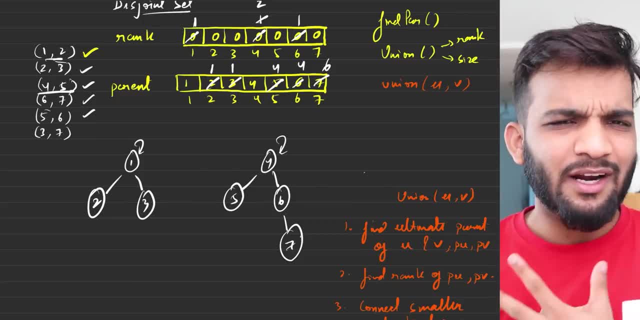 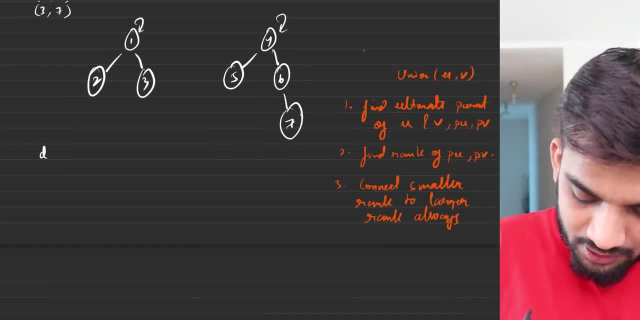 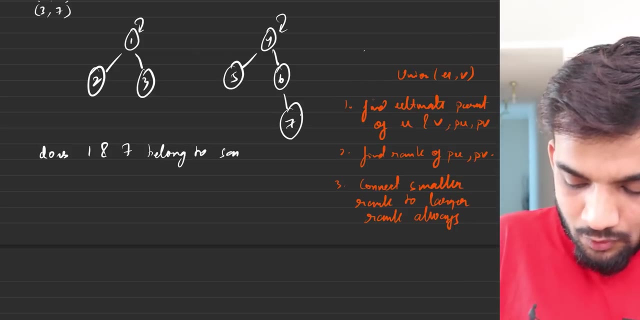 last step now if, if kyle kind of understood everything. now suddenly if someone comes up and says: does, let me write it. uh, does one and seven or do one and seven belong to same combo? if i ask you this question, the answer is no, but how will you find out? this is where 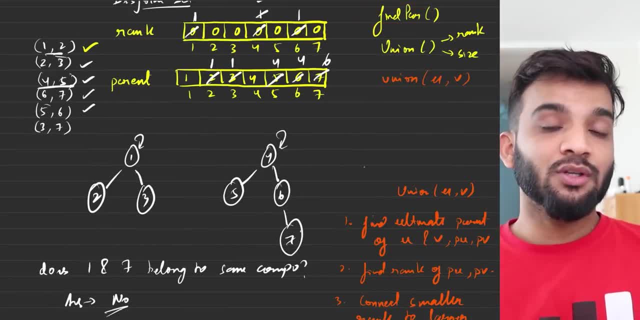 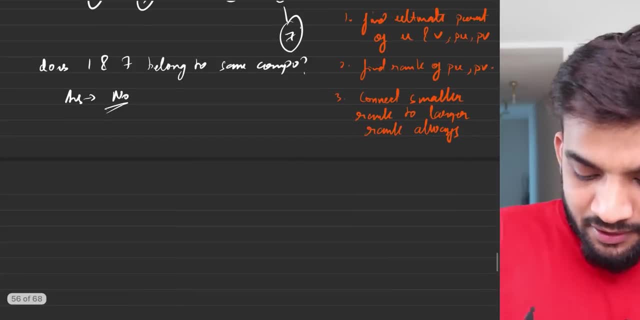 something like find parent will help. this is where something like find parent will come into picture. okay, so since i'm saying find parent will come into picture, let's understand. so when i'm seeing does one and seven belong to the same component, i look at the parent of one: it's one. 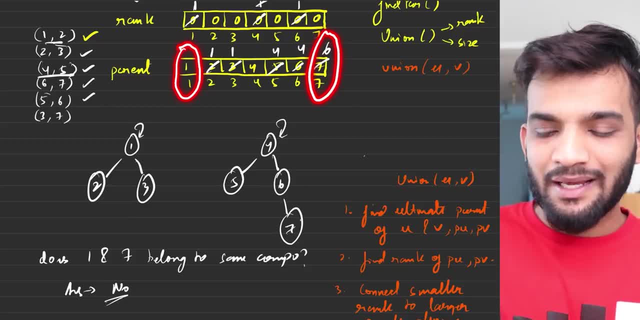 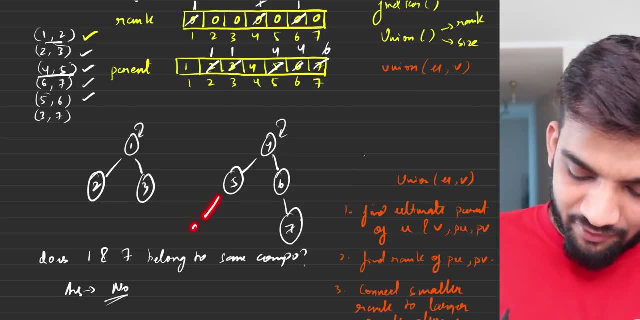 i look at the parent of seven, it is six. so i'll be like, okay, the parents are different, they are not. but wait, you should not do like this. just imagine you were having a eight here. imagine, right, i'll ask: does eight and seven belong to the same component? i'll ask: does eight and seven belong to? 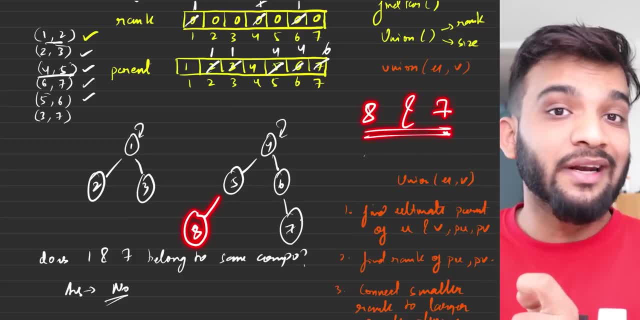 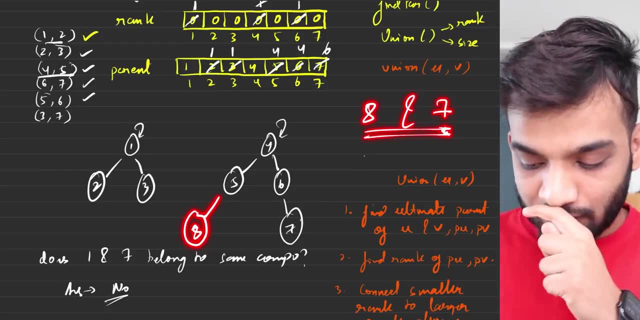 the same component. now something to notice: we are not creating a graph, we are creating a different data structure over here. a graph is not being created, okay, a different data structure is being created. if i ask you if eight and seven belong to the same component? ideally they should, but if you. 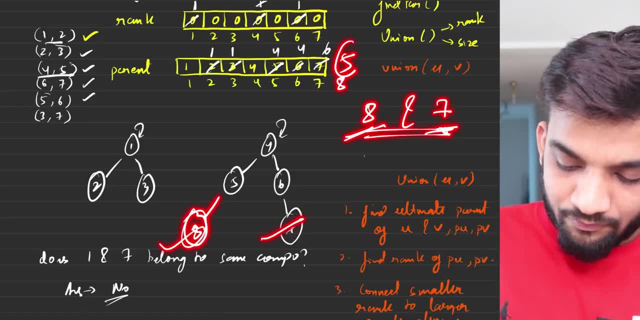 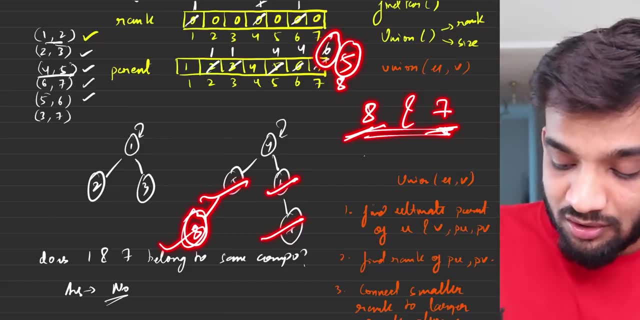 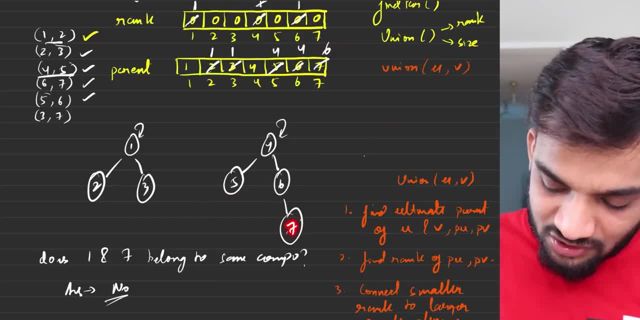 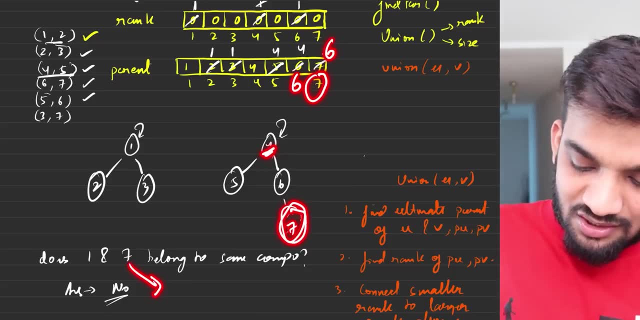 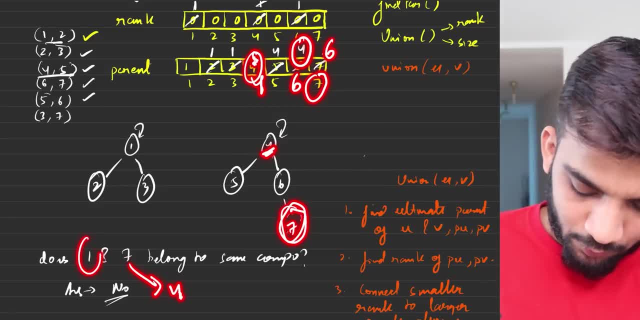 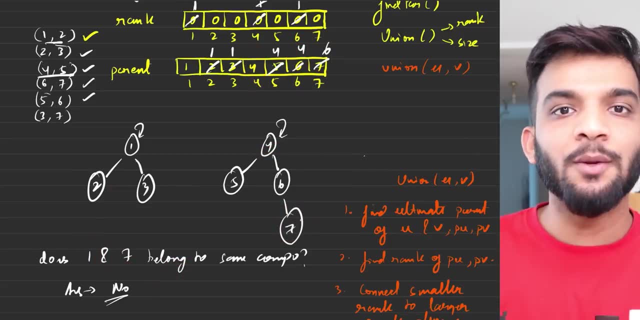 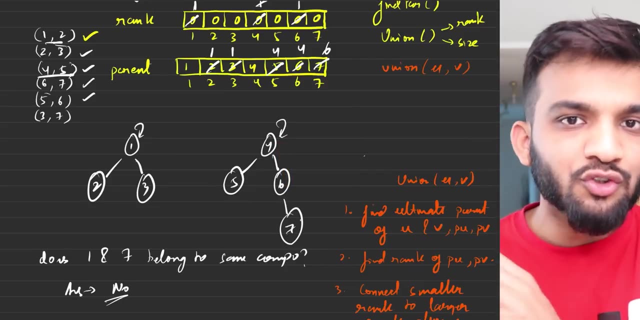 parent. ultimate parent boss is four and the boss for one is one, so both have different ultimate parents. if both have different ultimate parents, you say they do not belong to the same component. use of find parent. now, since you are creating a kind of a tree structure, the tree will increase. 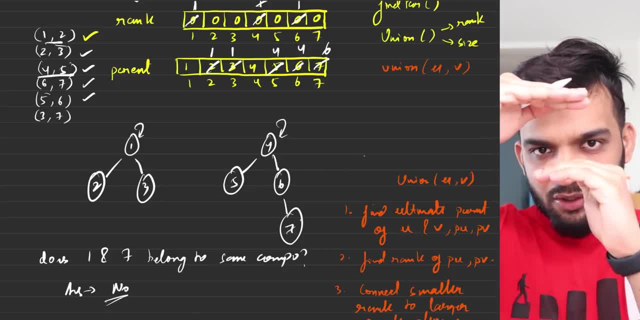 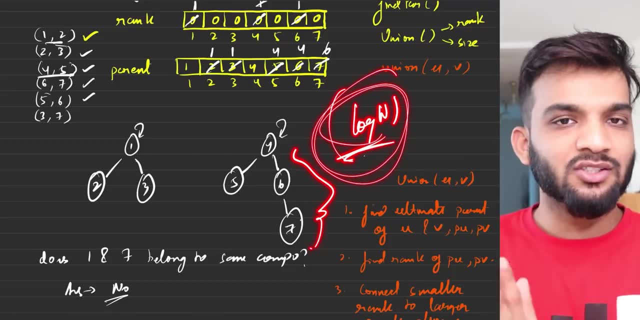 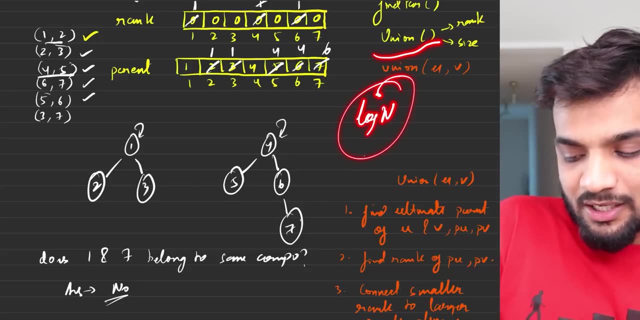 in depth. with more number of edge additions, the tree will increase, increase, increase, increase, so it will end up taking log n. it is theoretically proven that you will. the tree will increase and end up taking logarithmic of n if you just apply union by rank. because in order to find the parent, 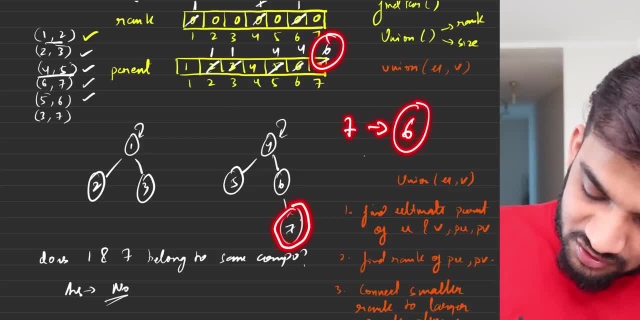 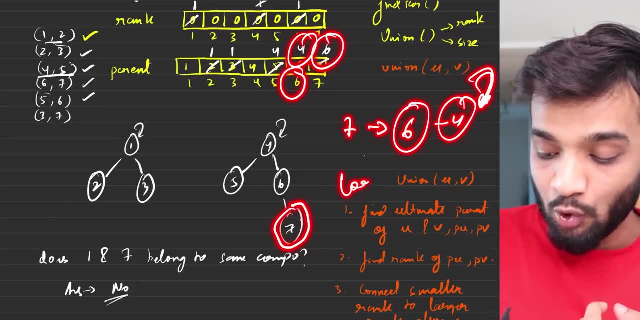 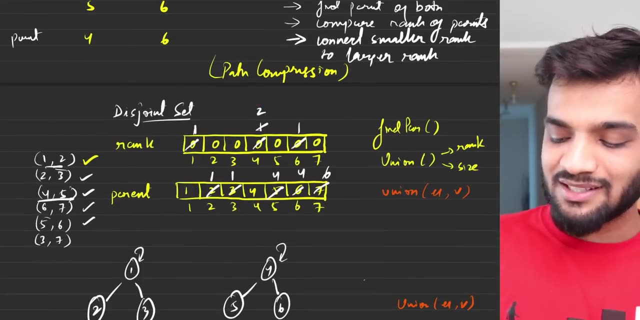 of seven, you have to go from seven to six, from six you have to go to four and at four you find he is himself. so you get the top boss or the ultimate parent. that's going to take you a logarithmic of time, but wait, but sorry, you said it works in constant. it does we apply something as? 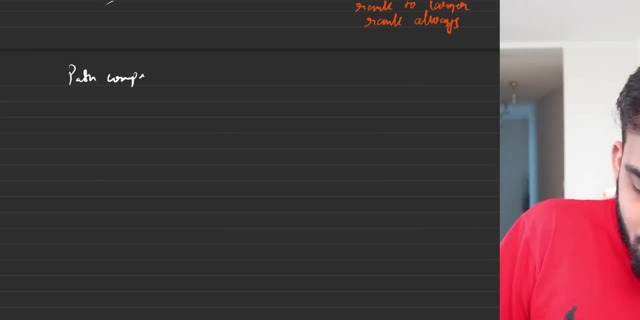 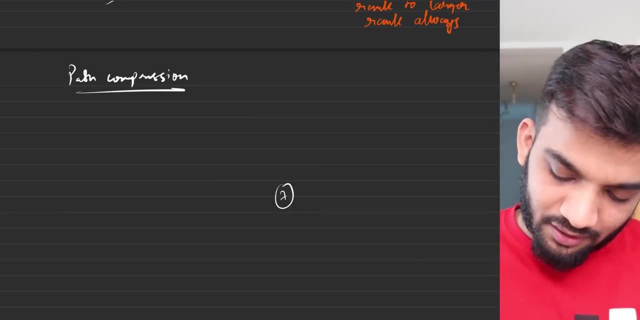 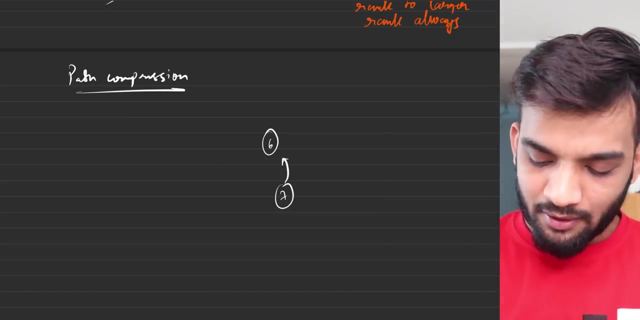 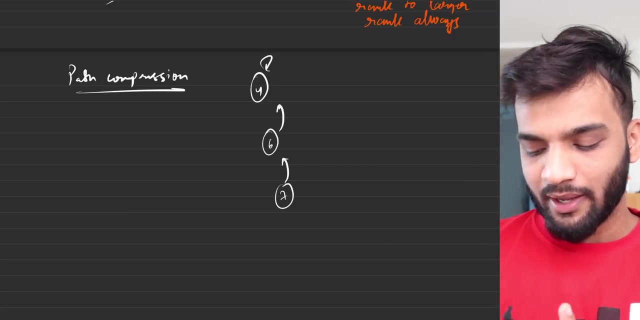 path compression. okay. so what i do is i say: okay, someone did ask me to find the parent of seven. so what did i do? i went to six because six was his right father or the next parent, and six's parent was four, and four says i'm the parent. so you can write something like this: okay, i went from seven to six, six to 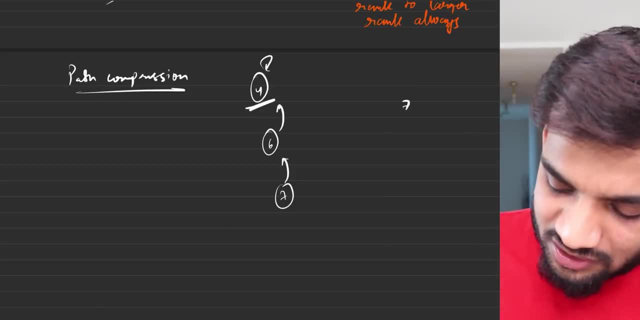 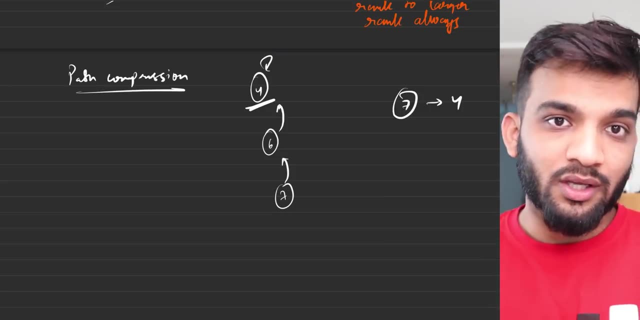 four. so i know the four is the parent. so once you have figured out, seven's parent is four. and since we are just dealing with parents- and that is what i require, because our aim, main goal is to figure out who is the ultimate parent, so can i say: 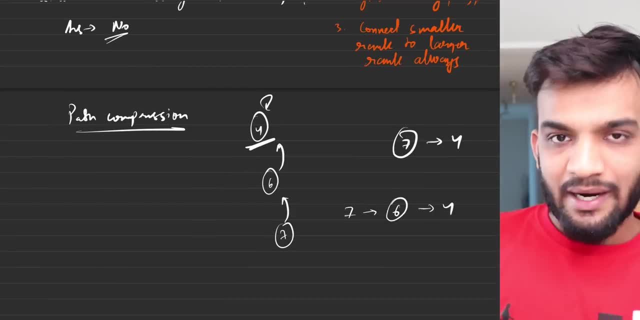 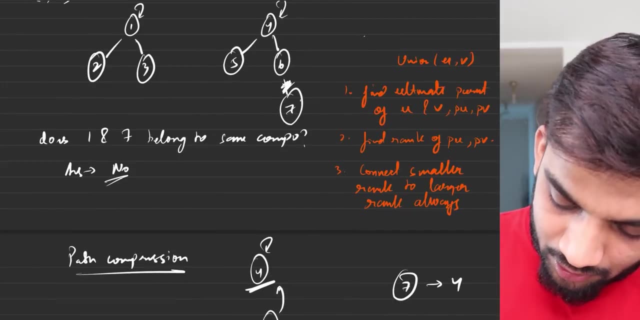 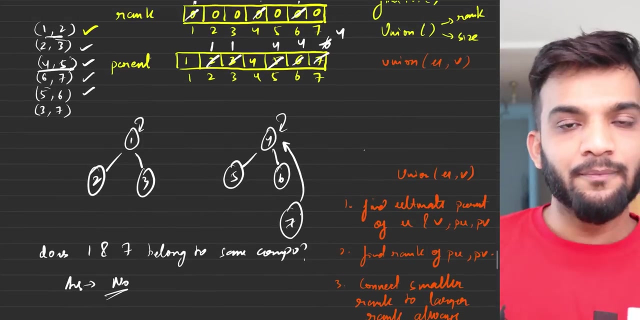 once i've gone to seven, to six, to four, and once i figured out the parent of seven is four, can i actually say: let's, i don't need this link anymore. or i don't need this link anymore because i know seven's parent is now four. so can i change seven's parent to four? i can, because the next time, if 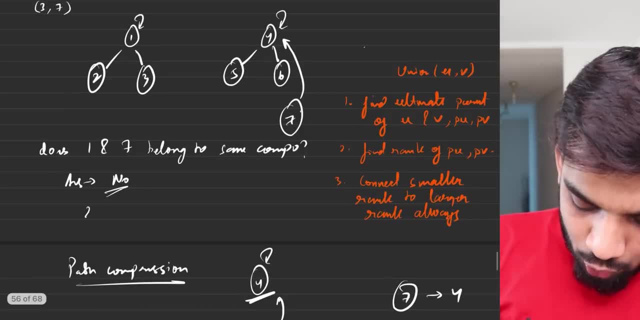 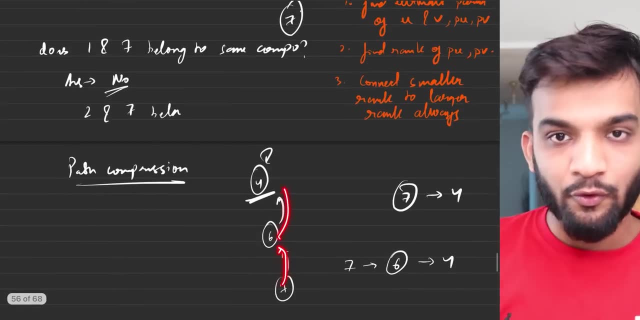 someone again comes up and says me: hey, does two and seven belong to the same component? and you again go and call find parent. you will not move like that. you will not be able to find the parent like seven, six, four, because this time seven will directly go to four and it will find him to be the. 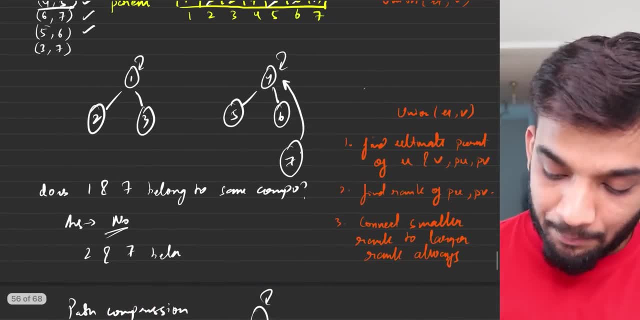 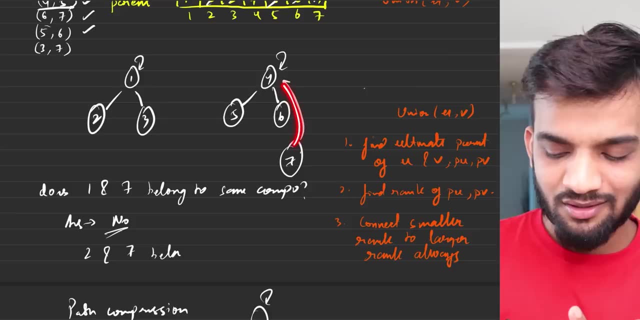 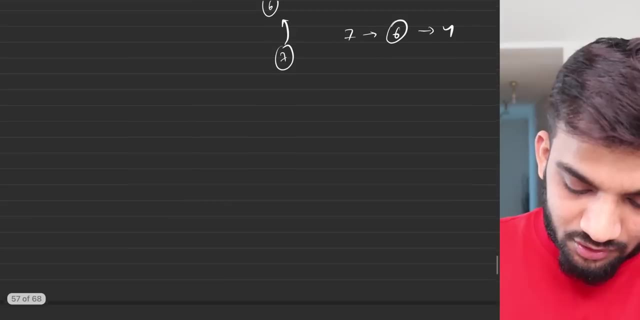 boss. so you did a path compression. you did a path compression. you said once: i will just compress you. and then i know that, hey, listen, your parent is this guy. i know this, i don't need to go via six. imagine the tree to be longer. imagine the tree was something like this, just imagine. 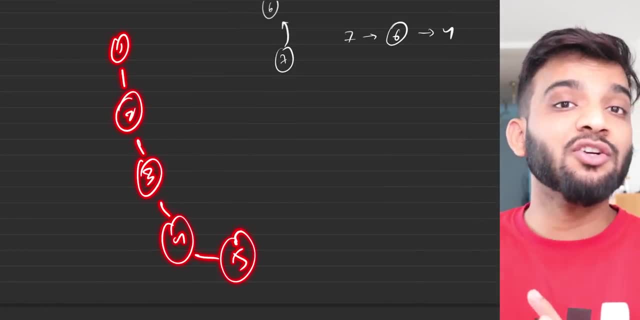 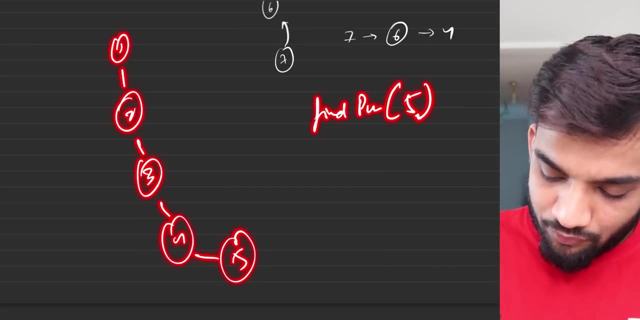 take it as an imagination. imagine the tree was something like this and someone said: find the parent of five. so what would will you ideally do? you'll go to five, you'll go to four, you'll go to three, you'll go to two, you'll go to one, and at one you'll find he's the. 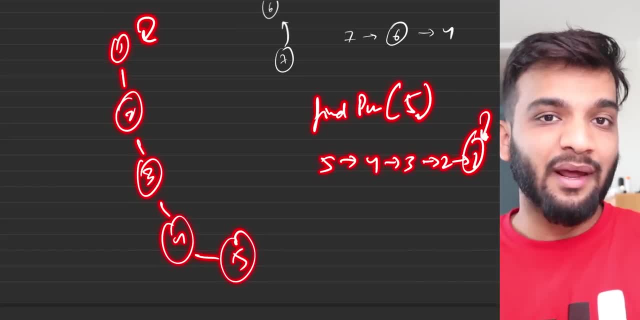 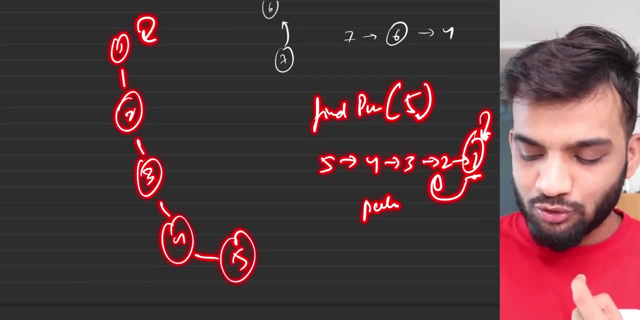 parent himself, and you'll say: one is the parent. you'll say: one is the parent, but what i will do is i'll do a path compression. i know one is the parent and one will be the parent of two also, so i'll say: two is directly correct. one will be the ultimate parent of three as well, so i'll say: 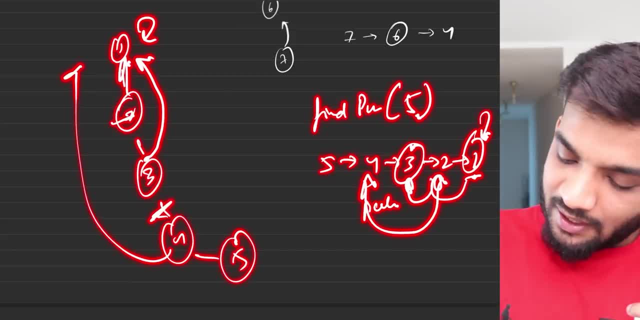 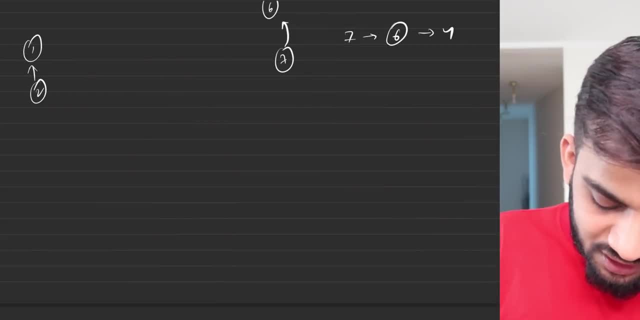 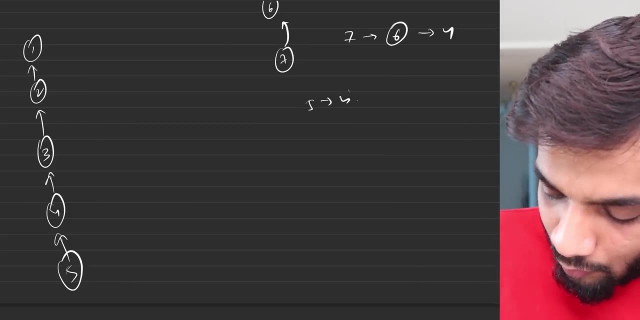 one will be the ultimate parent of four as well. so i'll just remove this and say- and i know five ultimate parent will be one. so apparently a tree, which was something like this: if you do path compression on finding parent of five, four, three, two, one and you get two as the 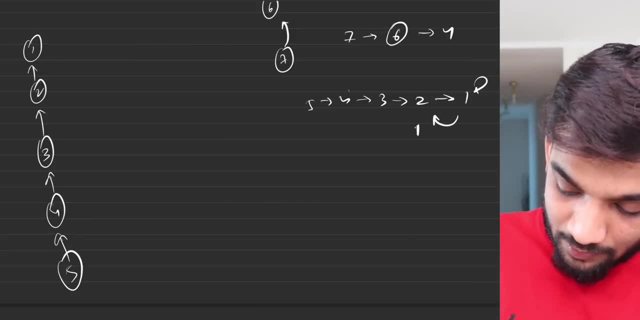 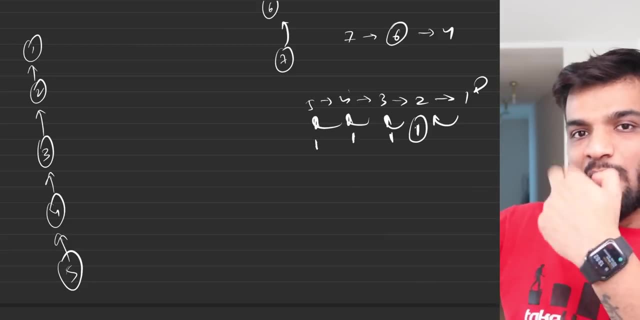 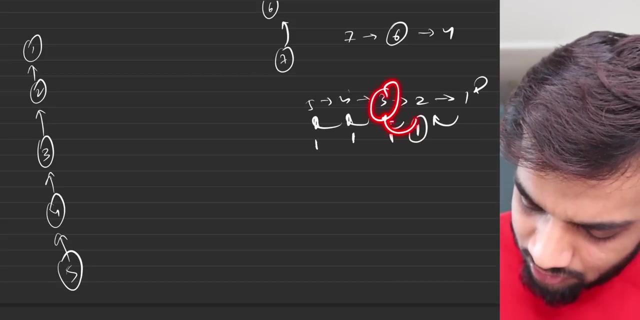 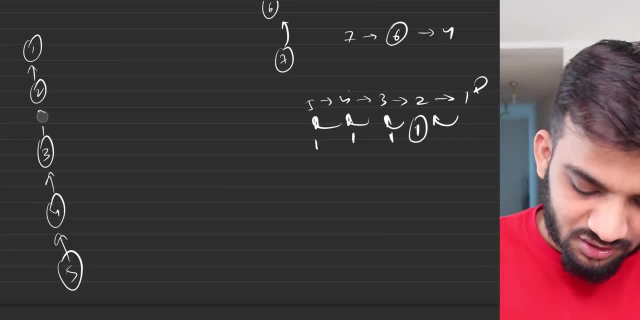 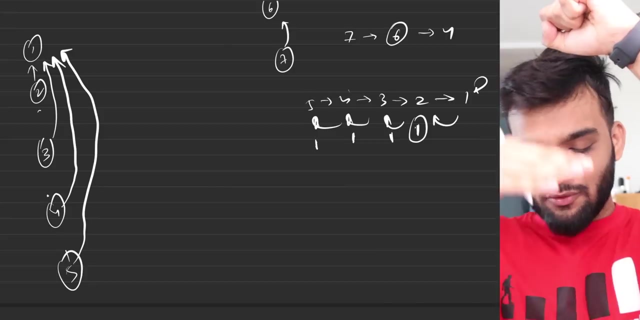 getting connected to two. three, like yes, does make sense. let me connect to one. four will be like yes, i'm also wasting time. i will be like i'm wasting time. everyone goes and gets connected. so this is how the graph will change now: under one, we will have two. we will have three, we will have four. we 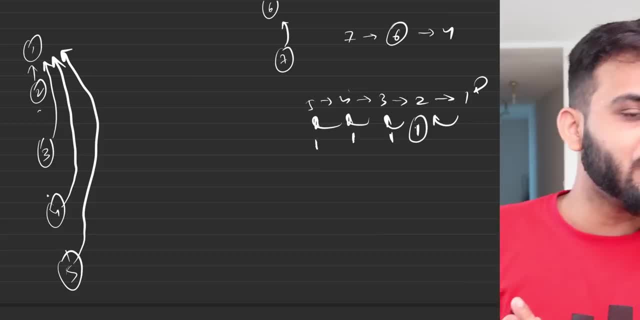 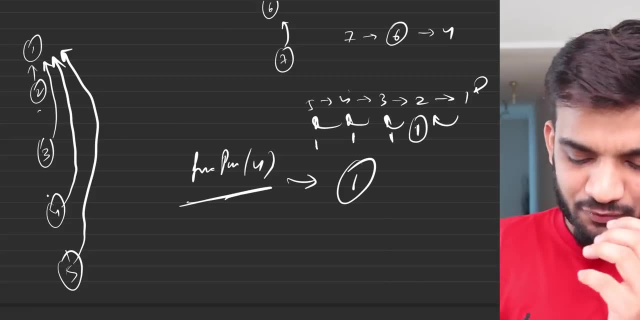 directly. yes, so you know, this is for sure. and next time when someone comes up and says find parent of four, i'll be like array one direct, low one, because four is connected to one and one is the ultimate parent. someone comes up and says, find parent of five, take one. one is directly. 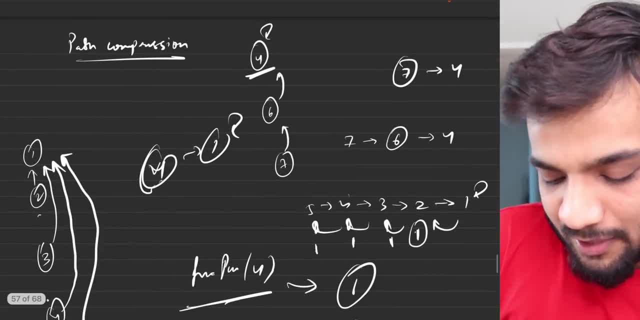 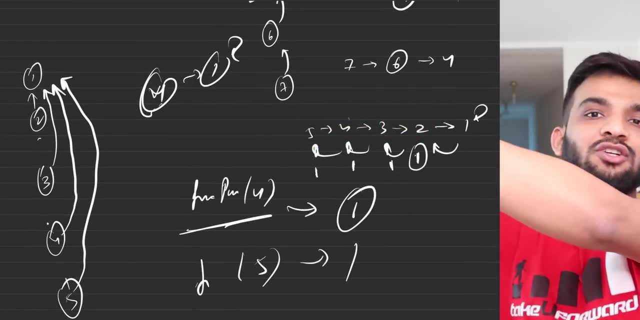 connected ultimate parent. so this is what the path compression technique is. if someone is asking me parent everyone in the path whom i encounter, i'll replace their links and attach it to the direct parent. but here comes a slight twist. i'll attach it to the direct parent, so it's fine. 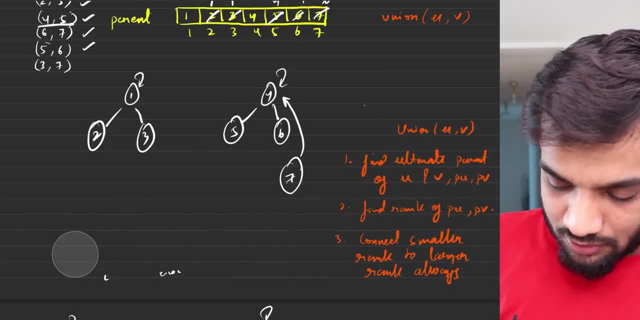 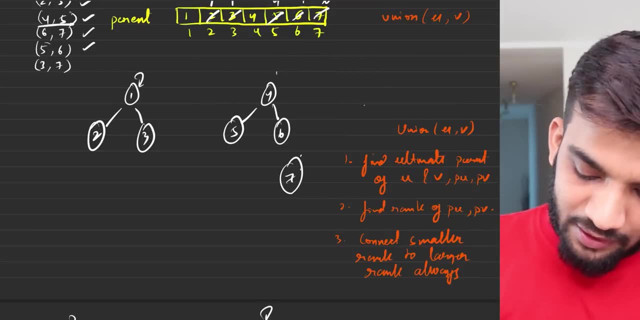 so what we usually do is we attach it to the direct parent, and that's what we call as path compression. okay, remember this. so as of now, we have something like this: now what will happen? the next three and seven will come, so i'll be like you have to attach three and seven, so we know. 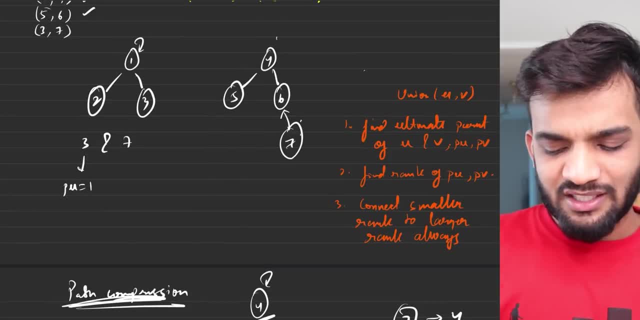 three's ultimate parent is one, and that's very easily found, because three is the ultimate parent of four. so we attach it to the direct parent and that's what we call as path compression is directly attached to one. but when i try to find out- find out the seven, i'll have to 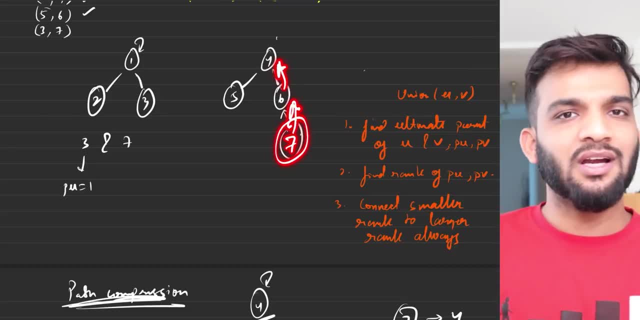 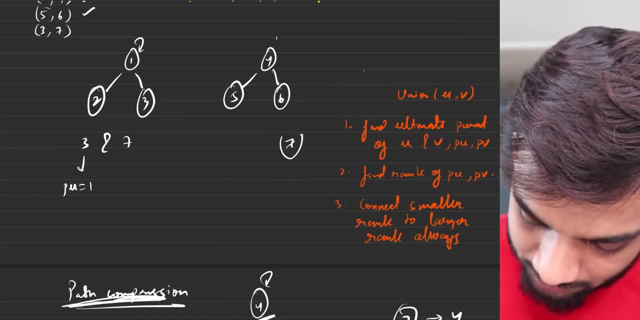 find the parent of seven, which goes to six, which goes to four. and in order to find the parent, we will end up doing a path compression. we will end up doing a path compression. so let's be honest, let's do the path compression, which will be something like this, and i'll find the ultimate. 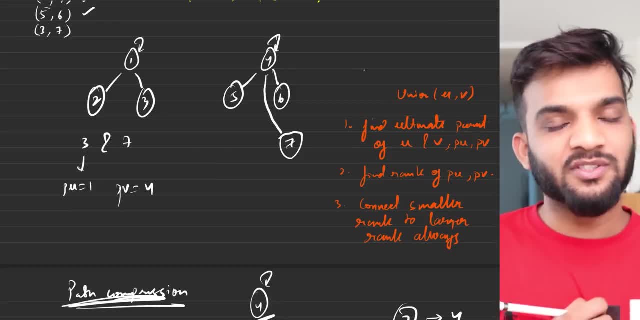 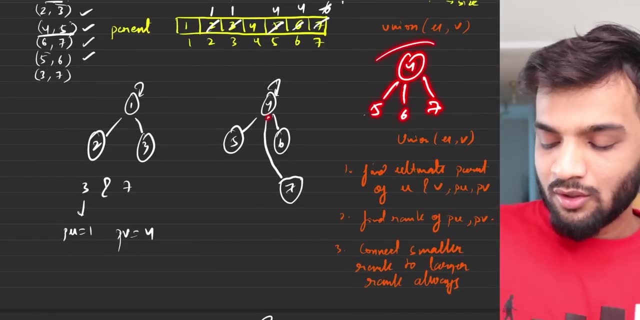 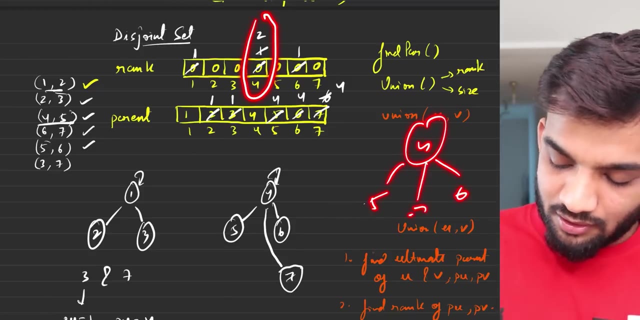 parent of seven to be four, who is connected to himself. right, but if you do this, the tree will be something like this and the rank of four, if you carefully observe, is two, but actually you have five, six and seven. ideally, the rank will also decrease, but we cannot do it. we cannot do it because we're not sure of it. because the rank cannot be reduced in while path compression. the simple reason is: imagine you had something like this and someone asked you to find parent of eight. so you went ahead and found parent of eight and you found parent of eight. and you found parent of eight and you found parent of eight. 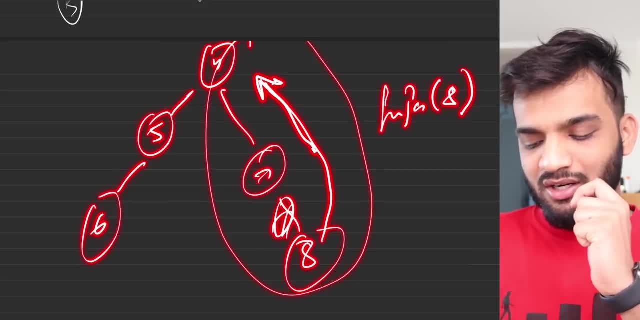 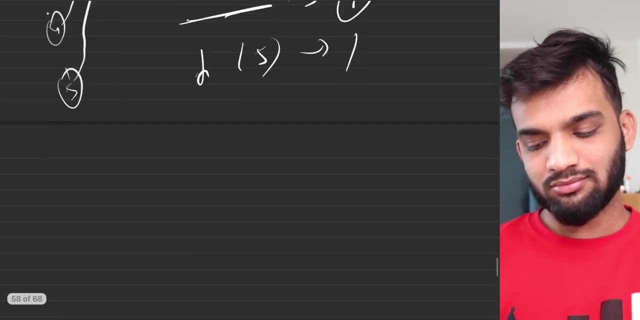 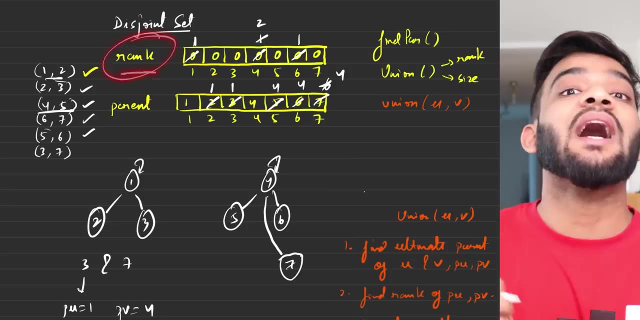 path compressed, see you, reduced one section of the tree, but the other section is still having a bigger length. so the rank cannot be- uh, cannot be- reduced. so that's why we call it as a rank and not height. if we can reduce it, we would have called it as a height. but since 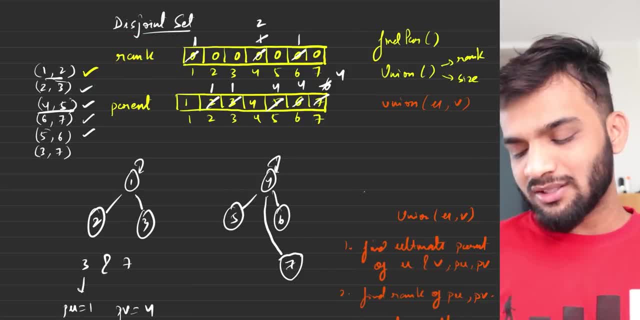 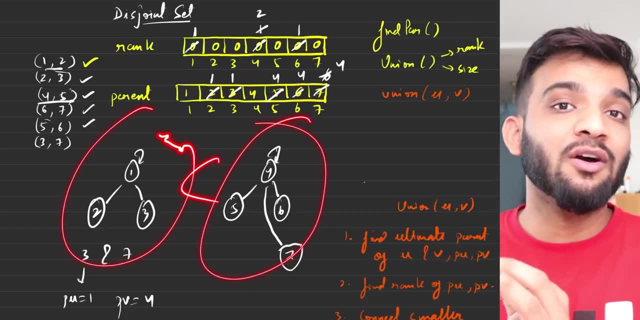 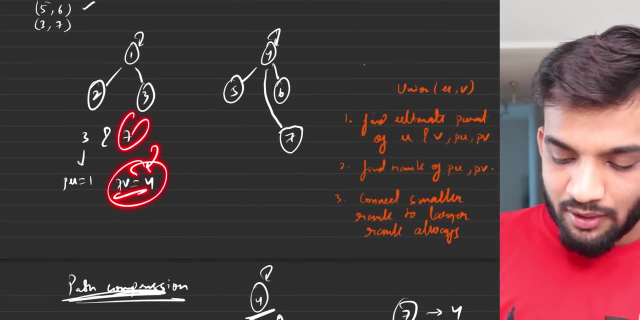 it cannot be reduced. we call it as a rank. rank in the sense means this guy is bigger than this guy. sorry, opposite: proximal guy is bigger than this guy. that's it. that's the meaning of rank. this guy is higher ranked than me, got it. so the moment you find the parent of seven to be four, i find the rank to be two, which means 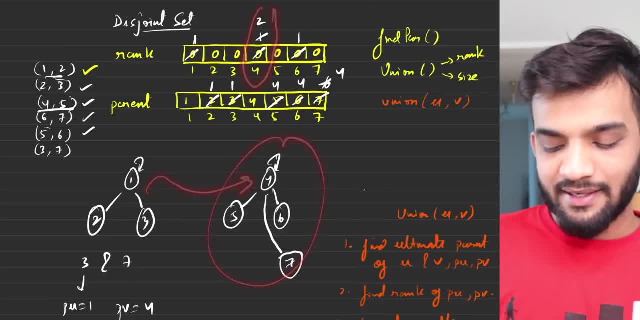 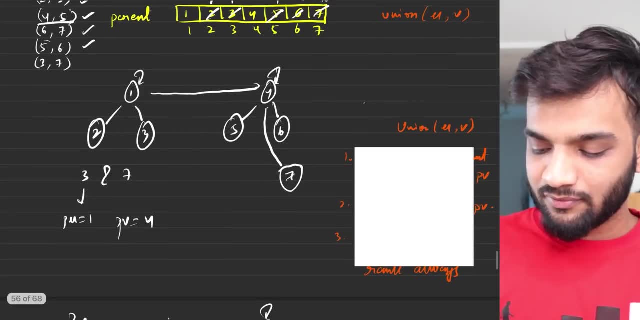 this is the bigger guy, so the smaller guy will this time come up and get attached to this guy. so what will happen is this guy will come up and get attached to this one, so ultimately we will have. so ultimately, what we will have is, uh, the parent of seven will be four, and i'll attach 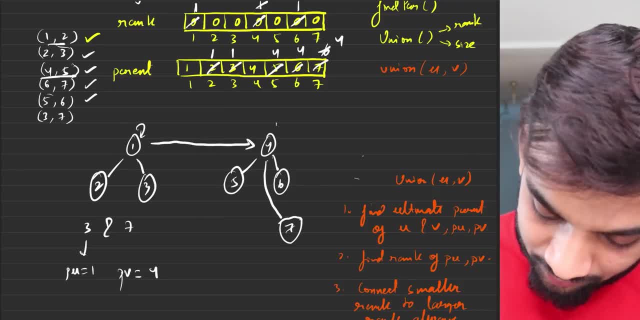 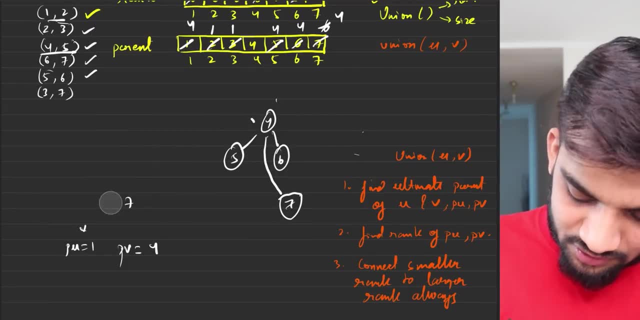 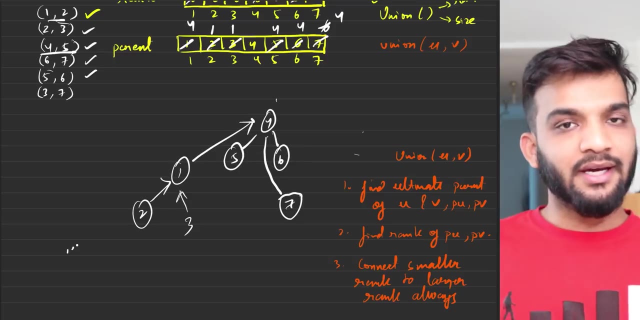 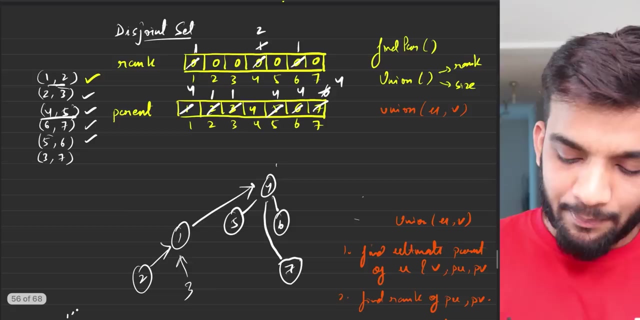 one to four. what will happen? the parent of one will now become four, correct? so if i just read: uh, draw it. it's going to look something like this: one attached here and two and three attached to this guy, correct? so will the rank change? no, it's still the larger guy. attaching the smaller to the larger guy will not impact. 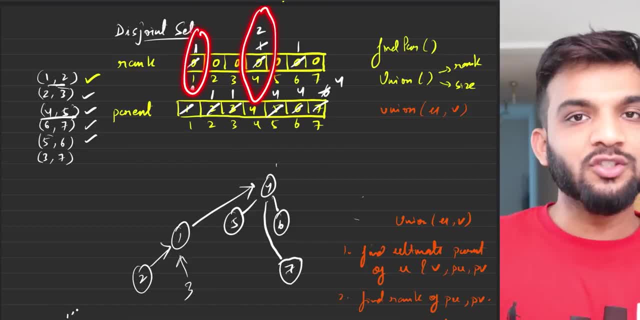 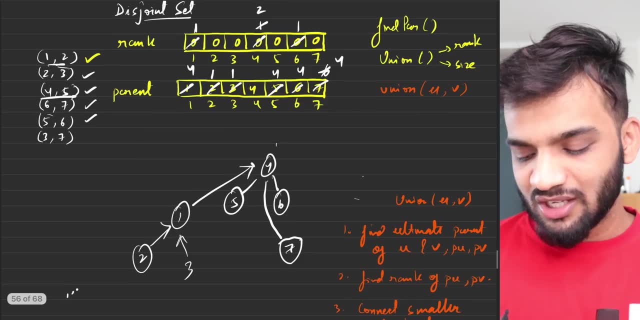 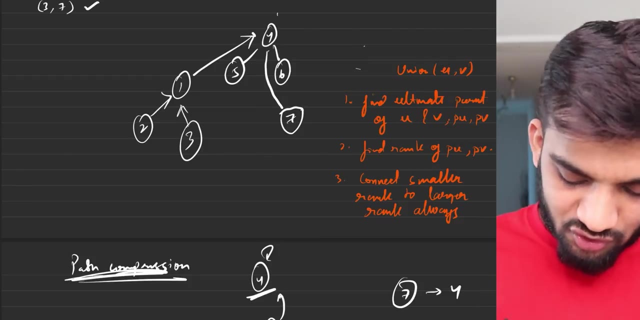 because the rank of one, if you remember, was one, the rank of four was two. so we are not storing the height because during path compression the height will shrink. so this is how easily we can do it now. if, after this, someone comes up and says: hey, uh, does three and 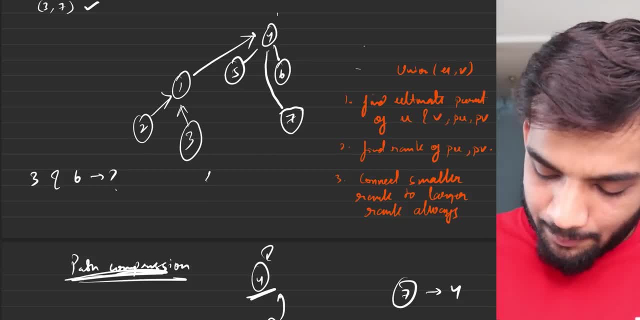 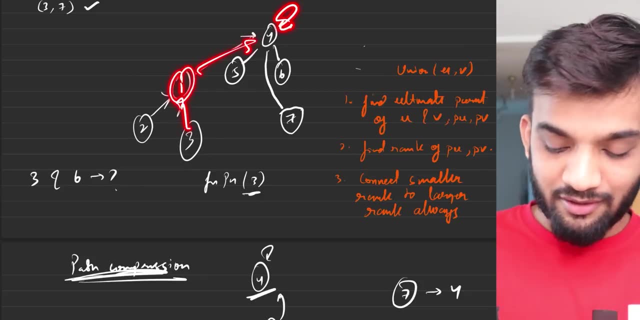 six belong to the same component. what you'll do? you'll call the find parent for three and it will find you, the parent to be ultimate, ultimate three, one, one, four for himself. so again, a path compression will happen. yes, when you find the parent, three will give you an. 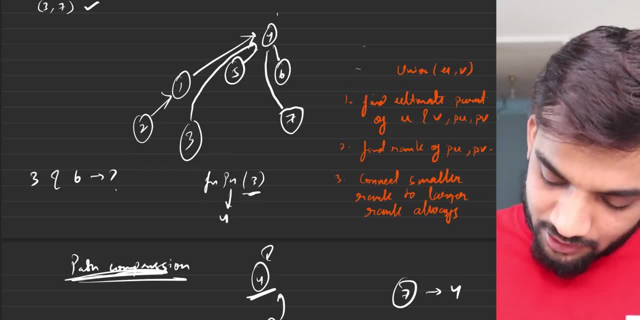 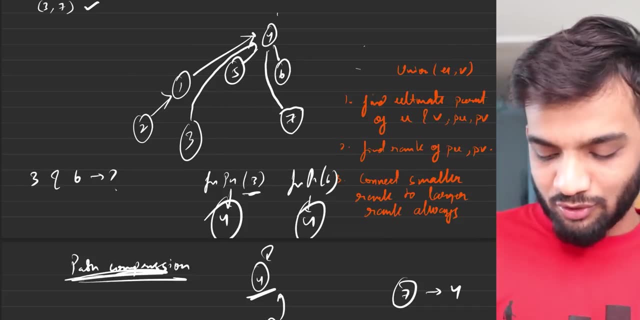 as four. so the path compression will also happen. fine parent of three will give you four. fine parent of six will be directly four, so both of them have same parent or ultimate parent, so they belong to the same form. quite easy, you, since you're compressing the tree, since you're compressing the. 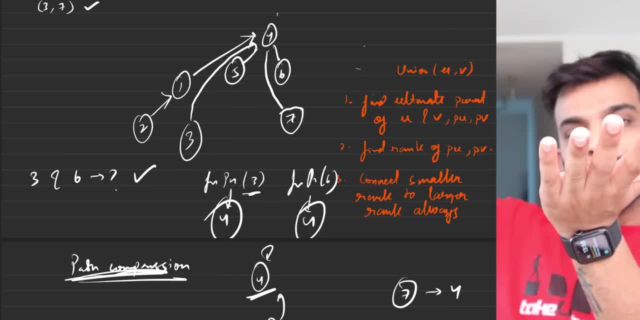 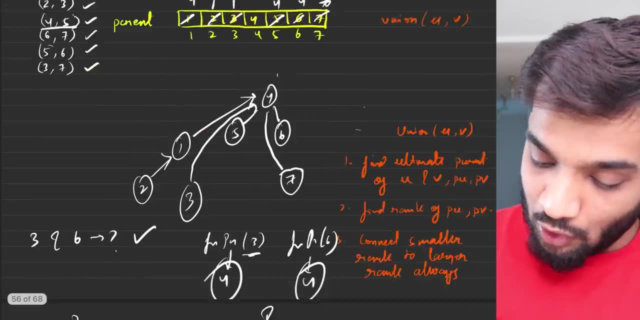 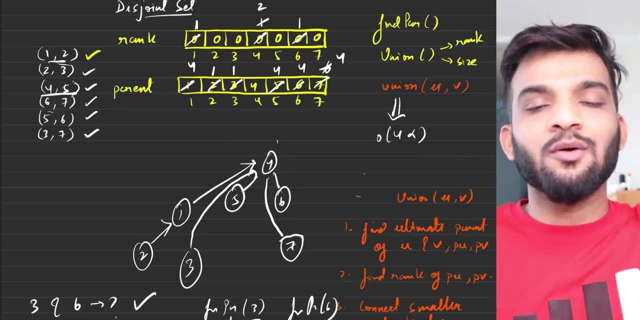 tree. the tree will be always a very limited size. in order to find parent you have to do limited traversals. always got it. so thereby the time complexity in order to perform the union operation is bigo of four alpha. now this four alpha has a huge mathematic derivation which is not required. 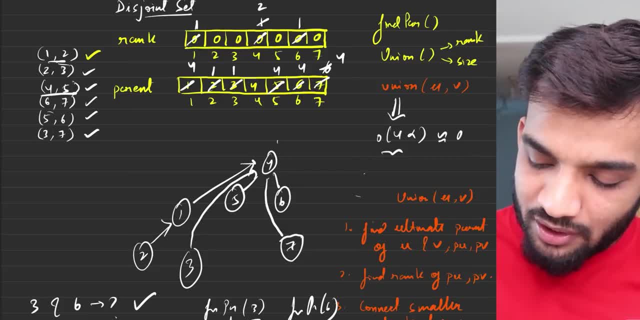 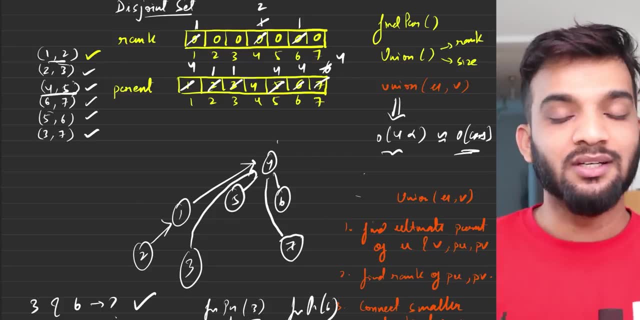 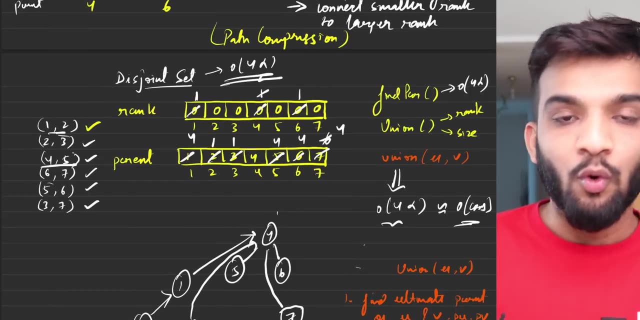 in interviews you can say four alpha, which is as good as constant, because the alpha's value is very, very close to one, that is as good as a constant. and in order to find parent, it is also four alpha. so overall, the data structure works in bigo of four alpha. remember this, okay. so the question: 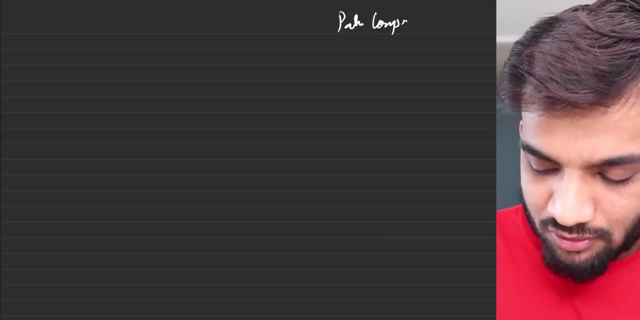 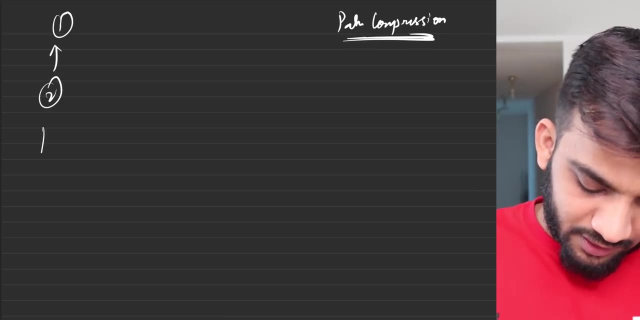 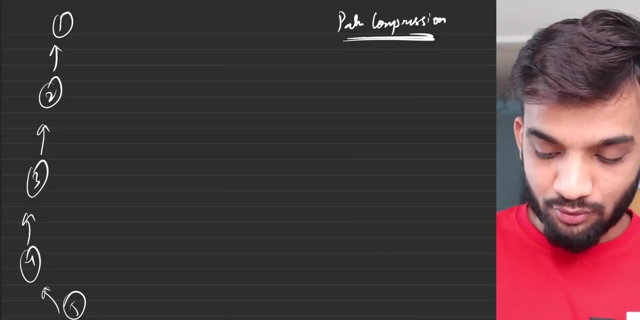 comes up. what's driver? how do we do path compression? you might be thinking: how do you do path compression? because it looks scary, because if you are connected to this, then you're connected to this, then you're connected to this, then you're connected to this. how do you path compress it? it's very simple, so. 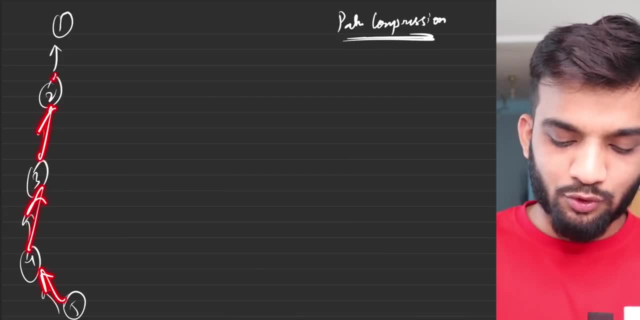 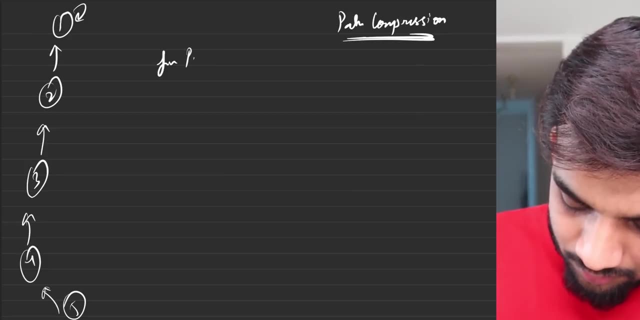 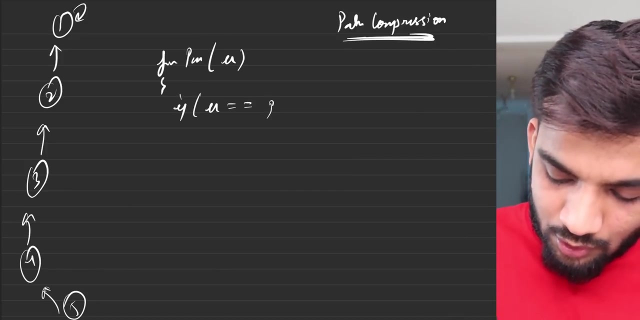 five's parent is four, four's parent is three, three's parent is two, two's parent is one and one's parent is one. so what you can do is you can backtrack so you can write something as find, and what will happen is you will say: if u is equal to equal to parent of u. 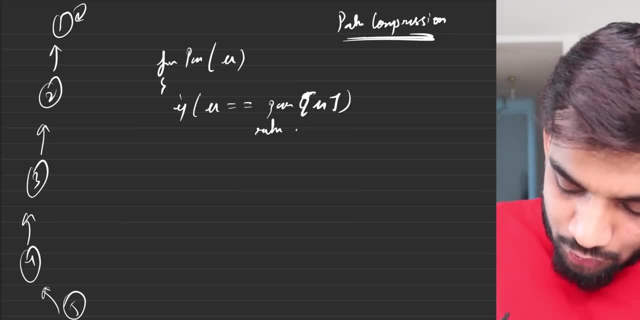 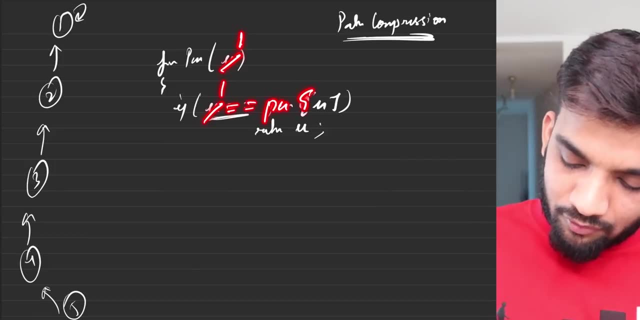 then return this u. so, basically, what does this mean? if at any moment one comes, one will be equal to equal to parent of one, because parent of one is himself. they'll return the parent as one. that's the base case, because that is where you stop. otherwise you will be like: can you please return? 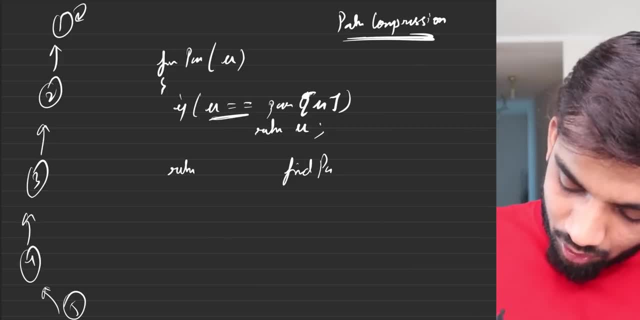 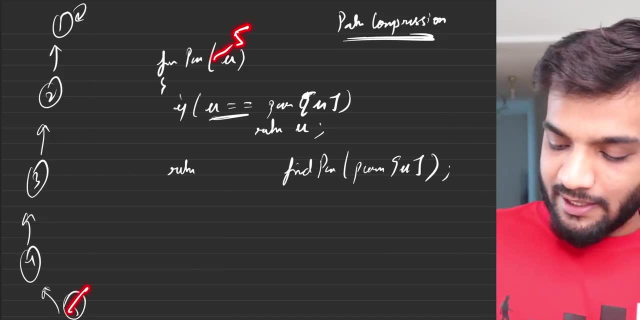 find parent of parent of you. what does this mean? imagine i give you five. what will happen? it will go and say: parent of five. what's parent of five, four? we'll go and say: find parent of four. so the next time find parent of four will happen- does not obey. again. it will say: find parent of parent of four is parent. 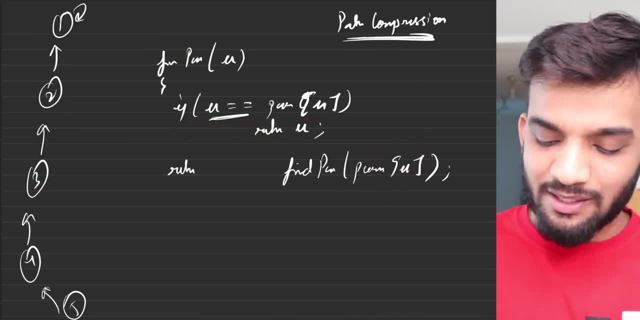 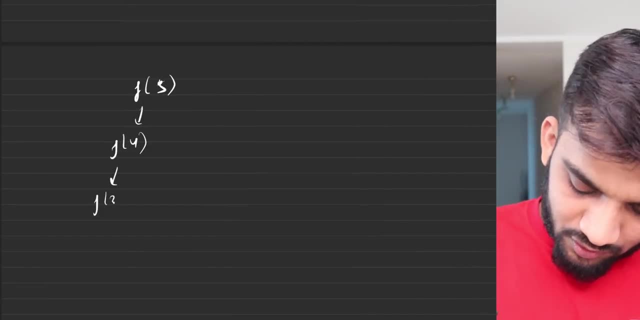 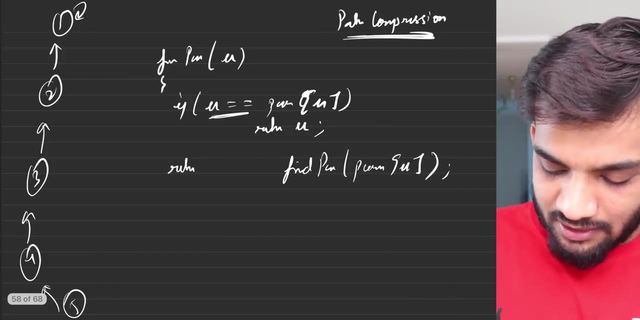 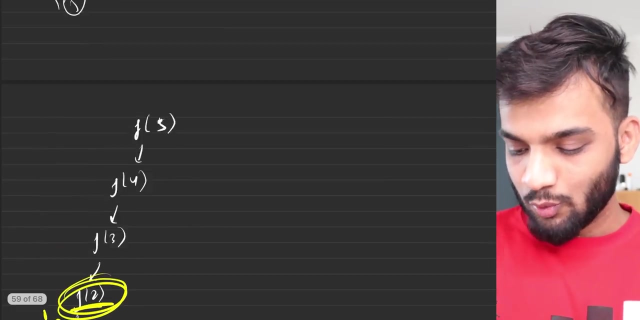 of four, three, so it'll go on. so the recursion will be something like this: function of five calls, function of four calls, function of three calls, function of two calls, function of one at one, the base case is executed, and when it is executed, it returns one. so this two which called, which you would have called here, what you'll do is you'll say: 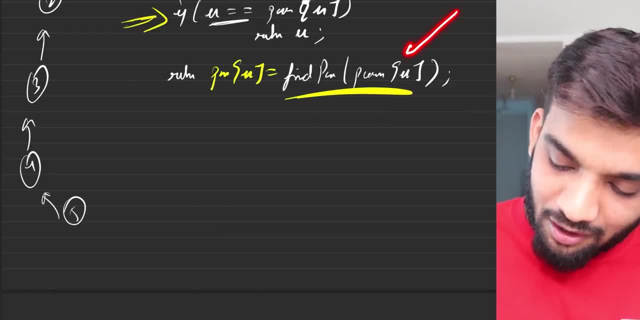 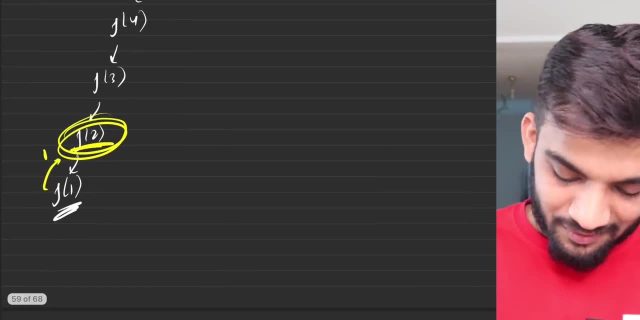 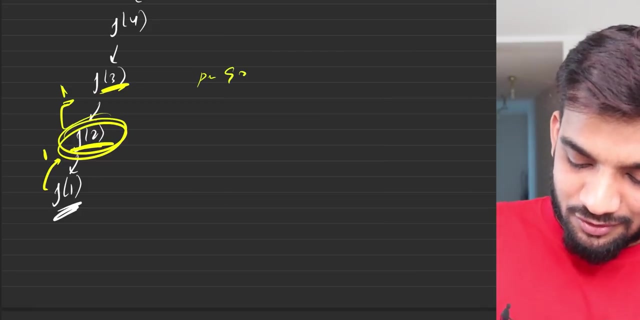 parent of you will be two. so when it will return of, it will return with one. you'll say: hey up, one, keep it right, keep it one. next you will again return one, you'll again return one, and then you'll one. so now three will also keep one. parent of three is one. next you'll all also return one. so 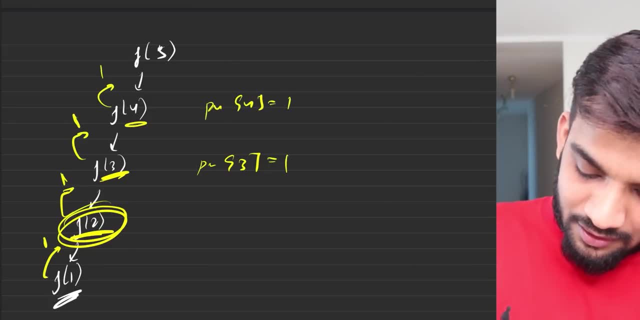 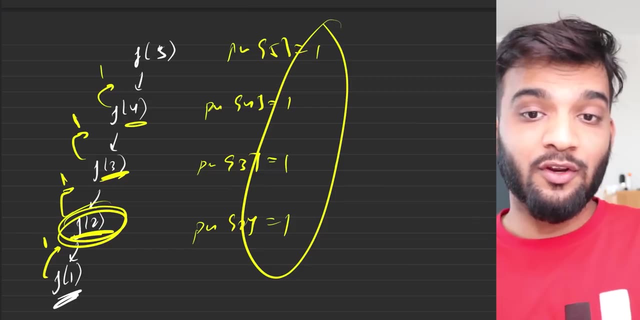 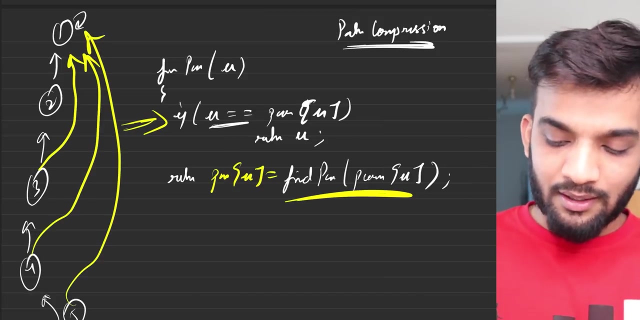 now parent of four will also be one. next you'll also return one, so parent of five is equal to one. so everyone in term will assign one to it in. if everyone assigns one to it, so automatically all the links will be path compressed and pointing to one and and all these links will be destroyed. 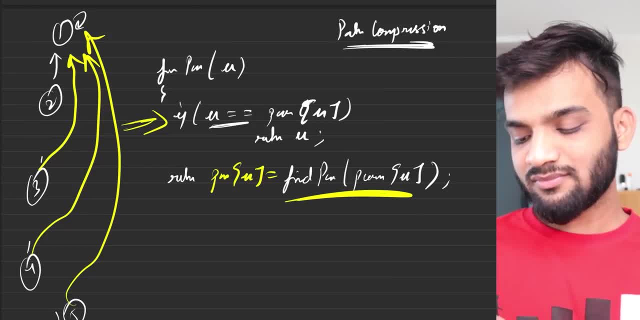 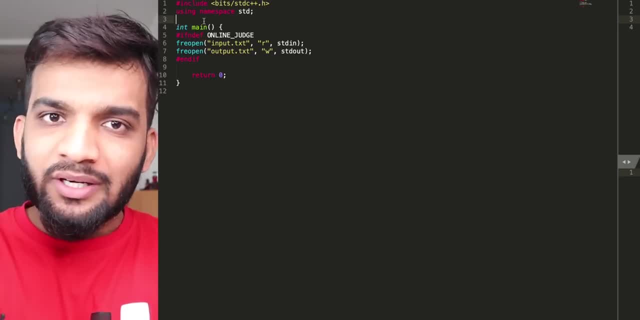 perfect. done so, i hope you have understood everything about the union by rank and the path compression. now it's time to code it up, so i'll try to create the data structure in a class so that going forward, in the upcoming problems, we can use that snippet of code to solve. 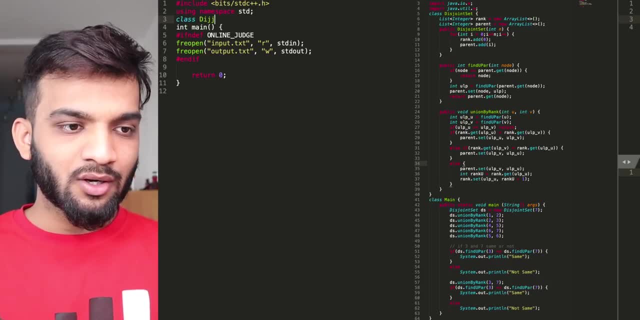 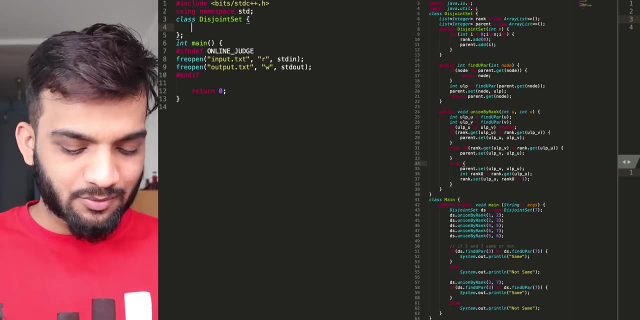 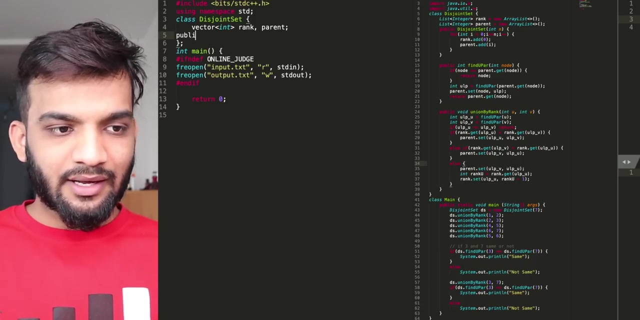 almost all the problems. so we have a class of- uh, disjoint set. nothing to worry like. don't, don't get worried about a class. very simple, it's a very simple thing. what's the initial configuration? you initial configuration required a rank and a parent. we'll just have it and declare everything. 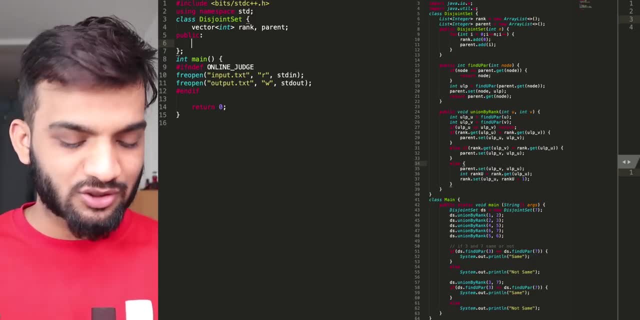 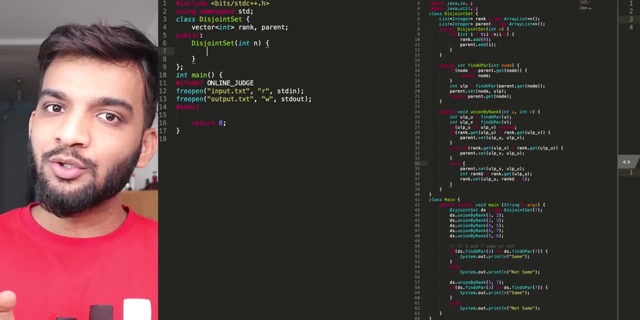 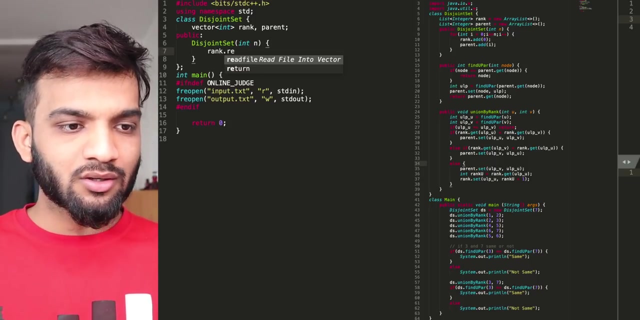 afterwards public, so all the functions can be reused outside. so now go ahead and declare the constructor. what is the construction? uh, what is the constructor? rather so, if you remember, i said you initially: rank will be marked with zeros, parent will be marked with themselves. that is what we do. so we say: rank dot, resize of n plus one comma, zero, y, n plus one, imagine it's a one. 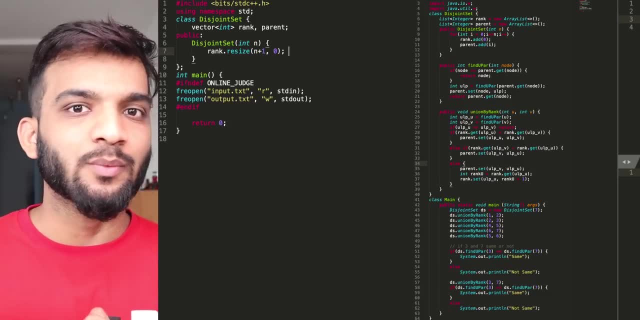 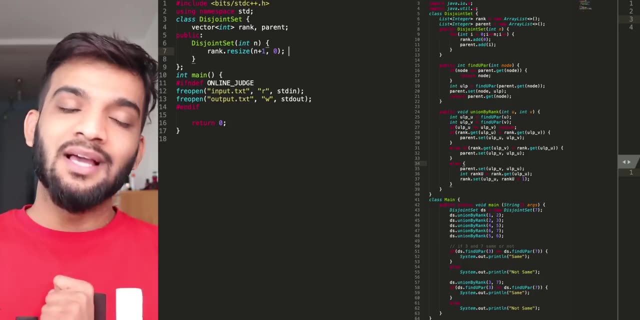 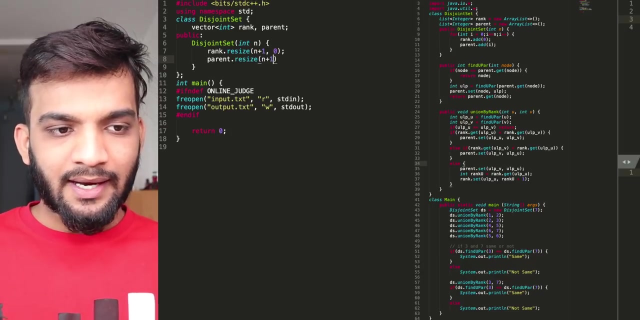 indexing graph, we need the nth index as well. if it's a zero based, fine, but declaring, uh, declaring it as one n plus one will work for both one based as well as zero based. similarly, we can define parent dot resize of n plus one and we can keep it, and then we can go ahead from zero- very, very important- to go till n, for. 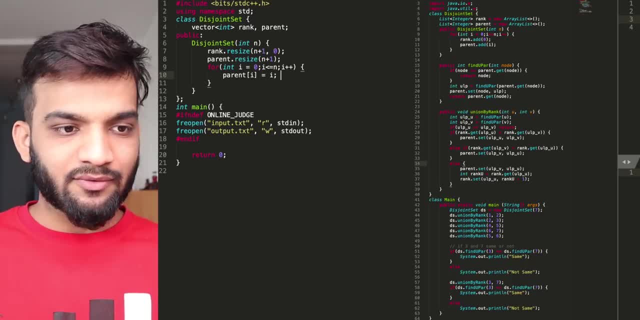 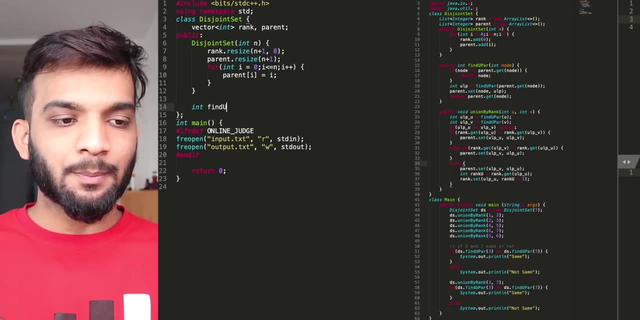 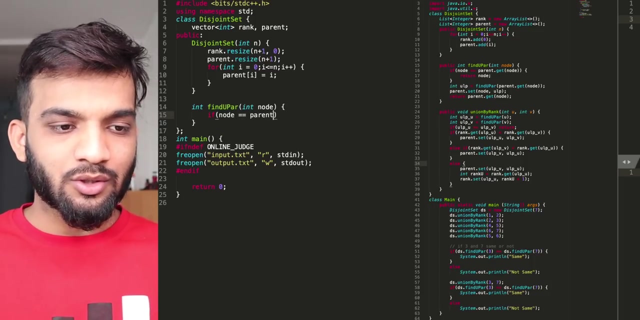 one base indexing, and it'll be i itself. so this is how the constructor will look like. now, what does disjoint set give you? it gave you: find ultimate parent, right. so this will be the node, and for this you have to find the ultimate parent. so we know one thing: if node is equal to equal to the parent of node, this is 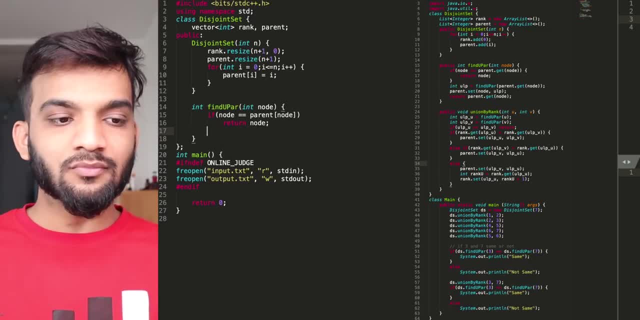 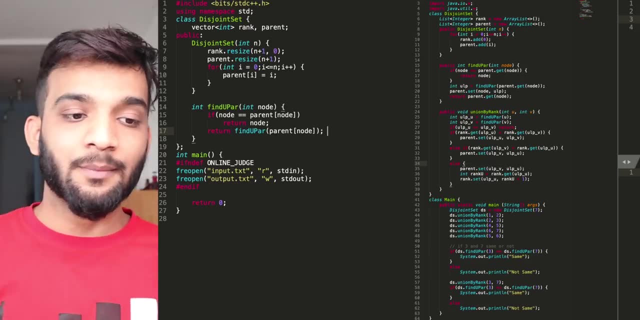 the ultimate parent for sure. so you go ahead and return the node, but if it is not, then you call the ultimate parent and say: go to its parent, and then look for parent, parent, parent, parent. but this is the normal logarithmic guy. we need the path compression. so this is where i can say whenever: 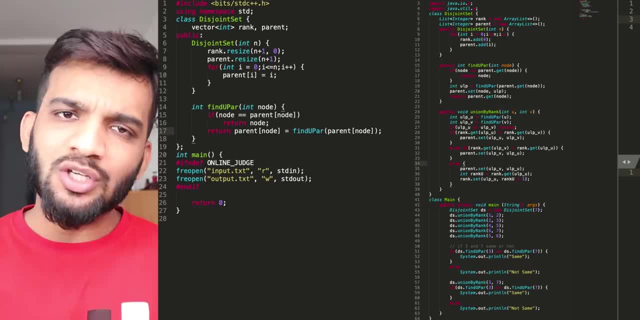 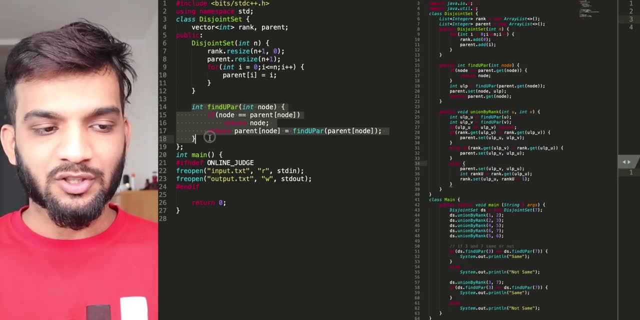 it returns the value. i'll store it so that in future, if someone comes up and does ask me the same question, i can tell him that this is the parent. so this is where the path compression comes in. path compression done next, what i'll do is i'll be like: okay, void union by rank is what i need. to implement union by rank. so i'll have node u and node v which i have to combine. so ultimate parent of, i guess the ultimate parent of you will be find ultimate parent of you. similarly you can say: ultimate parent of v will be find ultimate parent of v. now i can say: if ultimate of u is equal to: 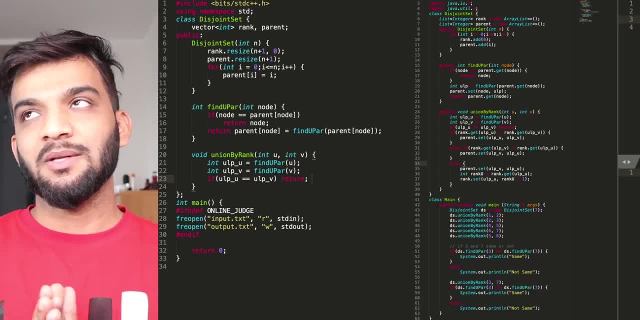 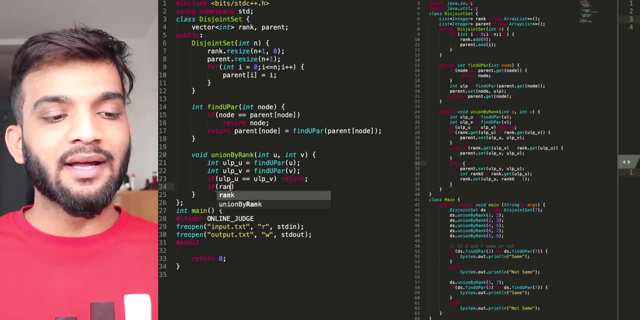 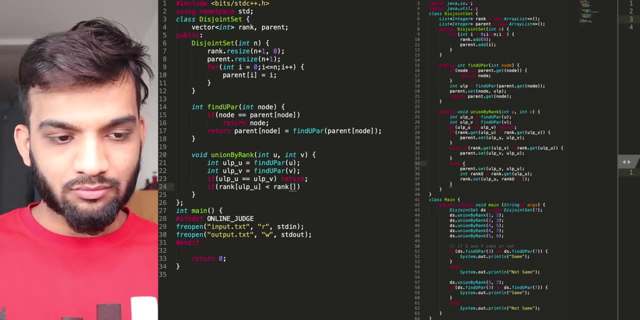 equal to ultimate of v. i can simply return. what does this mean? if they're belonging to the same component, i don't need right, but if they're not belonging to the same component, i go ahead. the first thing i do is i check if the guy u is smaller than the guy v, right? so 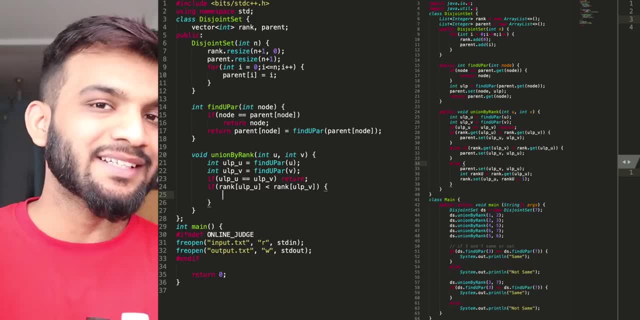 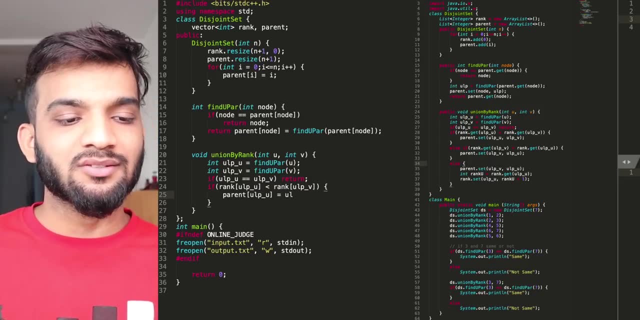 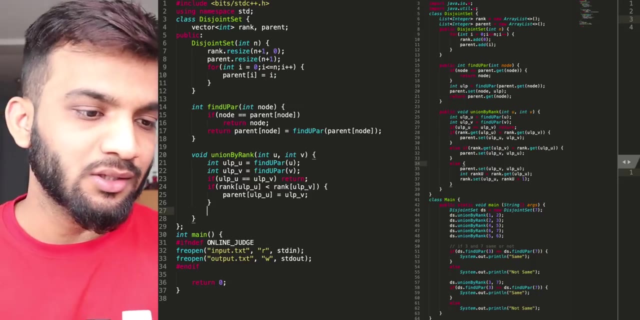 if v is the greater guy, the smaller goes and gets attached to the greater guy. so the smaller will now say: okay, i'll go and have the parent as v, no change in rank, because if a smaller guy gets attached to the larger one there will be no increase or that still. 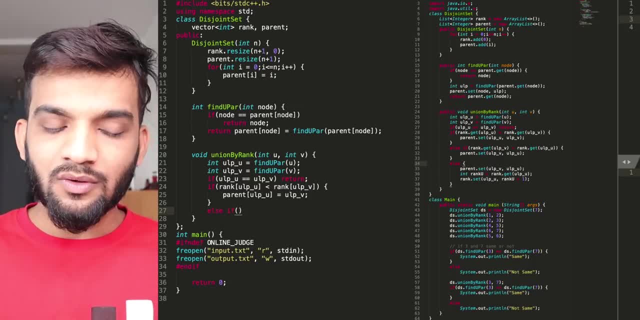 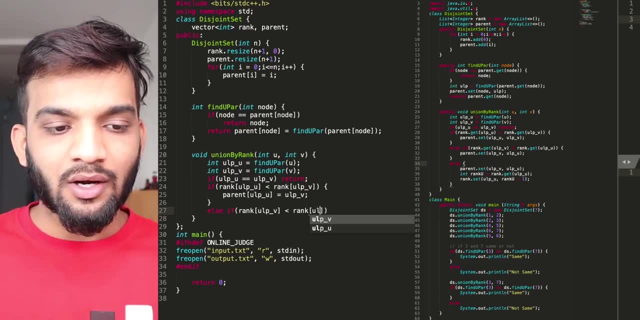 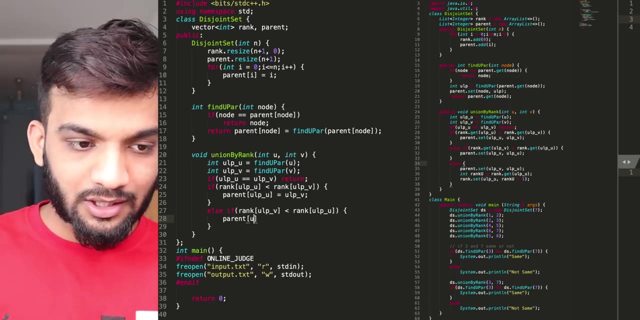 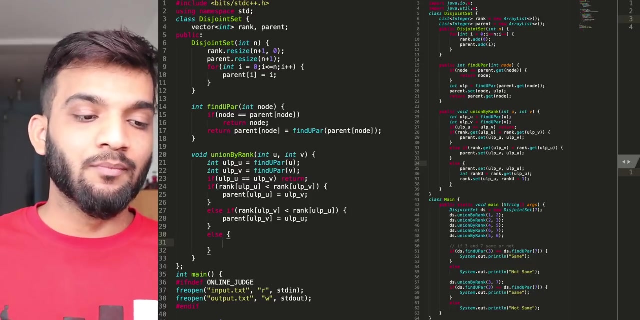 stays the larger right. next else, rank of ultimate of v. if this is the lesser guy, rank of ultimate of u. if this is the lesser guy, then i say the opposite. i say parent of rank- sorry, parent of ultimate of v- goes and gets attached to you. perfect done. but if what? if they are same, if 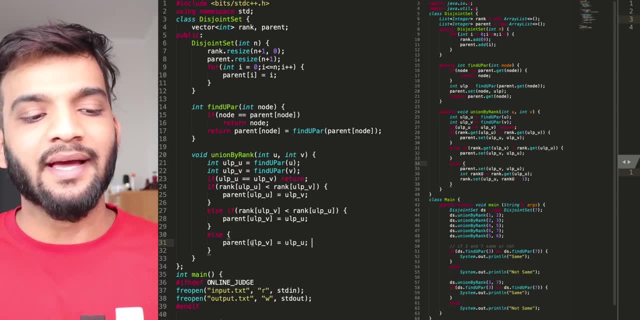 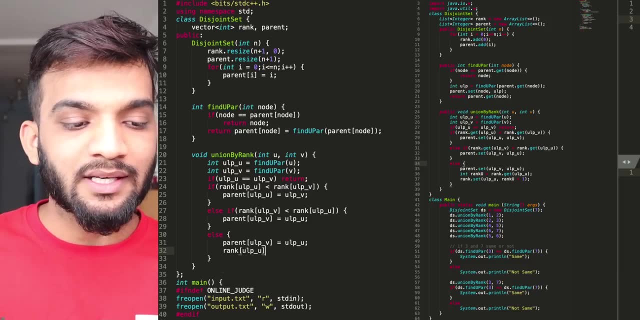 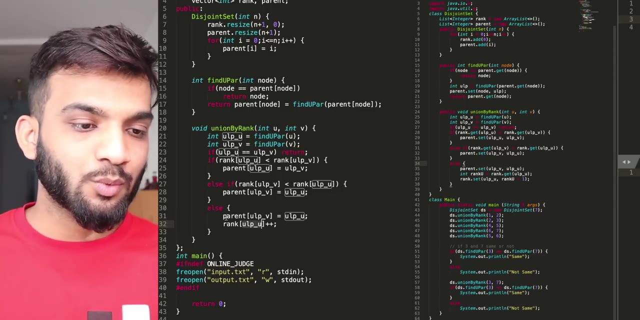 they're same. i'll self attach v to u. you can do the other way as well. u to v is okay as well, and rank of ultimate of u will increase because that is where i am attaching it to v attached to u. so rank of ultimate of v is okay and rank of ultimate of v is okay and rank of ultimate of v is okay. 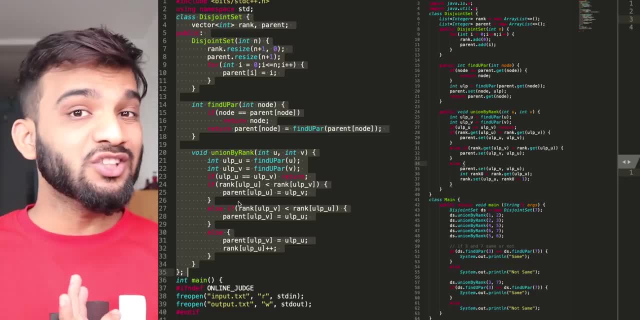 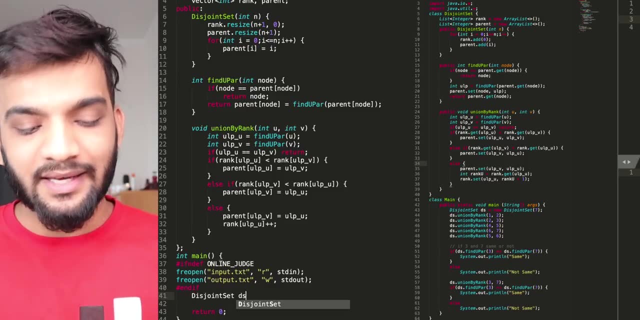 this is how our data structure will look like. how can we use this snippet of code? so i'll just hard code it to show you how can we use it. it's pretty simple. so you can be like: disjoint, set ds- what is the number of nodes? so in our case it was one, so i can have it as disjoint. 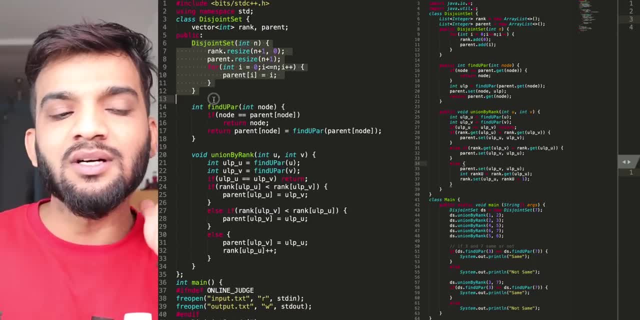 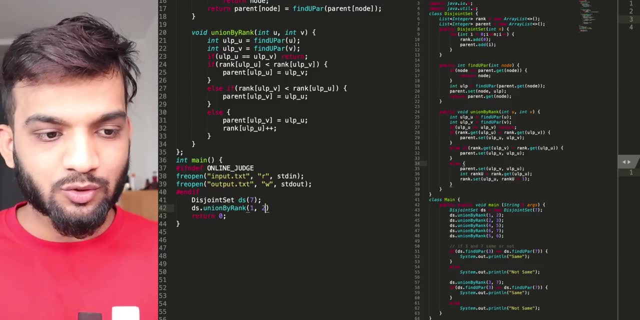 set of seven. so it will call this constructor and have the initial configuration ready for us. next will be, i'll call it, the union by rank, and the first thing was one comma two, if you remember in our example right. so we'll have it one comma two. 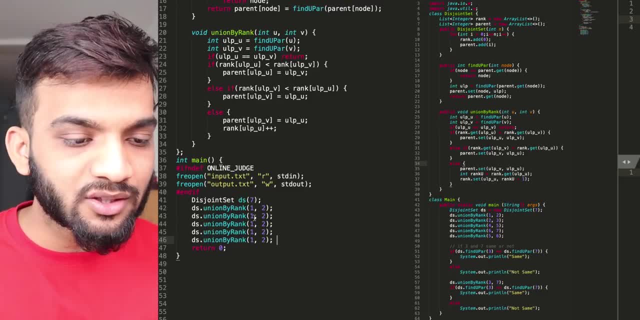 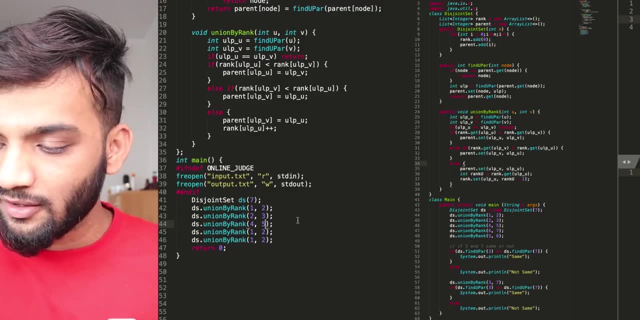 so i'll quickly add all these uh things. so next was two comma three, if you remember. let's add two comma three. next was uh, four comma five. so let's add four comma five. next was six comma seven. let's add six comma seven. next was five comma six. let's add five comma six. 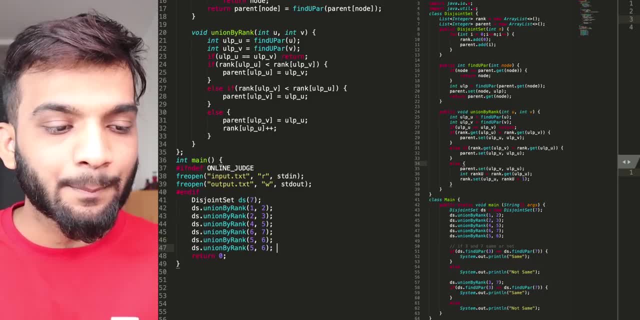 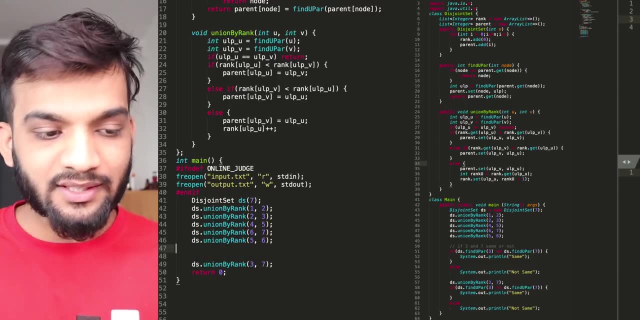 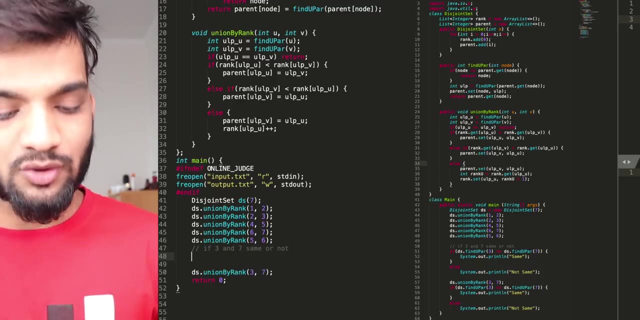 and the next was, if you remember well enough from the example, the next was three comma seven. so i'll be adding up this. but before adding up three comma seven, let's quickly check if three and seven belong to the same component or not. same or not? okay, so what i'll do is i'll call the find ultimate parent for. 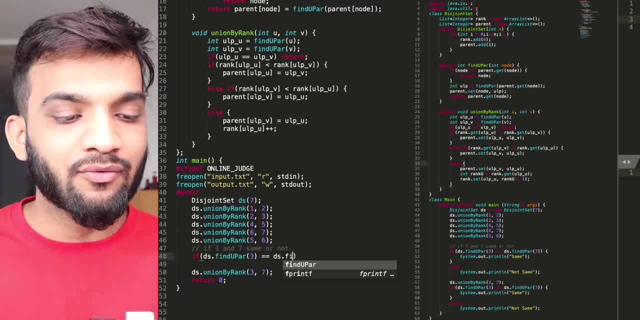 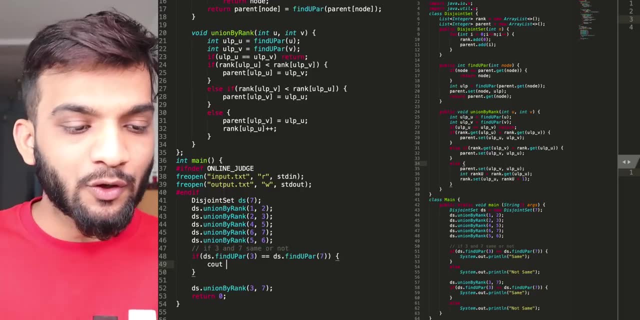 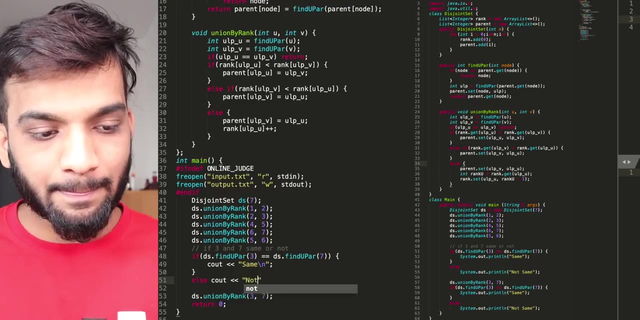 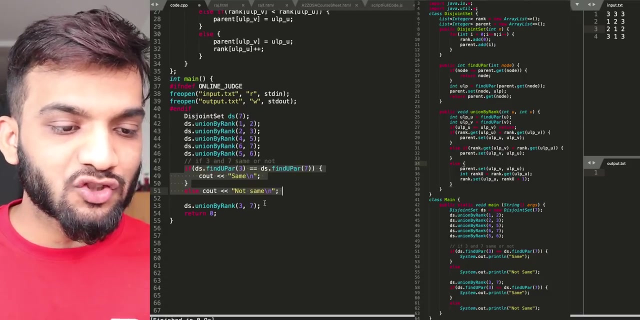 three and i will say: okay, do you have equal to equal to seven? like, do you belong to the same? like, do you have the same boss, same ultimate parent? if you do, then same as the same, or else i will say not same. i'll go and say not same, right, perfect done. and after connecting them i will again check. 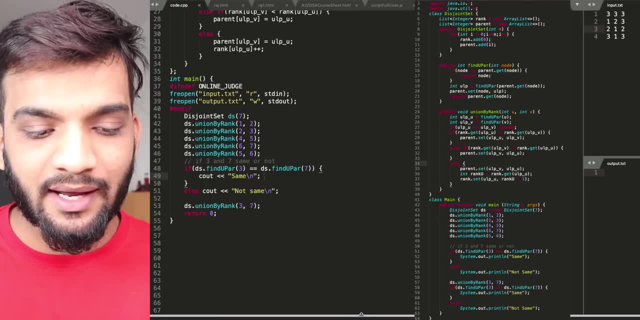 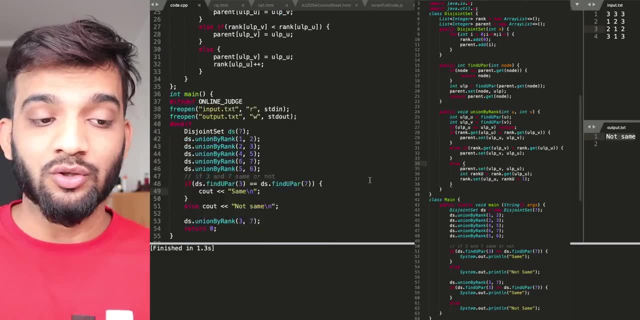 for the same. so as of now, let's uh have a quick run and see if it is giving us correct answer. so i'll just go and compile this. so on compiling, it is saying no, they do not belong to the same. and if i go ahead and move it to the next guy, it will actually say 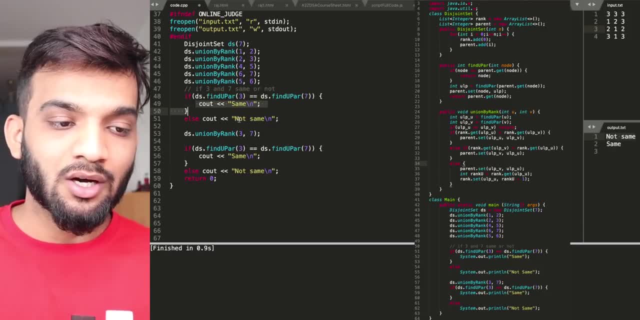 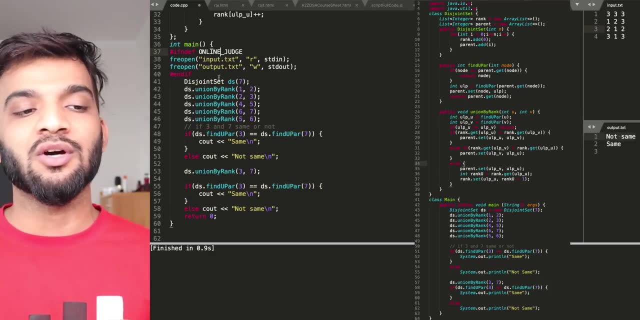 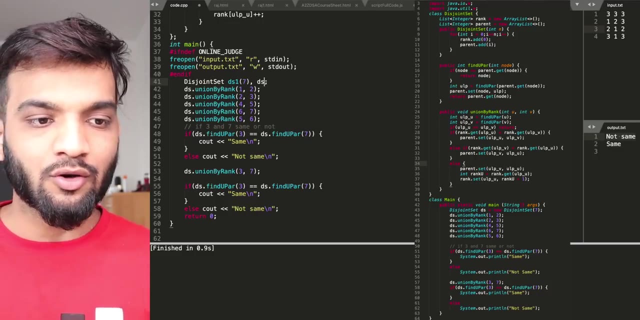 that they belong to the same. see: first time it says uh, not same. then on combining, it says same. so this is how you can always use the data structure. if you want to have two disjoint set data structure, you can go as ds1. you can have two different objects of this class and you can have 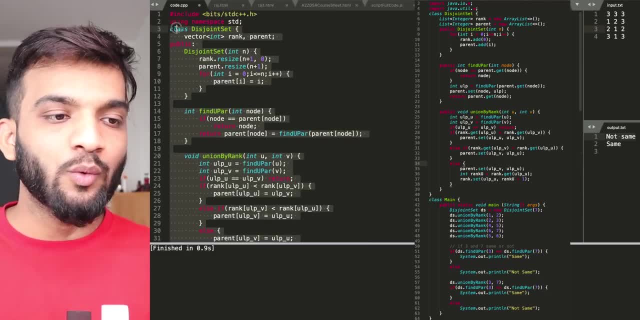 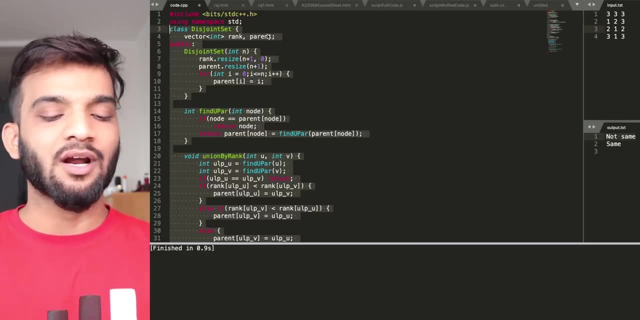 two different graphs in two different data structures. so this code can always be reused in almost all the problems, because it covers up zero based indexing graphs as well as one based indexing graphs. now a question might be coming to your head, but striver. we did not understand why. 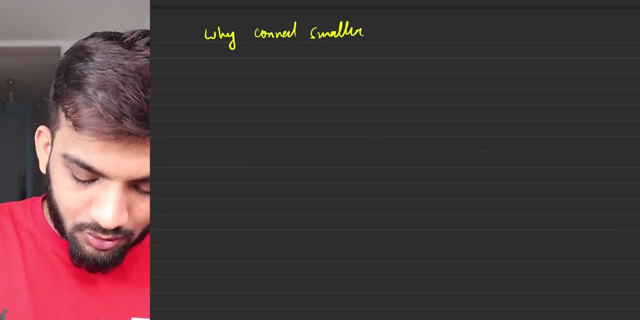 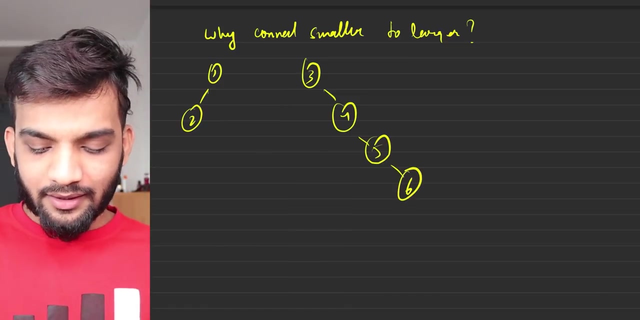 connect smaller to larger, like. what's the idea of connecting smaller to larger? the first idea is: i don't want to increase the height. for an example, if i have one, two, i have a three, four, five, just for an example, empty. so if i connect the larger to the smaller, see what will happen: one, two, three. 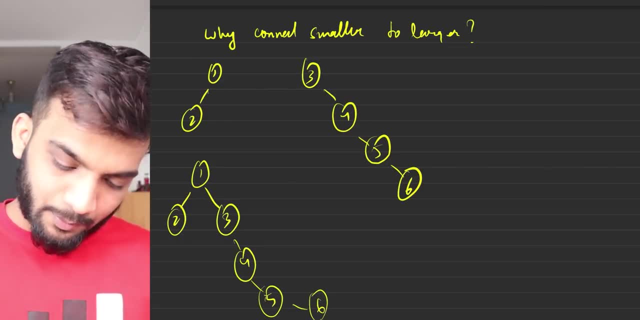 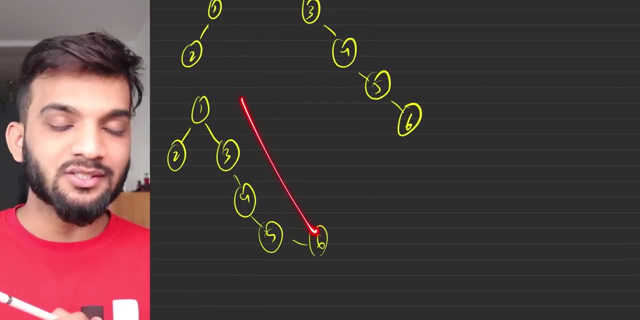 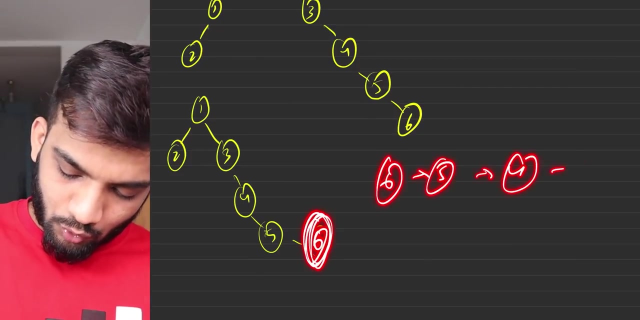 four, five, six. so basically the height increases. and if the height increases, like we will do, path compression for sure. but if the height increases, what happens is now, in order to find the parent of six, we'll have to travel six, five, four, three and then one. so we're taking 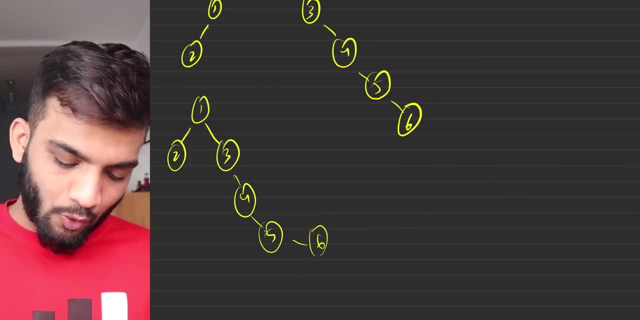 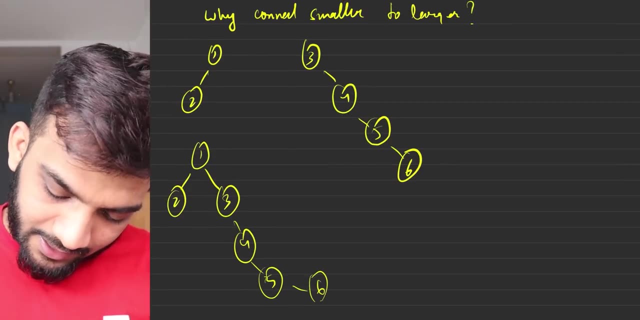 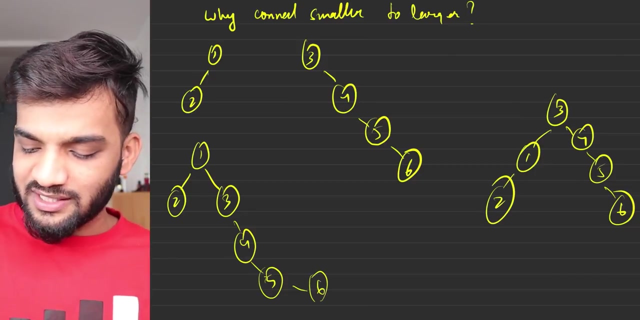 a longer distance. so imagine someone would have said for four, so you're actually taking a longer distance. and if you do the opposite way, which is saying let's connect like you keep three, four, five, six and let's connect one and two, so if you see for. 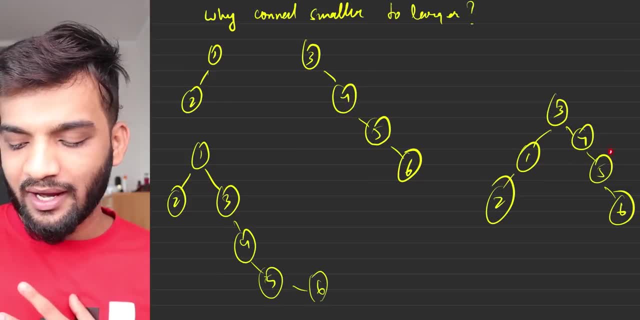 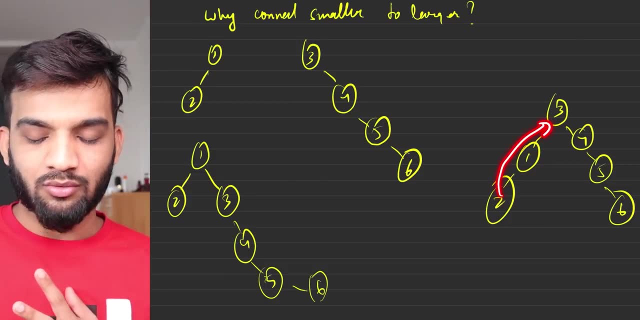 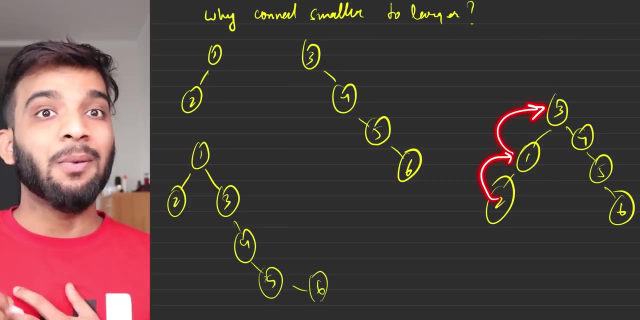 the distance taken is shorter. even for 5 the distance taken is shorter. even for 4 the distance taken is shorter, but for these the distance will increase. like for 2, the distance will be now more, because over here 2 was just traveling once and getting the ultimate, but over here it has to travel to 1, then to 3, but 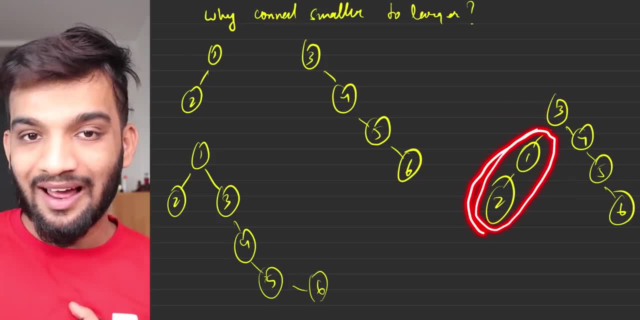 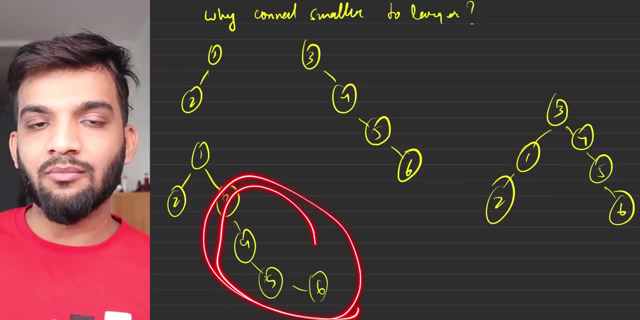 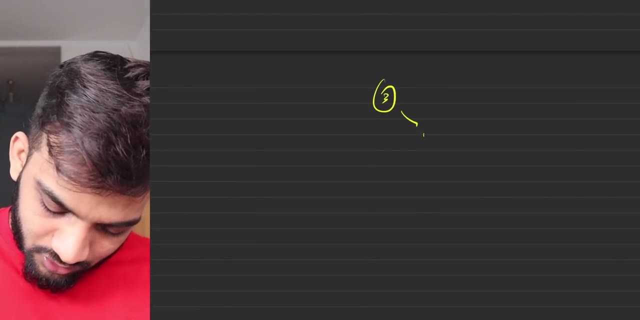 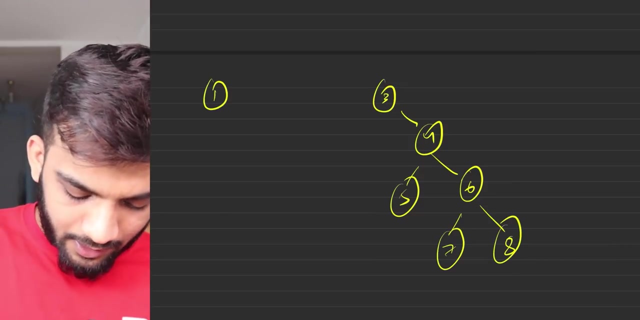 the number of nodes over here are lesser, so the travel time for all the nodes computed will be lesser. over here the number of nodes are larger, the travel time for all the nodes will be larger. so to give you a clear vision, imagine we had something like this. imagine 5, 6, 7, 8, okay, and we had 1, 2 now. 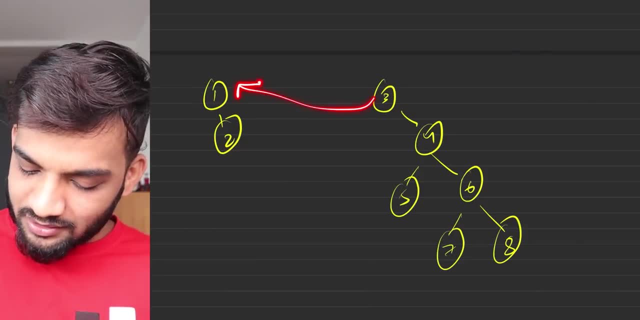 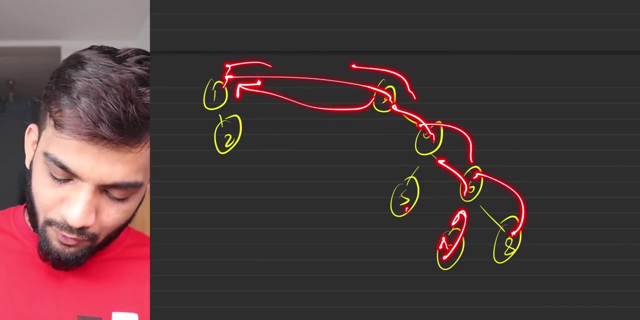 if you attach this guy to this guy, what will happen is, in order to find the parent of 7, 7 will go to 6 to 4. 3 to 1. similarly for 8. 6, 4, 3, 1 similarly for 5. 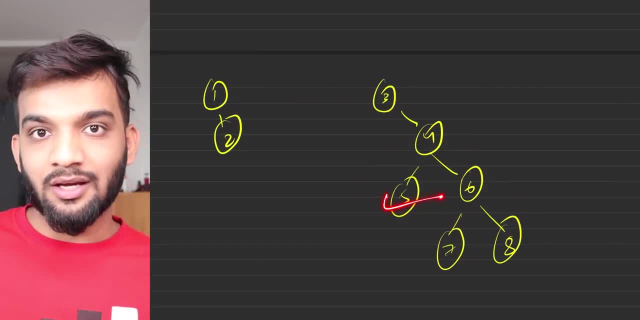 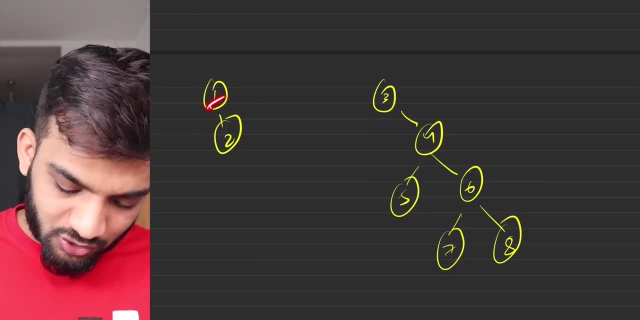 4, 3, 1. right, so this will take longer time. this will take longer time. this will take longer time. more nodes will take longer time, whereas if you attach this to this, they will take the similar time that they were taking and only two nodes will take slightly longer. 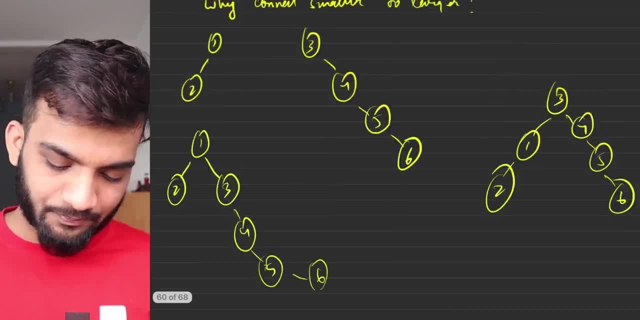 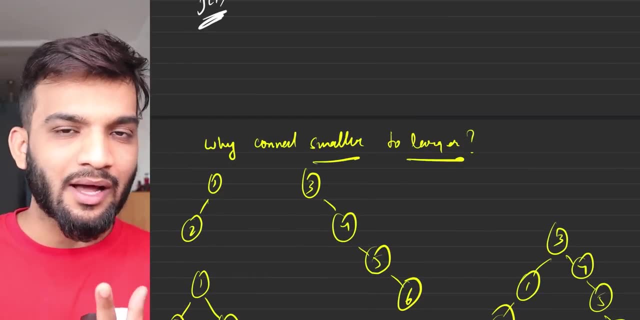 time, which is okay. this is the reason we attach smaller to larger. first, to keep it shrink. second is to make sure that the time taken in our finding of the parents is as minimal as possible. so you must be thinking, striver. if that's the case, why are we? 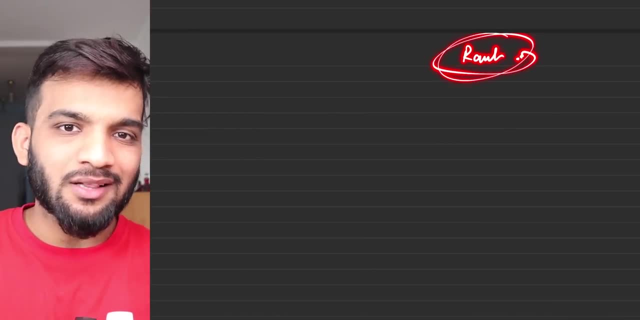 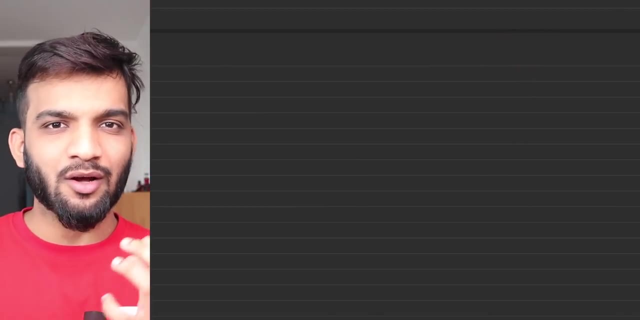 using something like union by rank, because after path compression it doesn't even gives us the height, because the height is distorted after path compression. can we use something, a size, which keeps a track of what is the size of the component? I think we can. I think we can, so that's what we will be doing. 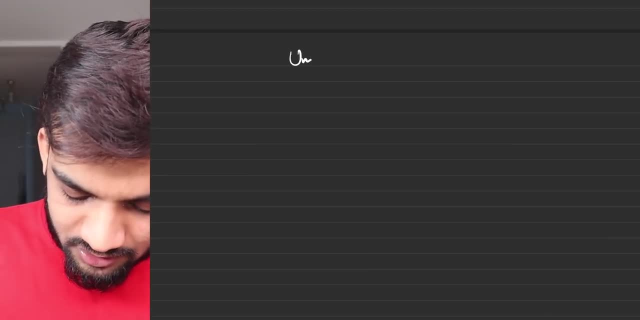 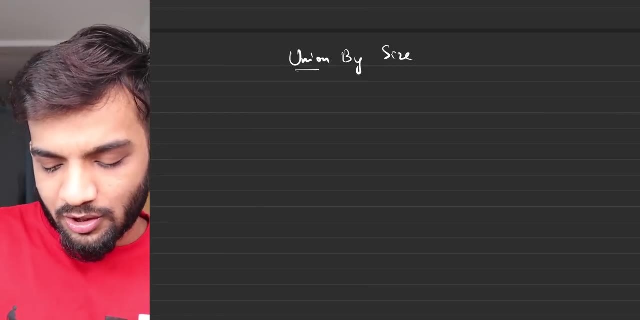 okay so? so what I will try to teach you now is union by size. we know find parent, we know path compression, but instead of rank we will be using the union by size. so over here, the same thing will happen: we will have a size array of the same size. so let's 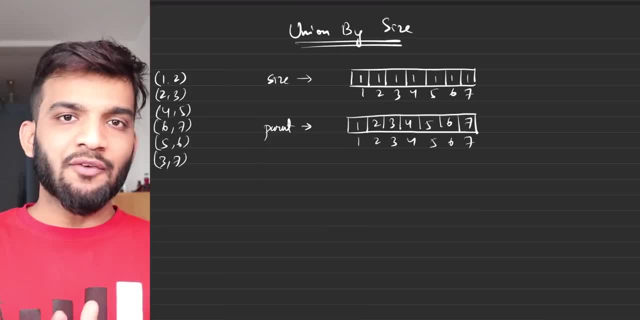 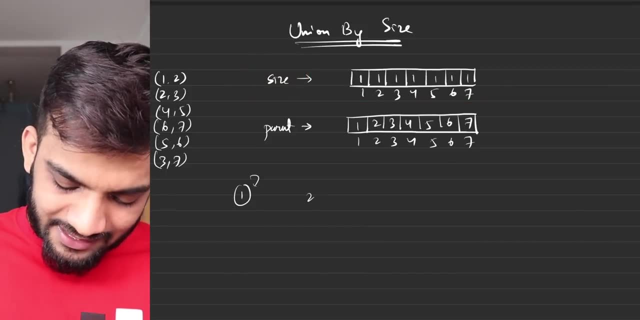 quickly declare the size array of seven sizes, so the initial configuration will be very straightforward: we will have a size and everyone will be of size one. why? because everyone is itself a component when we start off with, so everyone is going to be having a size of one. 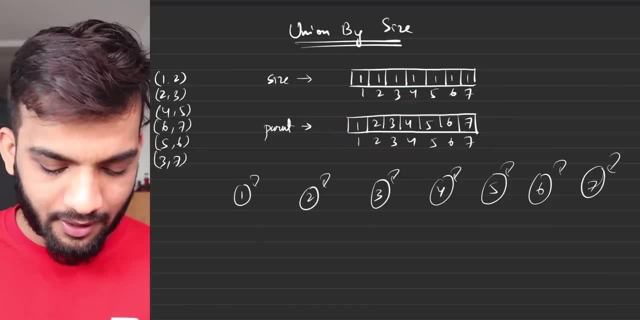 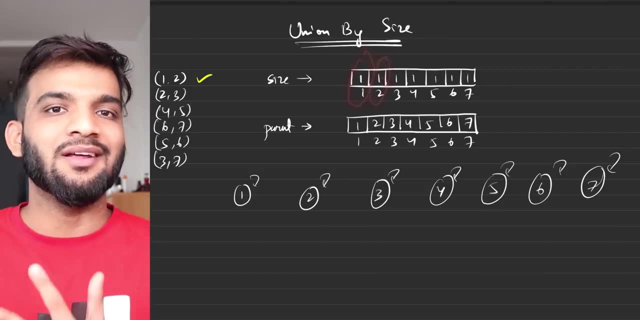 and we know one more thing: that the parent will be themselves. so this is what we take now to start off with, very simple. we say one comma two. we say one has a one, two also has a size of one. so both are similar size. so it doesn't matter whom you attach. so i go. 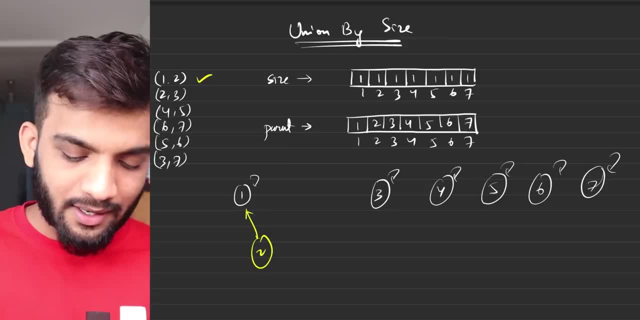 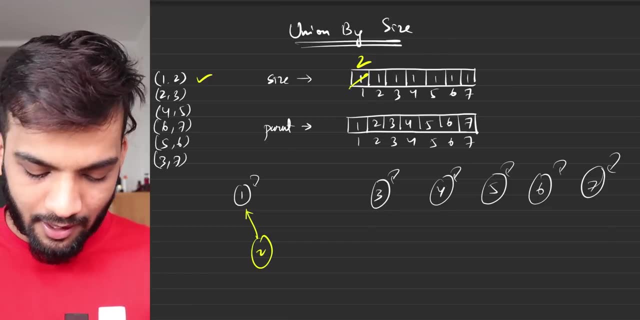 ahead and attach two over here. the moment you attach two to one, the size of one will increase to two, because it took a size of one, got attached to it, so the size increased by okay. next is two to three, very important point to realize: now one has a size of two and remember, the parent of two is 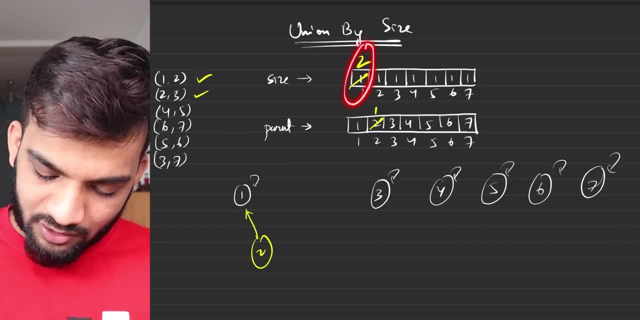 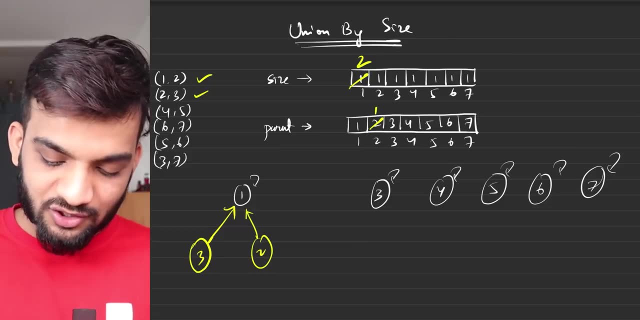 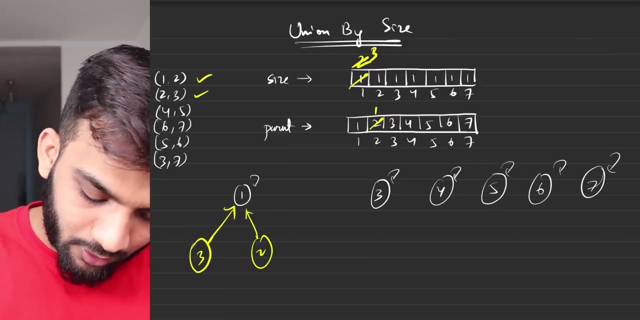 this time one. so one has a size of two and three has a size of one. so this is the smaller. goes and gets attached to one. so goes and gets attached to one. so the size will again increase by one. why? because three was a size of one, perfect done. and three will be having a parent of one. so this is 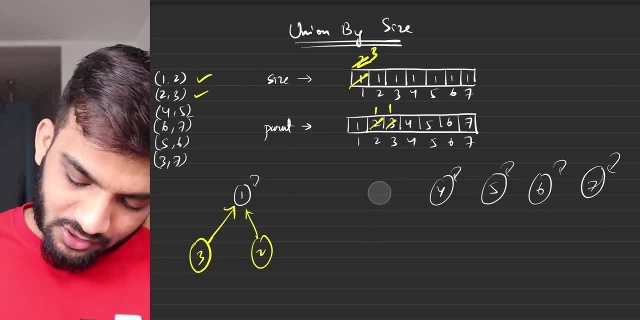 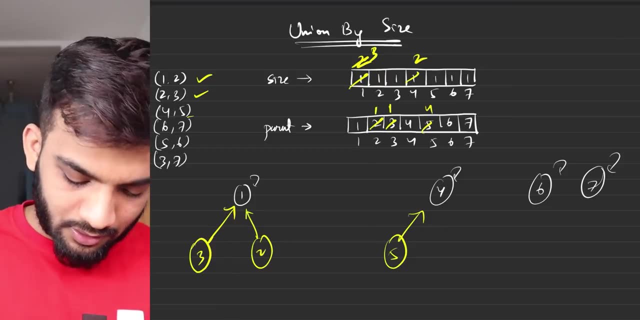 also done. next is four and five. so what i'll do is i'll just omit this and i'll just assign five to the sky, and five's parent will be four, and four will increase the size of two. next will be six and seven, so i'll assign over here, i'll assign seven's parent to six, and i'll 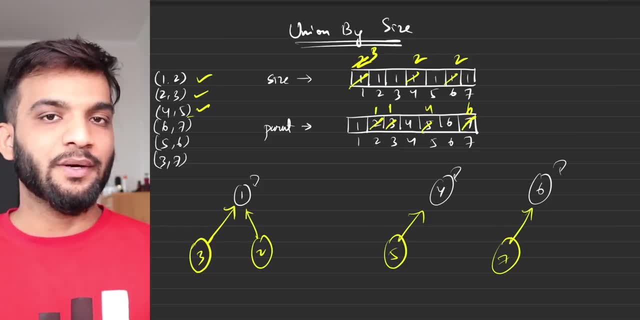 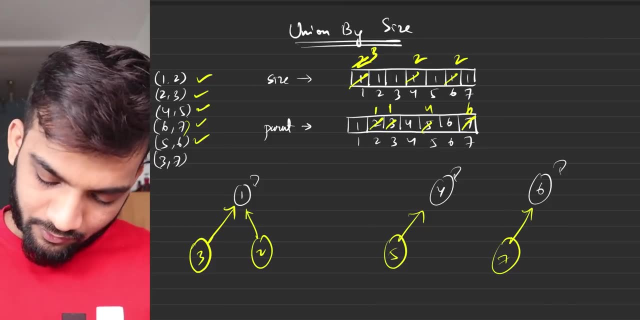 increase the size over here. perfect done. next is where you understand. so next is so 6 comma 7 is done. next is 5 comma 6. so where is 5? 5 is here with 4, and 6 is here, so both of them, if you see. 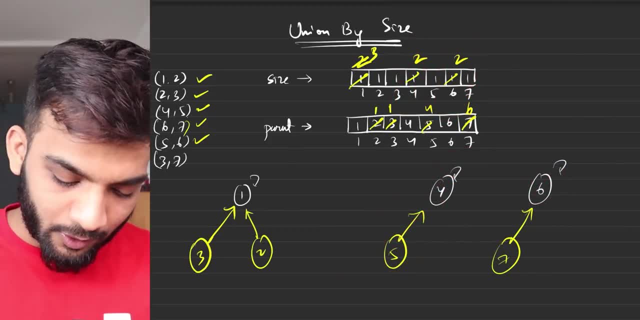 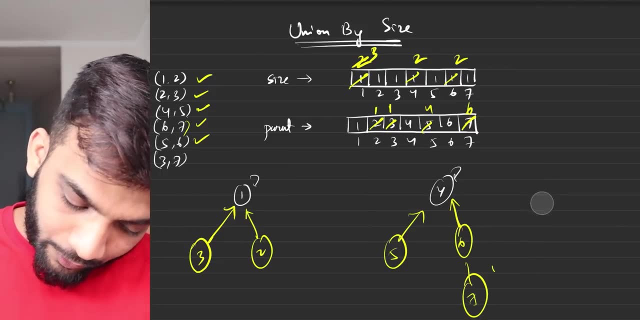 are of size 2, size 2, same size. so what you'll do is probably you can take 6 and get attached to this done. the 6th parent will be 4, 6th parent will be 4 and since you're attaching a size 2 to 4, 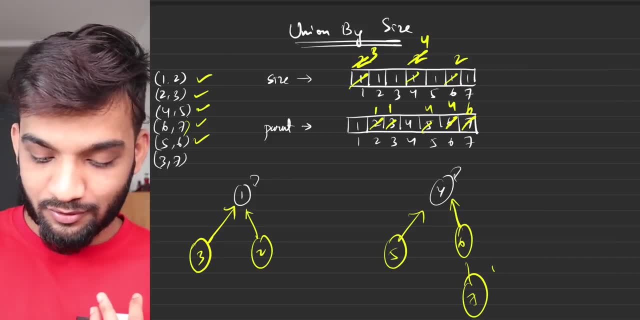 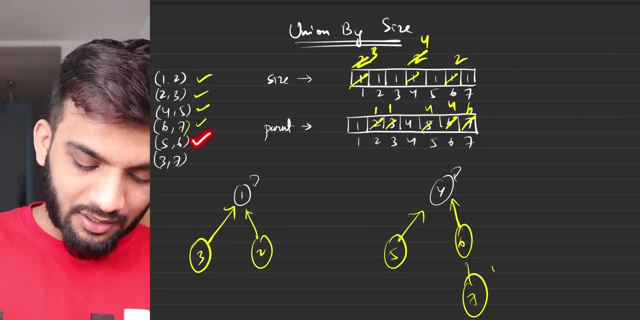 the size will increase by 2, not by 1. so basically, this is keeping a track of how big is this. this is keeping a track of how big is this. this is also done. next will be 3 comma 7. so for 3 it's 1. 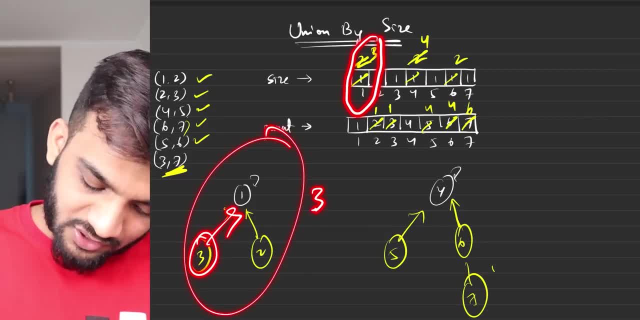 which is a size of 3: 3 size. component for 7. if you see, 7 has this, which is a size of 3: 3 size. component for 7. if you see, 7 has this, which is a size of 3, 3 size. 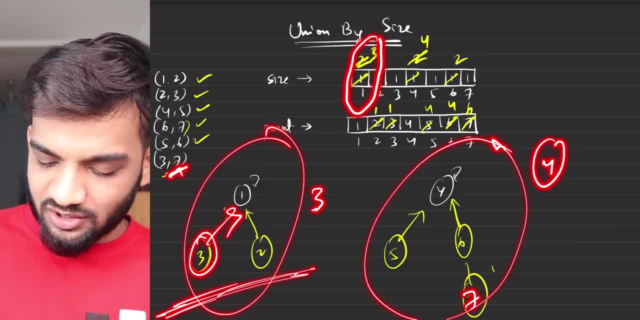 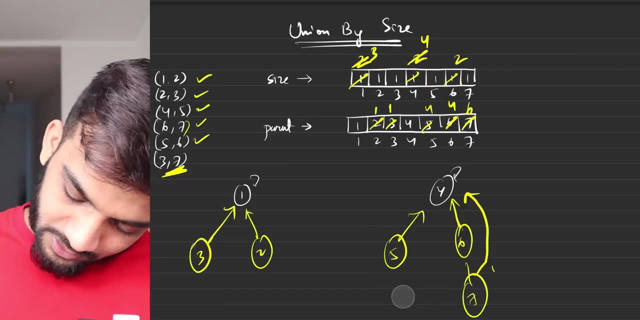 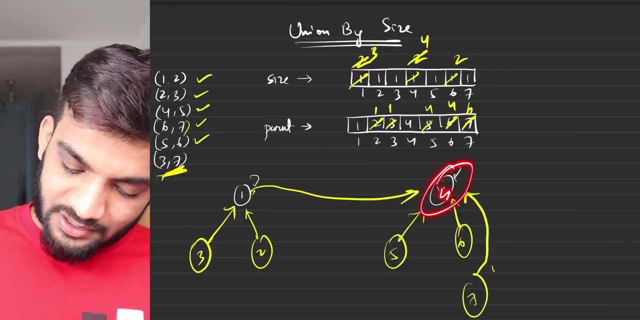 is nothing but a 4 size component. this is a smaller one, so this will go and attach. so when you try to find the ultimate parent of seven, definitely path compression will happen. here's the first step. next for three: the parent is one, so this goes and attach force size will. 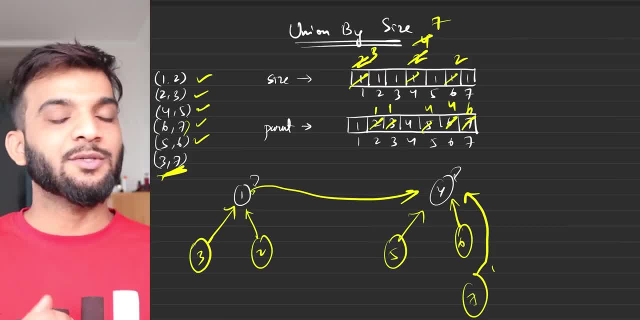 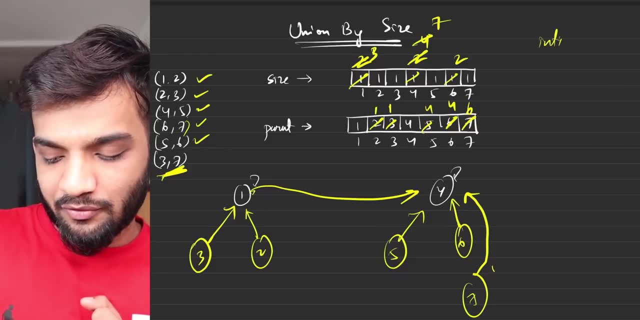 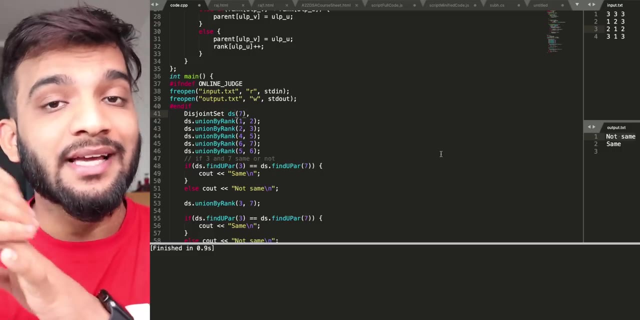 be increased by three. the four will be having a size of seven, so you can keep a track of size. and this actually is much more, uh, like intuition. intuitive, you can say: instead of the rank, i'd the rank. i don't find the rank to be that much intuitive, but i feel i find this union by size to 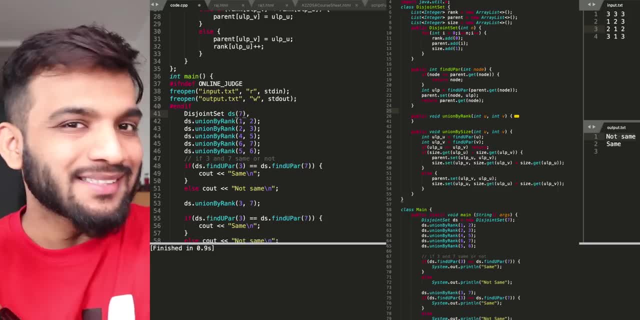 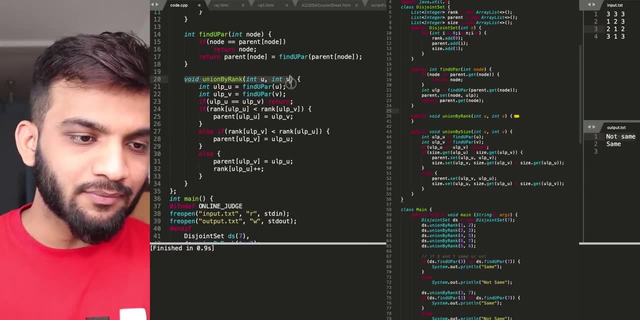 be much more intuitive than union by rank, because it kind of makes sense when you are storing the size because rank is distorted. so what i'll do is i'll try to copy the same thing. so i'll try to copy the same thing and i'll create in the same function. i'll just create union by size. 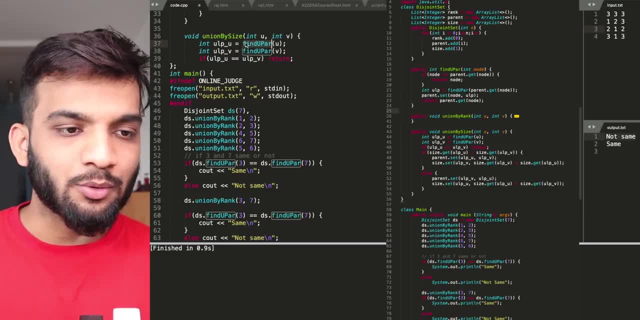 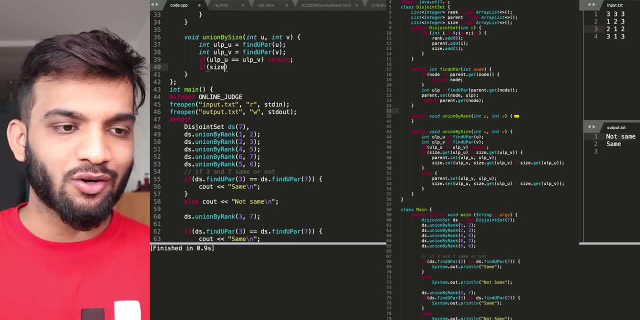 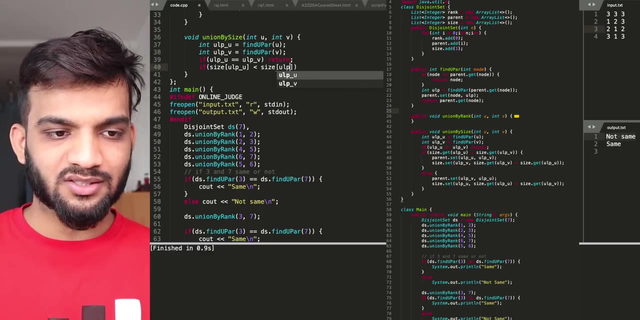 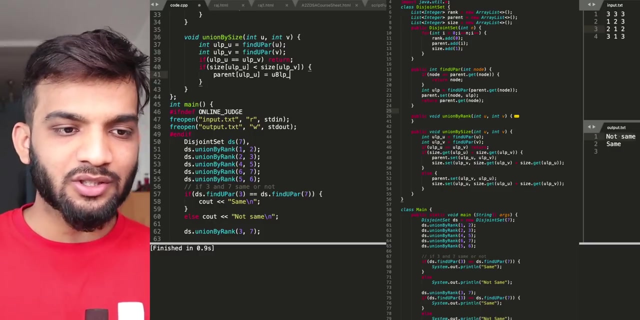 because everything else will stay same, union by size. and now what i'll do is i will say, okay, fine, i know one thing for sure: now i'm doing a comparison on the size. so size of this, if lesser than size of this, then i will like: okay, i will take the ulpu and attach to the ultimate. 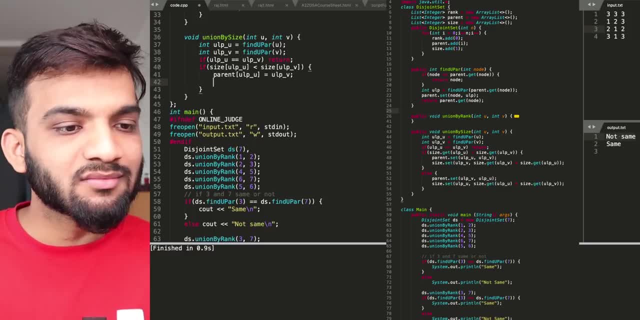 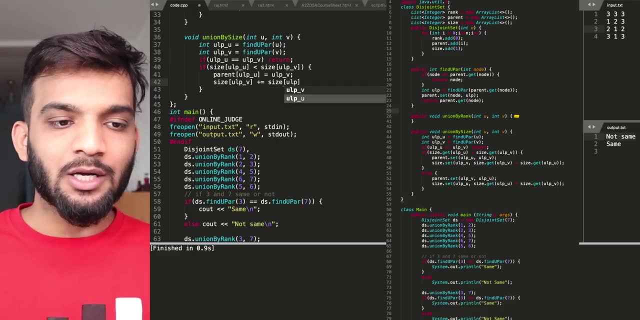 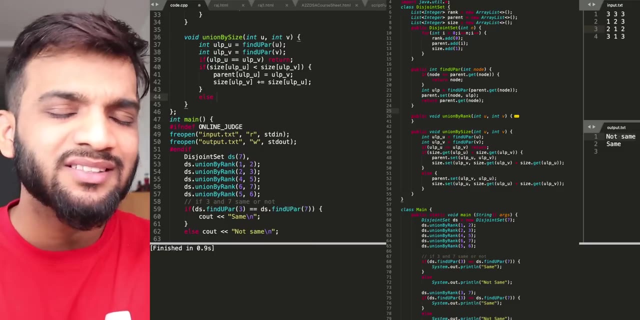 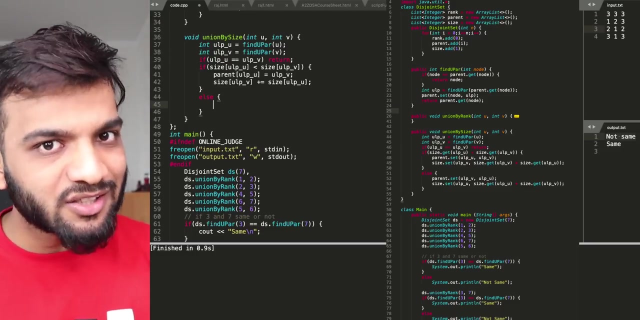 parent of v done next, the size of the ultimate parent of v, because it is getting attached to, will be increased by Matrix 1 pré取 you else. now will there be an equal case? if there is an equal case, you still attach it right, so we can just write an else instead of writing else, if greater and then else, because in equal it doesn't. 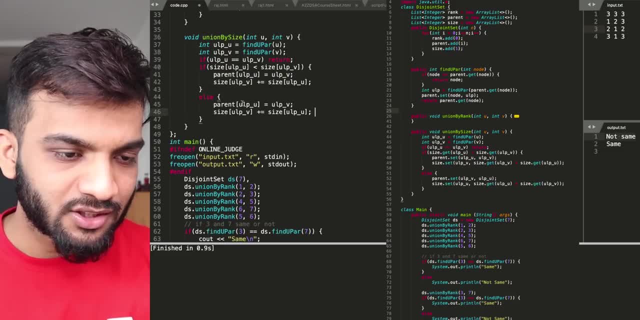 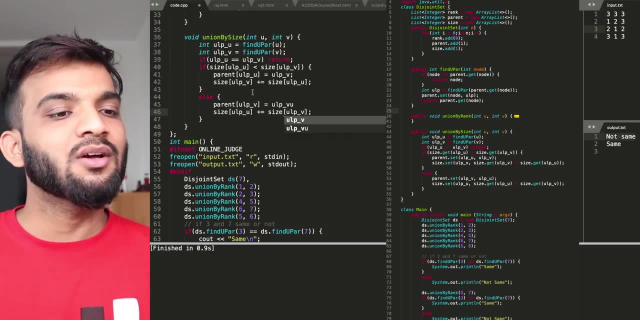 matter whom you attach to right. so i'll just take this and i'll just change this to v, i'll change this to u, i'll change this to u and i'll change this to v. that's it. so this is how the union by size will work, and what i'll do is now remember if you're implementing a data structure either. 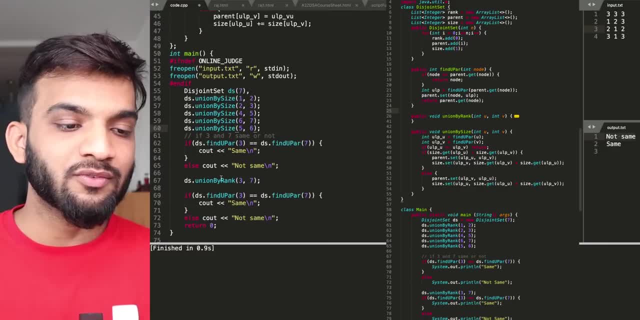 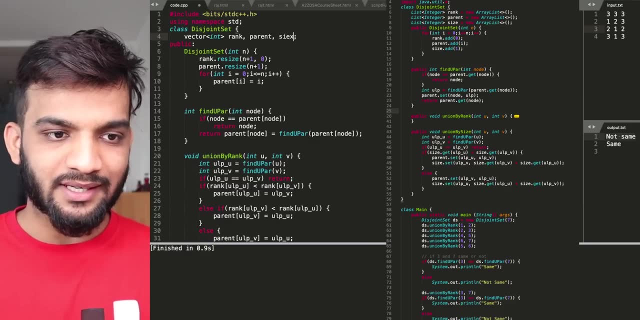 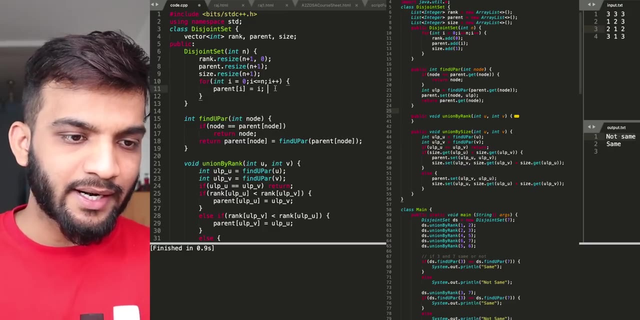 use by rank, or either use by size. don't use both of them together. don't use both of them together because we have to declare a size this time. so let's quickly declare a size, and over here what i can say is: size dot, resize n plus one, and i can go ahead and say: size of i is initially one. 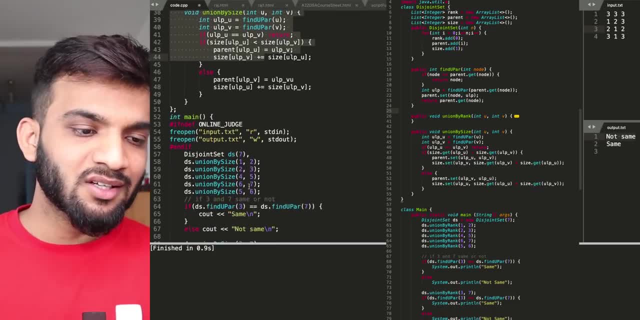 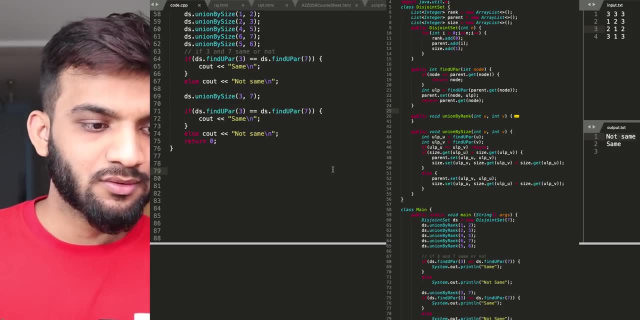 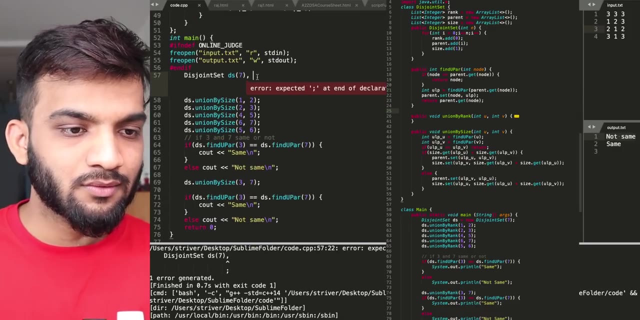 that's the initial configuration. then i've written the union by size, then i have everything is union by size. let's quickly do a compile and see if it is working fine. okay, looks like a mistake. oh, my bad comma here. okay, cool, should be fine. okay, not same, not same, strange. 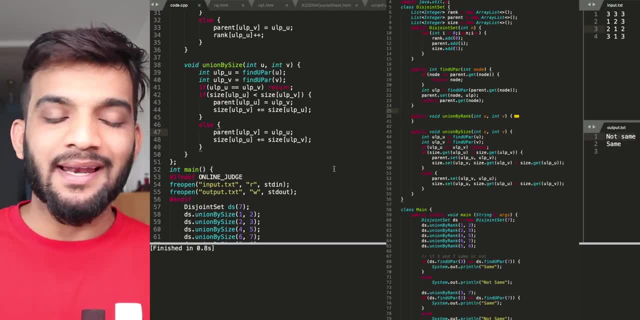 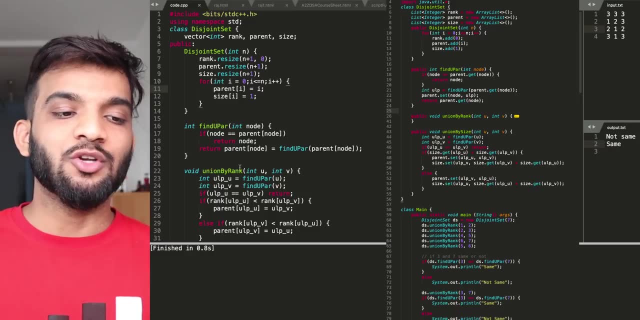 so over here there was a v. you have to make it u. okay, now we can compile and see if it is running. fine, yes, not same and same. so this is how you can easily create a snippet of code which has union by rank as well as union by size. what is the time complexity? which one is better? both are of the.